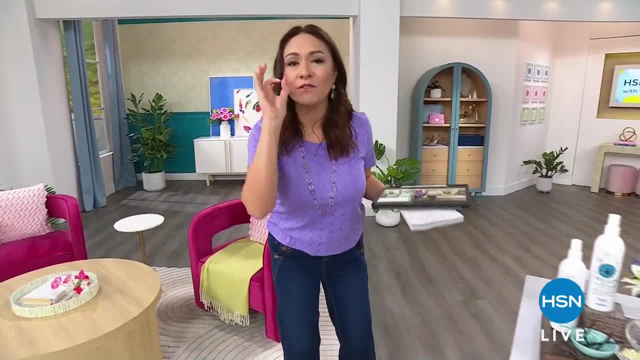 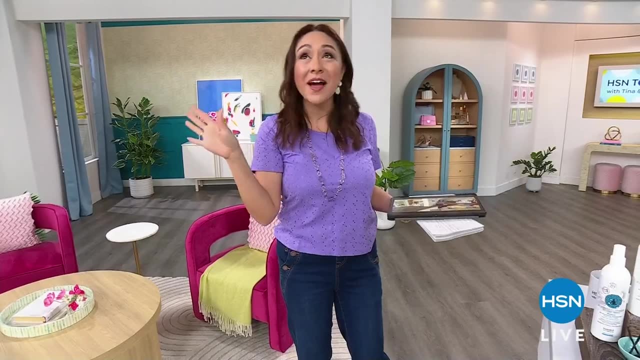 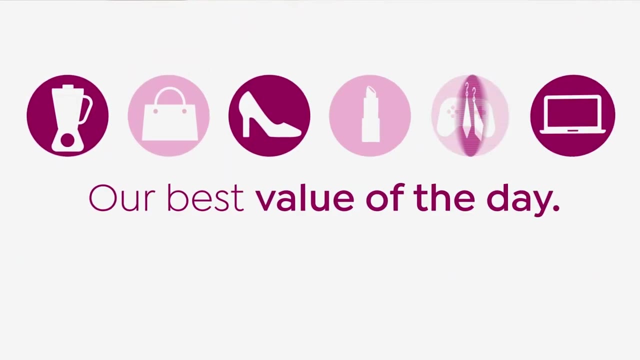 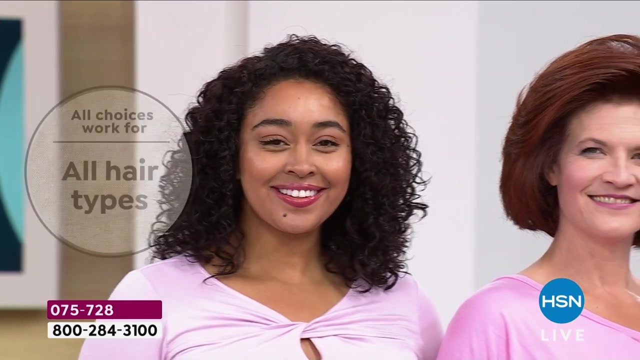 We always show you the Today special. Today's is on fire. You want to know why? Because everybody is able to use this on their hair And it's a brand new item that you've never seen from Tweaked by Nature If you have curly hair, short hair, fine hair, textured hair. 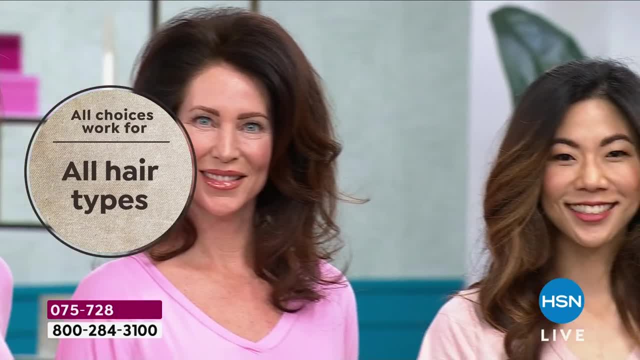 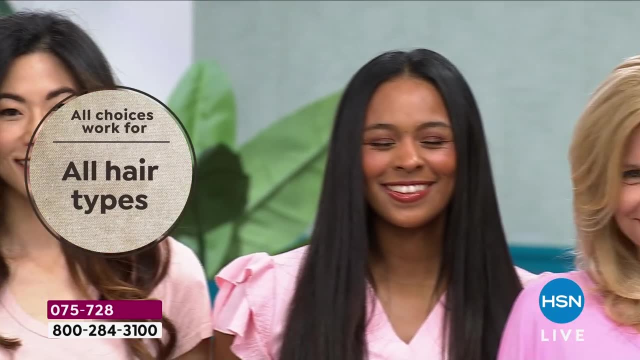 damaged hair, frizzy hair, brittle hair. I feel like I'm no hair. Dennis Simeone is like: this is how you become world famous. For 25 years, Dennis Simeone and Tweaked by Nature, brought us this amazing Restore Vitalizing Mist. 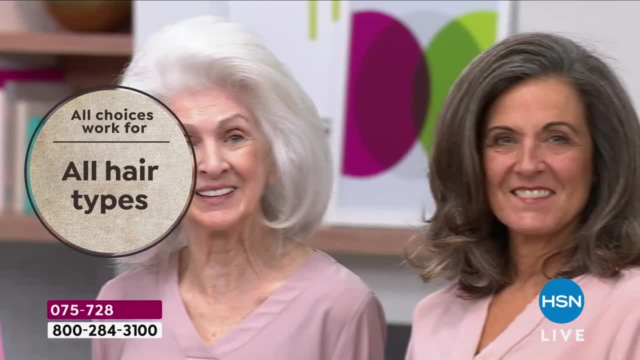 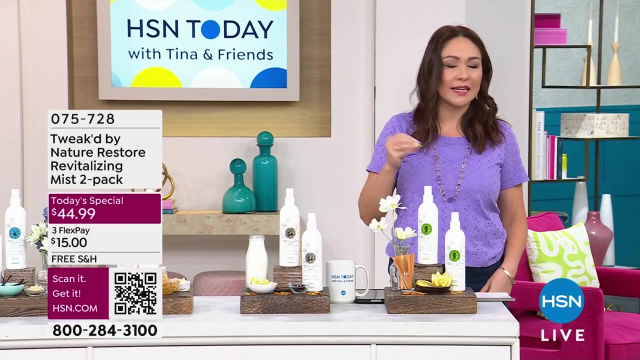 Well, you know what? I couldn't keep calling him the ingredient hunter if you don't keep hunting me ingredients. So it is the spray that protects us, repairs, gives us shine, gives us body, But now in this 20.. Now, 26th year, I guess. 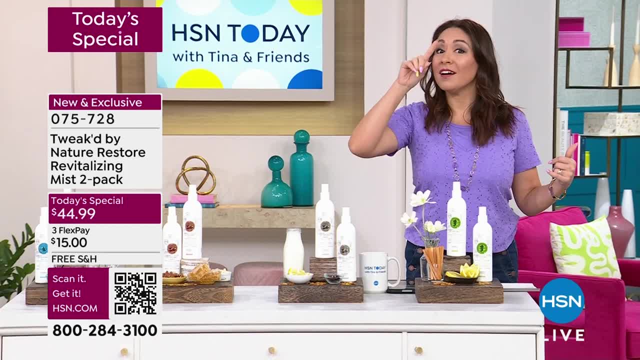 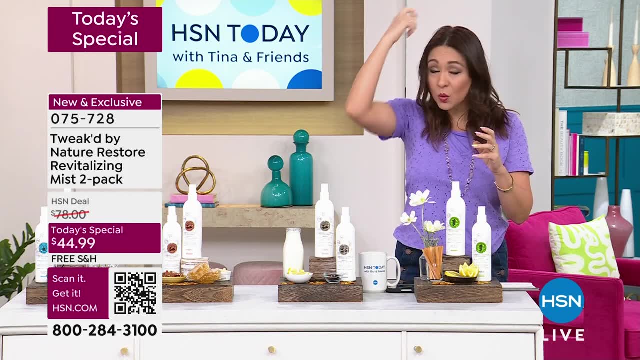 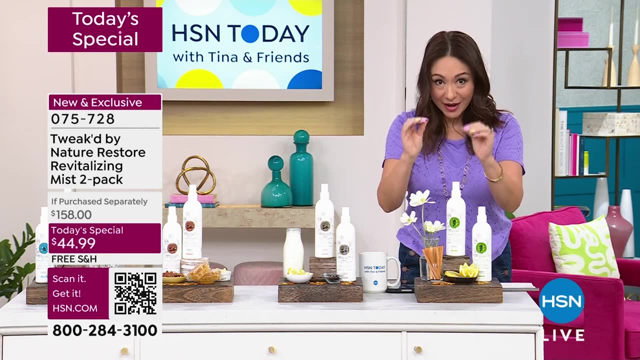 25.. This is the 25th year, 25.. We've hunted a new ingredient, So it is everything that we have loved. The numbers have not changed. One squirt of this, One squirt on your hair: We are, on average, reducing the breakage in your hair by 97.6%. 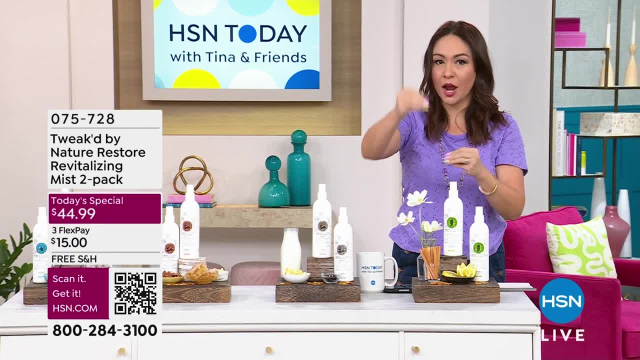 By one squirt on your hair, It's also going to protect your hair, Give it shine, Give it body, And it's- It's this beautiful, gorgeous scent. Now I want to show this to you. Hold on, Let me get my bearings here. 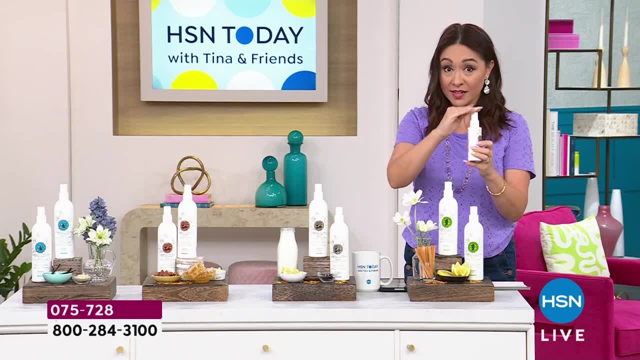 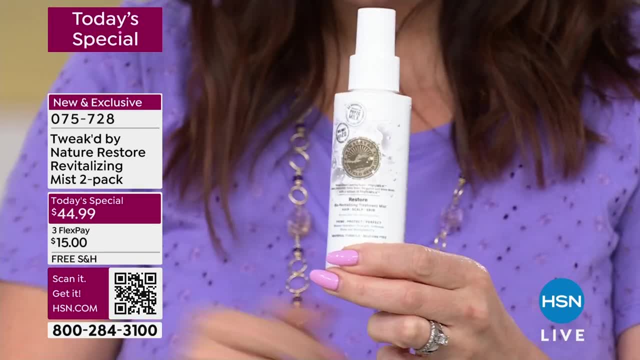 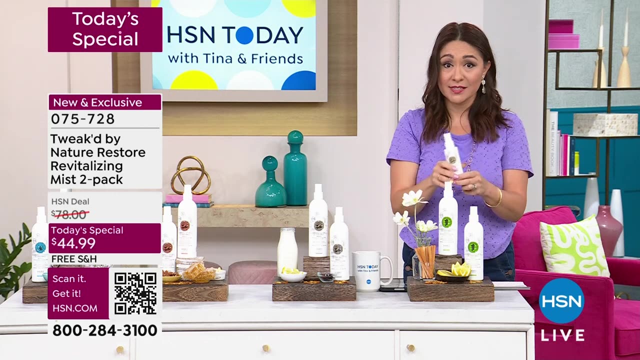 Normally. we have seen this in a four ounce. We've seen it, We've loved it. This is just the new, with the phyto milk in it, The new ingredient. okay, This is four ounces, It's $26.. So we have done this in a three times the size, which has gotten it to 12 ounces. 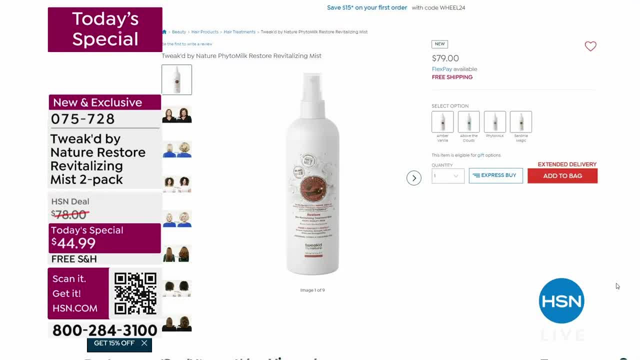 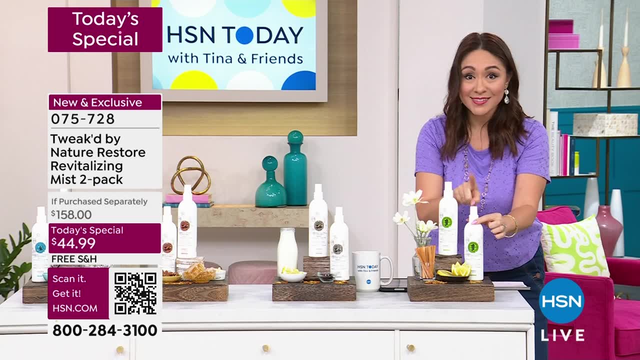 And it's been $79.. That's math, right? We're all doing some math. Don't order that one today. Don't go to Age of Scent, It's there. You can, Don't, Because what if I said that $79 bottle is going to be $44.99 today? 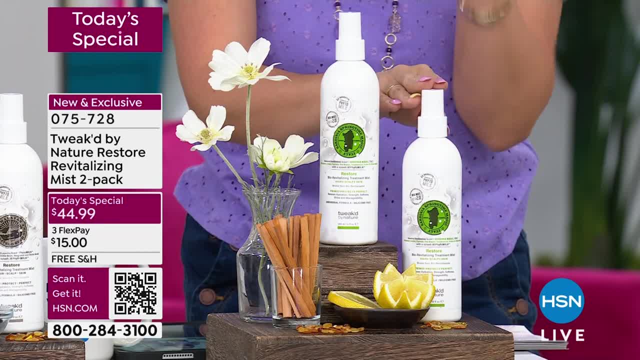 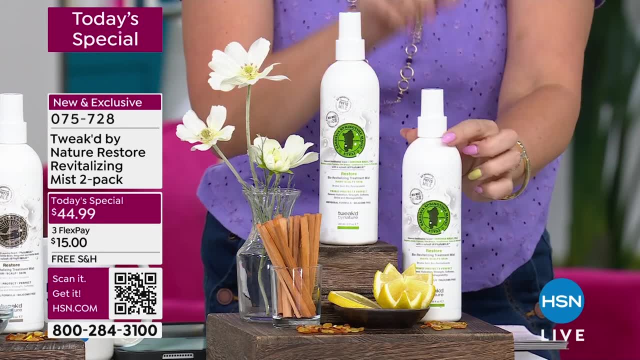 That $79 bottle is going to be $44.99.. That'd be $34 off. We could have stopped at one bottle. We could have made that a today special. It would be all hair types giving us everything that we love. The brand new ingredient included. 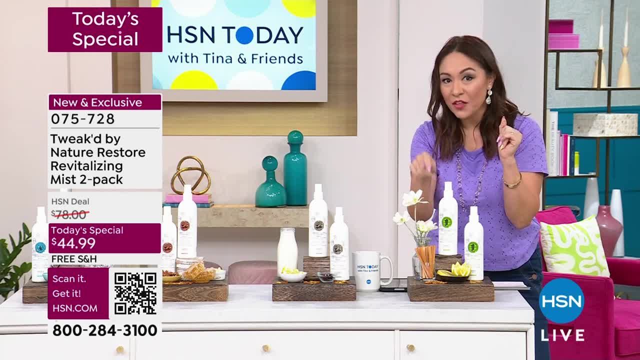 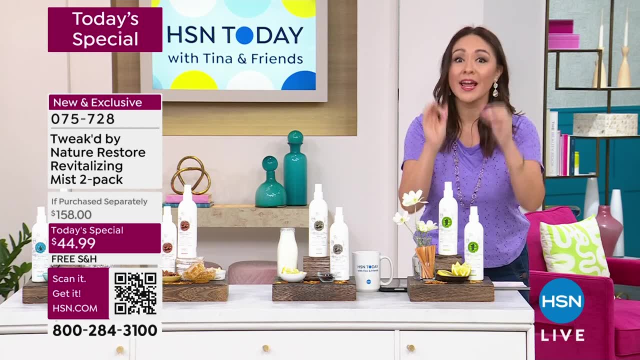 But Dennis was like: oh, we ain't launching like that. He's going to give us another $79 bottle at no additional cost. Yes, You can put this on auto ship. Yes, We will ship this to you for free. And he even said: let's give you a brand new scent. 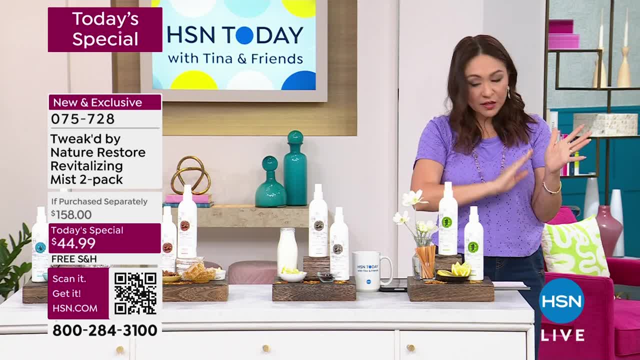 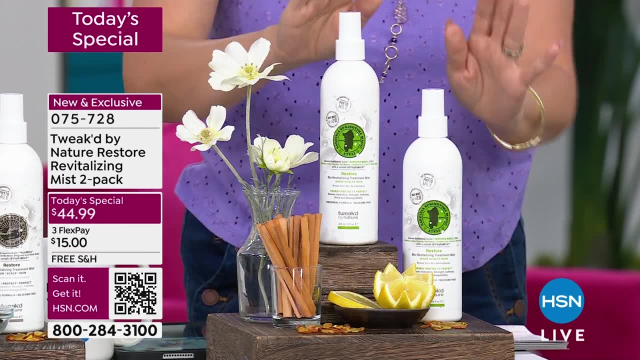 So let me go through your options that you're able to get this. The will be an early sellout. Everybody always goes for the new scent that Dennis brings us. This is the Sardinia Magic. So if you would love to get the brand new scent, make sure that it's lemon. 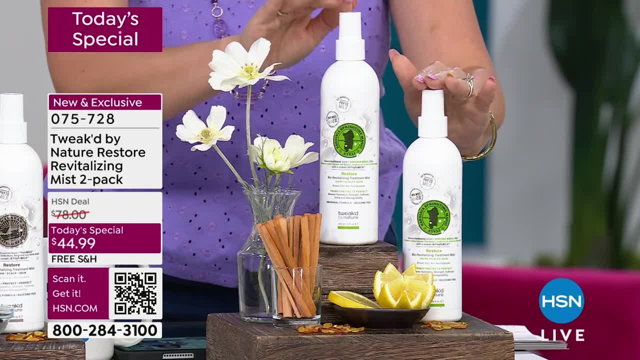 It's cypress, sea breeze, sandalwood, amber white musk and, of course, that phyto milk that we're talking about it, And he already knew you guys were going to ask for the phyto milk fragrance on its own. 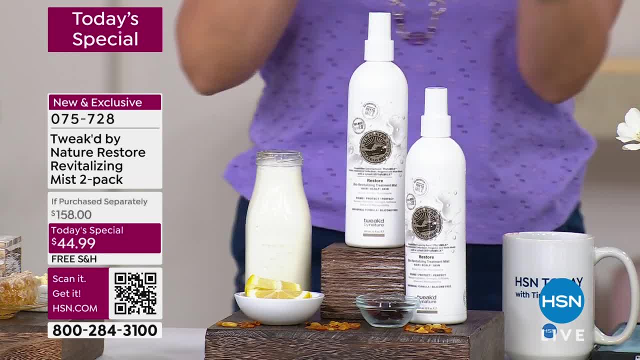 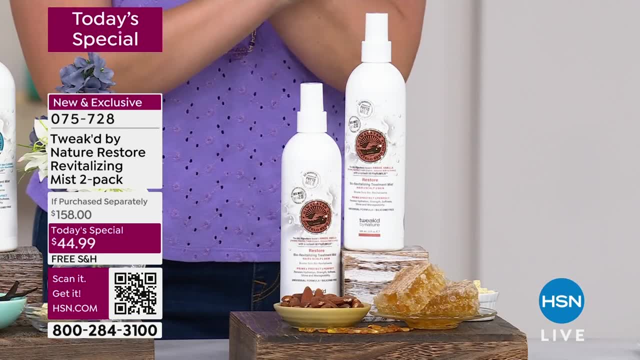 He's giving that to us as well. And again, this is again that tonka bean, a little bergamot white musk and that phyto milk. that's in there. Now my amber vanilla. you've loved it in, Tweaked by Nature. 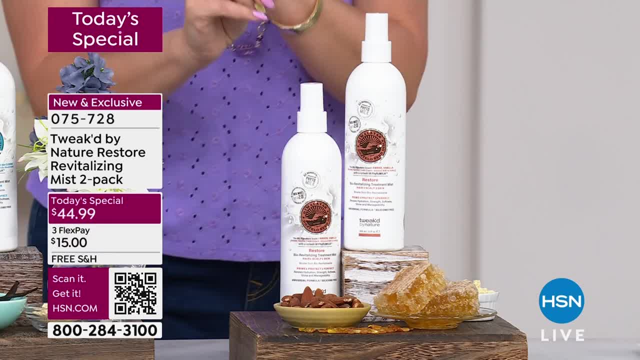 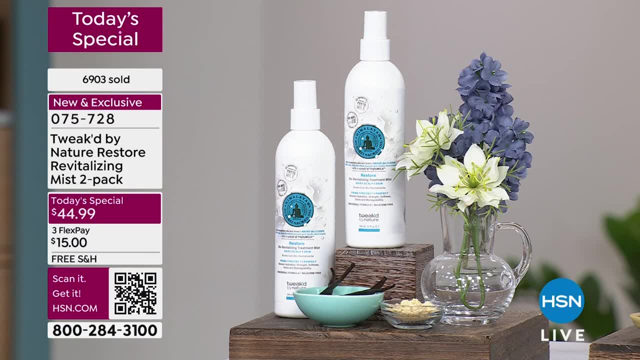 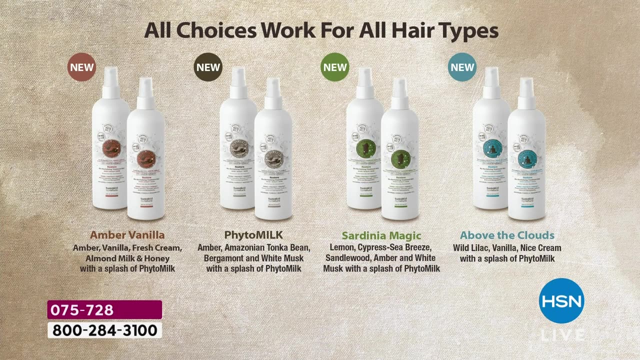 You have been an amber vanilla person. It's that just a little creamier, a little softer. beautiful amber vanilla, And again the world famous Above the Cloud: two pack Starting with Ojan Ingredient, hunted like in a canoe, Ouch. 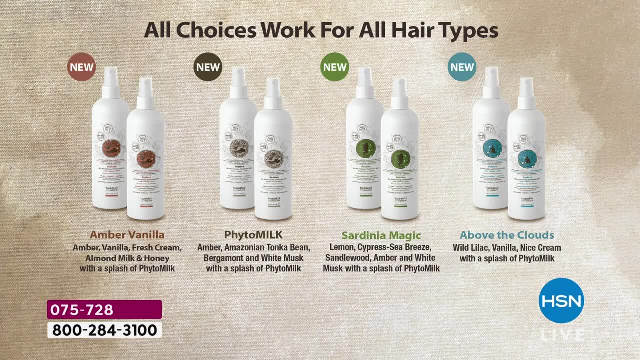 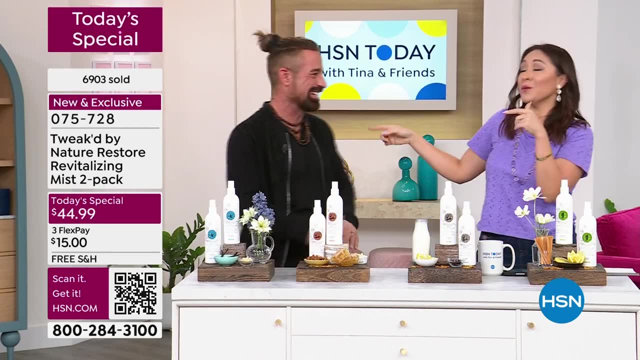 With all of the people Explains my sciatica. When you were talking about the good morning, Dennis, Dennis Simeone, can I tell you he Donuts to the luggage. Look when I tell you he's opened up his heart to the world. 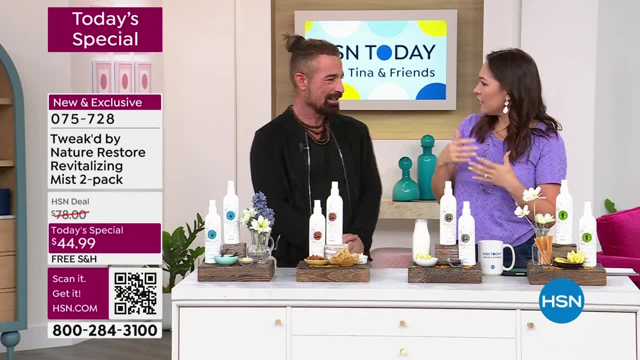 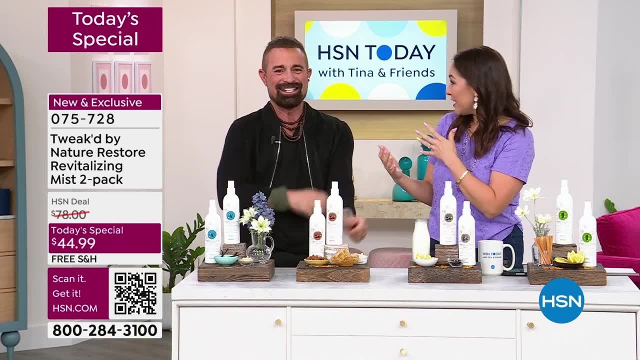 He talks about his mom. You've talked about your kids And you. I said I would take. I would take your ingredient hunter card away if you didn't keep hunting new ingredients. And you do, You reinvent Always, yeah. 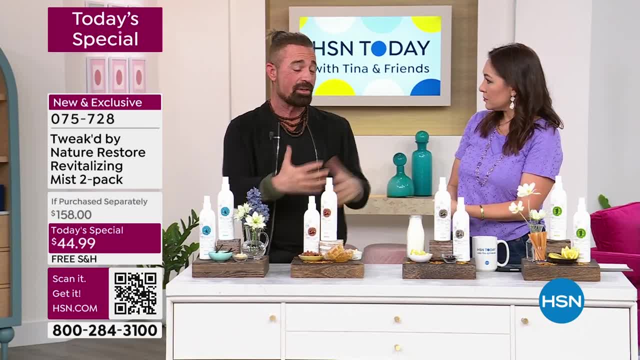 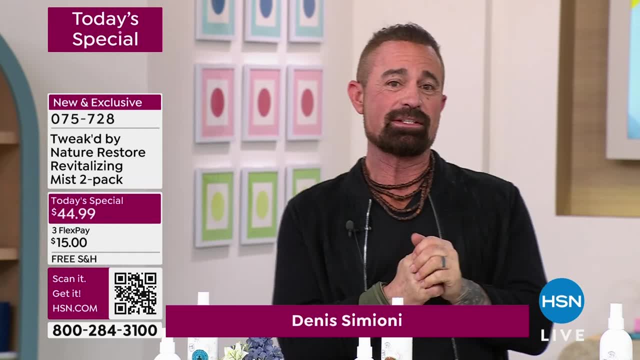 But also keep like the base of what you're about. Yeah, this one was cool Because it's 25 years, Yep Ago. well, July, that I discovered Ojan, me and the kids- Yes, I lied to them- said we're going to Disneyland. 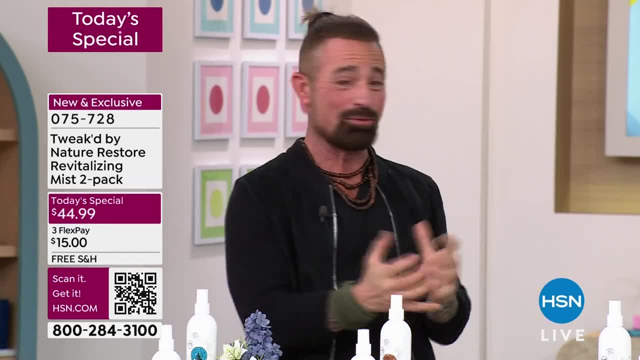 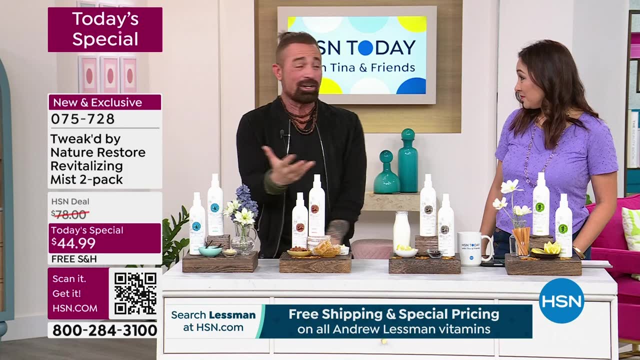 We were supposed to. It's a little little white lie. It was the real jungle cruise, The real one, Real alligators, crocodiles, spiders- Yeah, it was good, But we found Ojan, Yep, Yeah. 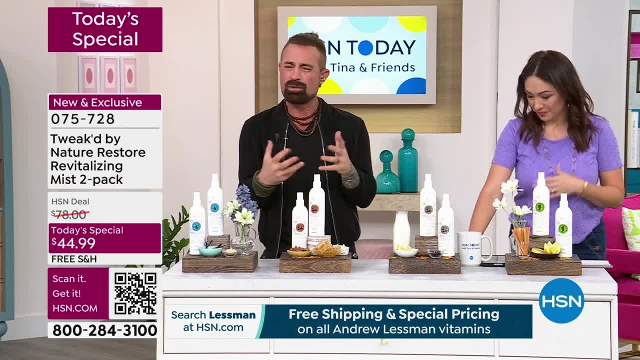 So with that, 25 years later, there was an orange peel that I've always wanted to use with Ojan, but it's orange And it was one time I put it on my skin and I looked like an orange. So 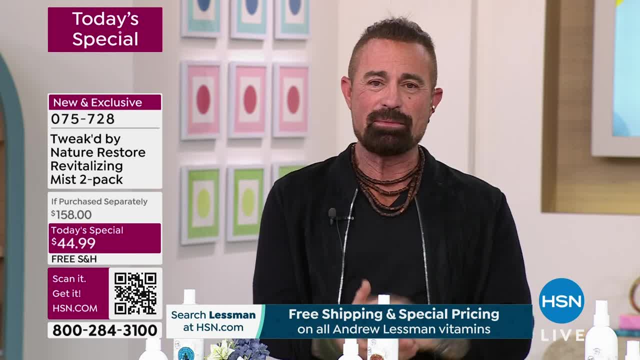 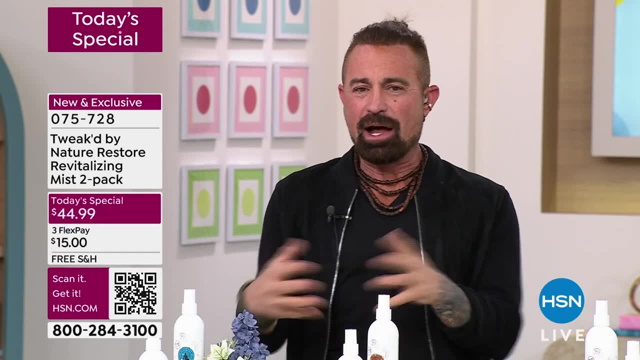 So I needed to find something with it. 25 years later, a lab in Brazil was was able to create a nano version of it. And but this is a clean nano. no, no metals, no iron. It was done with water and it turned it into a milk. 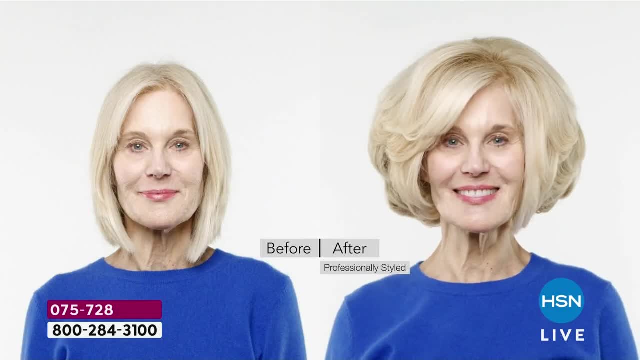 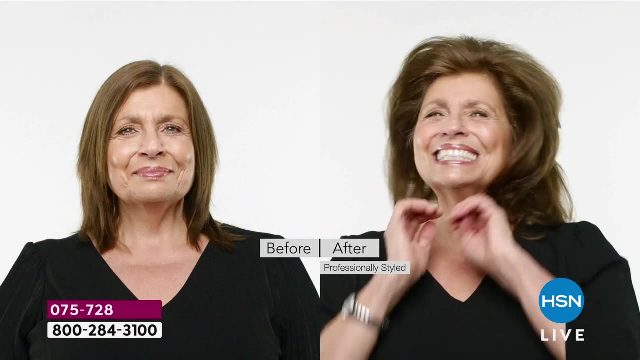 And- and I just had a smile on my face because I knew I had something special- Four almost 400 times smaller Yep In size- That means we can penetrate- Started playing with it and I basically turned it into this phyto milk. 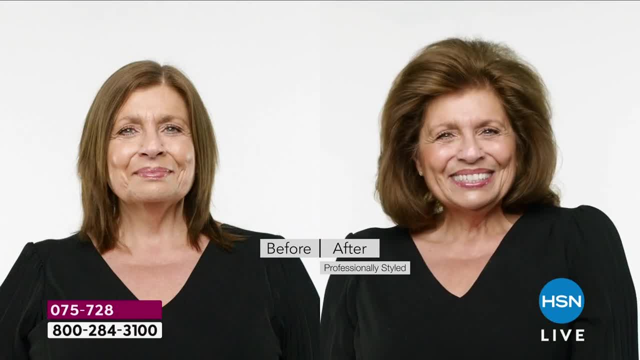 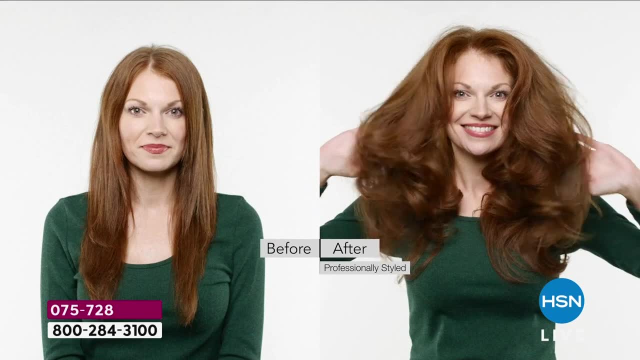 I threw it into the mist because I knew that's where I started. I wanted to see: Can I make that better, Way better? Right, It's way better. And what we had was amazing: A 97.6% reduction in breakage one time. 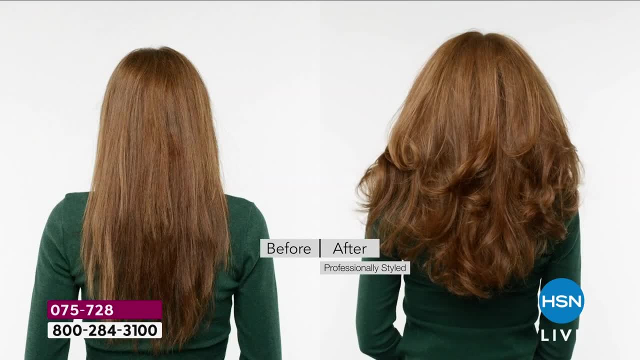 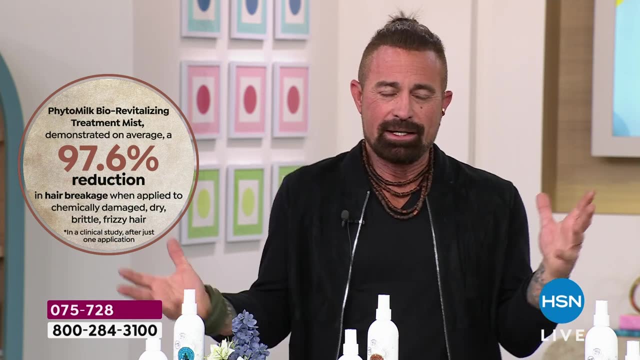 One time You've got six months worth And, like what you were using before, you can cut that dose down in half. That's how much more potent this is, So that's why the size is slightly smaller, but it's it's fine. 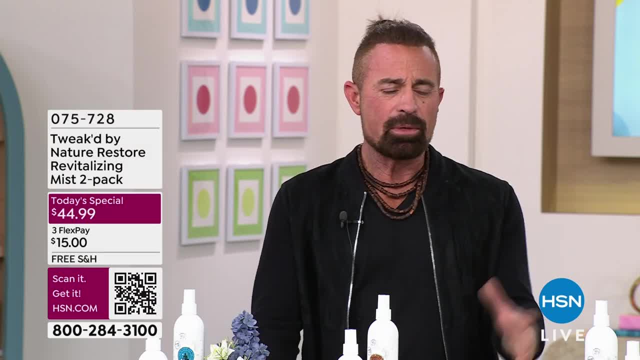 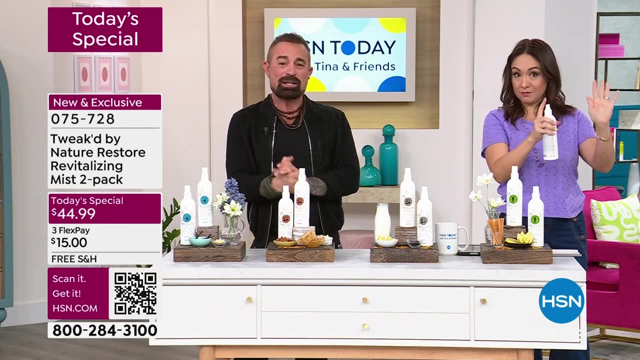 The mist is micro, so it's super, super, super fine, But you only need two or three spritzes, Whereas before five or six. No silicones. it's as clean, green and mean as it could possibly be. 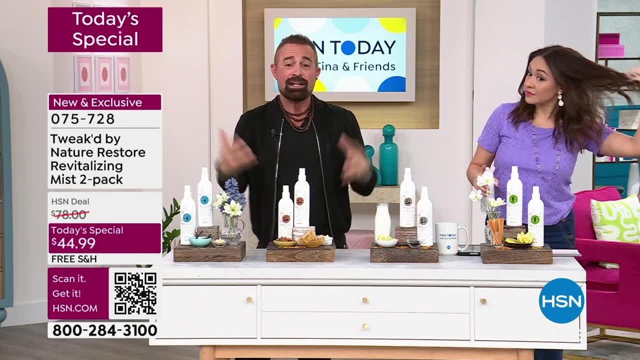 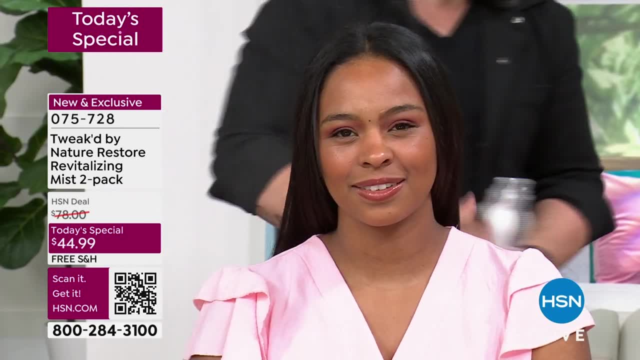 And it's for all hair types. Even if you don't have hair, it's phenomenal for skin. Wait, let me explain why Dennis is saying no hair. When I used this the first time, I spritzed it and I kind of did this with my hands and my hair. 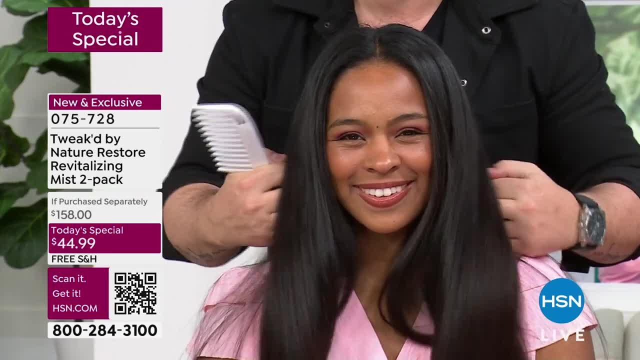 Late. like an hour later I was like, why are my hands so soft? It was because I touched my hair with it. in there It creates this nano film, but I call it a veil- that goes onto the hair, onto the skin. 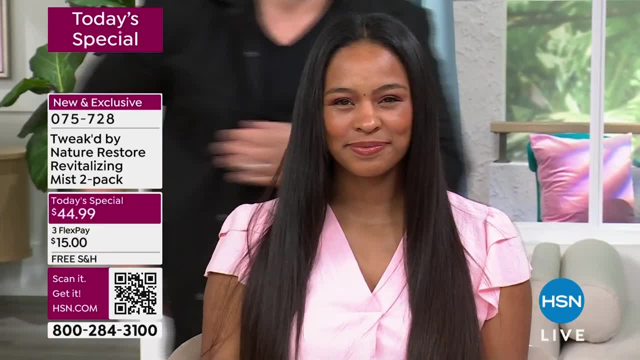 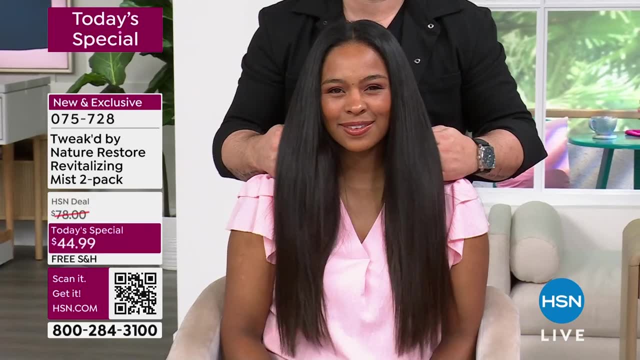 Yeah, Yeah, Yeah Yeah. It's a veil that goes onto the skin. It just holds everything a little bit longer but at the same time allows it to breathe. It's flexible, But when it's in the bottle, all my props were in my luggage. 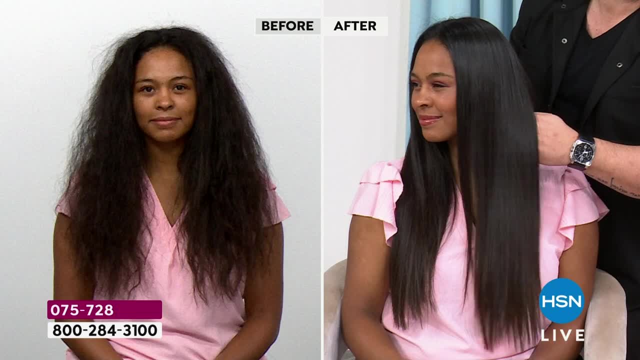 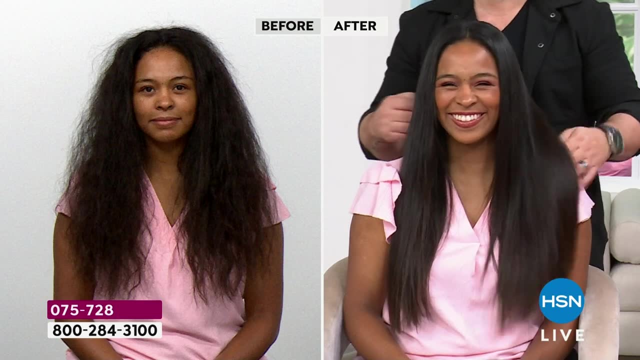 So I was going to show you that inside the bottle it's really creamy like a thick cream And then, but it jets out as like a nanoparticle, So it's really fine And the mist helps that. You can see I was doing the or or or or. 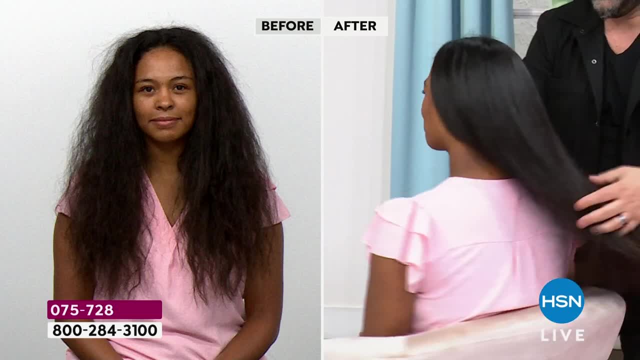 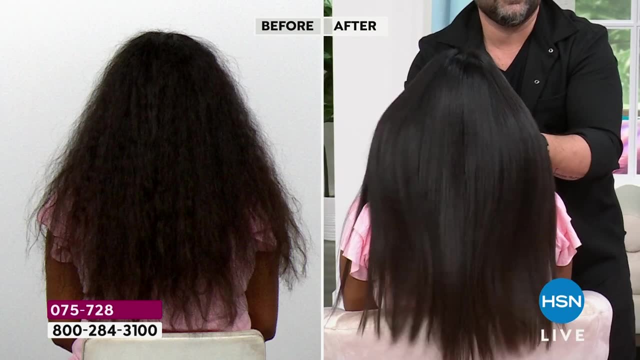 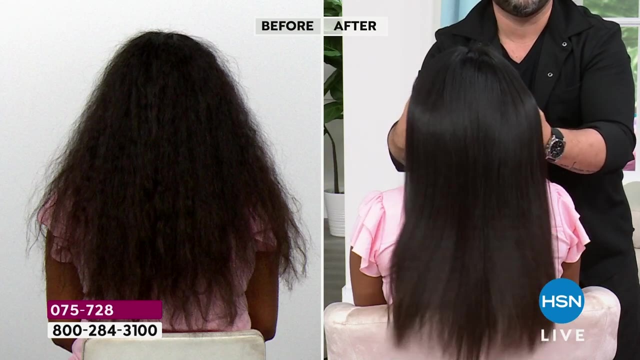 I had trouble just now- Oh my God, It's too early, But the shine that you get. remember no silicone. So this is what happens. Look at that Like your hair is becoming stronger, healthier. Donya, Don't got to wait 30 days, basically not even 30 seconds. 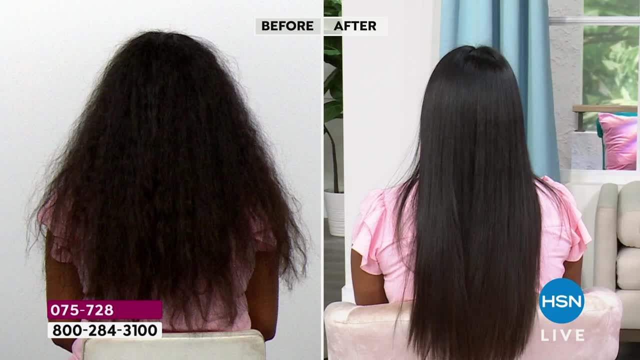 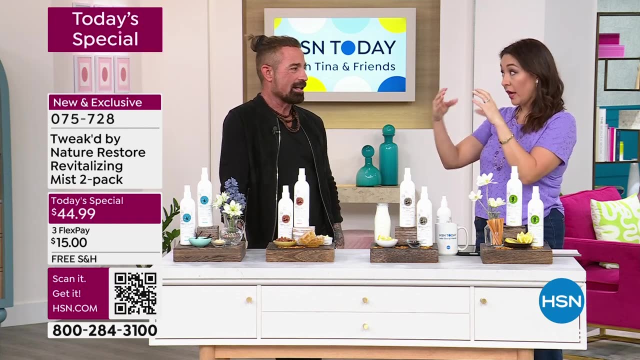 It's, it's a seven second splash mask. Okay, Think about this. If you're like 97.6, that's it seems like a very weird specific number, This is because it's clinical. Like you, you're like: I want to know exactly how much we're going to repair the damage to your hair. 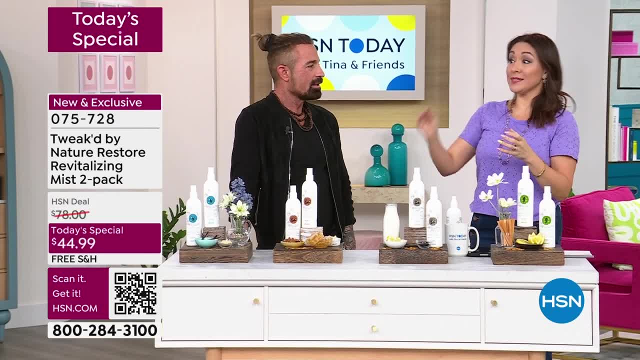 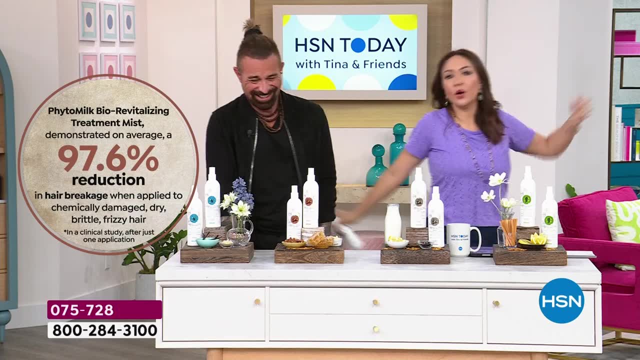 If it wasn't better, I wouldn't have touched it Right. That's why we got the 0.6.. I mean, this is down and think about this. this, I'm 97%. I mean, think about that. What. what do we get that kind of? but it's not only that. I used mine this morning, got out of the shower towel, dried my hair, spritzed it on. 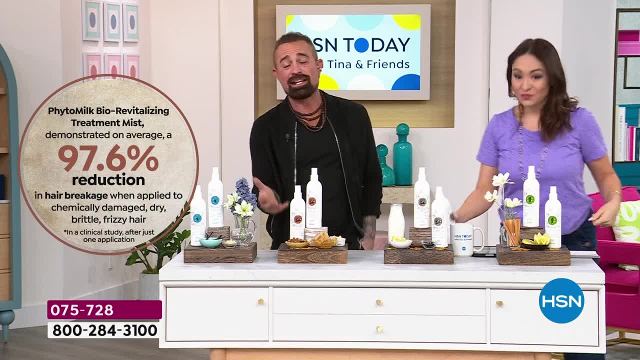 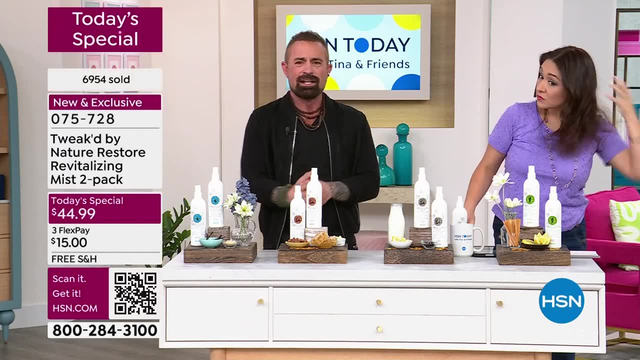 And then I did my blow dryer Cause you moved it's motion And actually the fragrance it activates when you when there's movement. So that way if you're like stagnant, just sit sitting, still, you know if it's, if a scent is overpowering you'll, you'll want to wash it off with this. 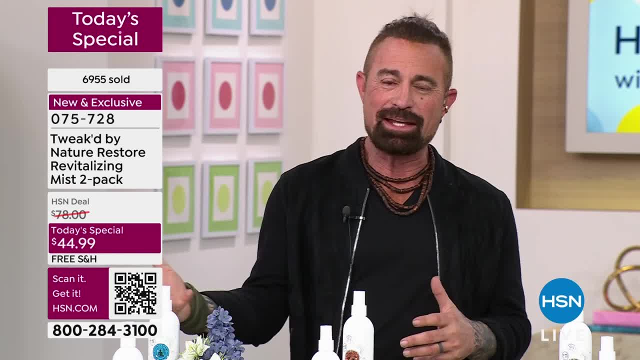 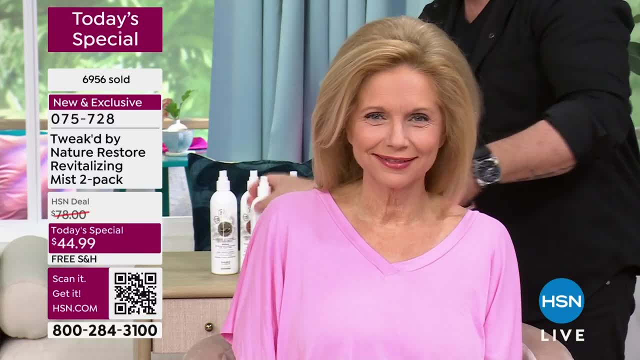 Okay, It's up to you. It's: the more you move, the more scent you're going to get. The molecules begin to burst and you lay- you lay a trail, a beautiful one, I think, why you cannot do this wrong. 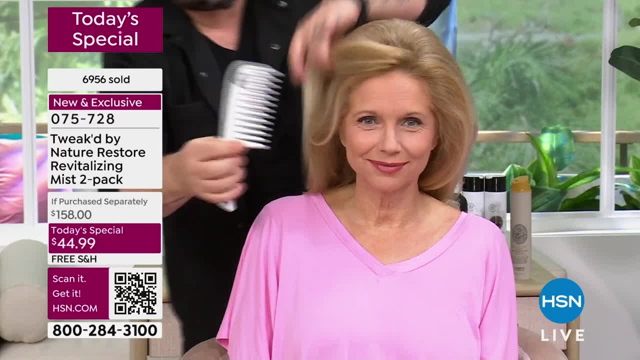 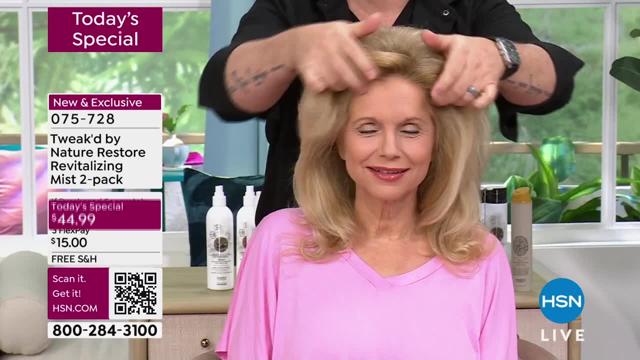 Wet hair, dry hair, damp hair, middle of the day before you go to sleep. you literally cannot do this wrong. There's certain times that are better. So when you wake up in the morning, put this before you do anything to your hair: don't put water. 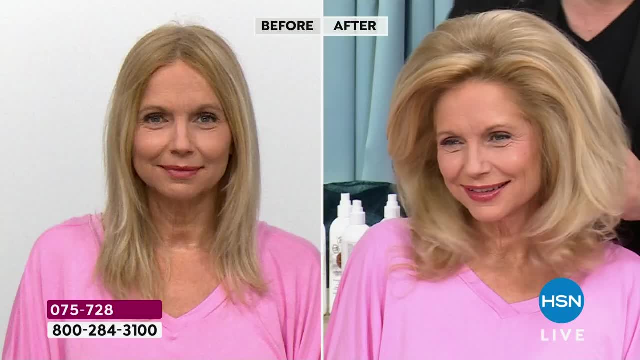 Water is more damaging than anything. So this will be how you, if you have a kink in your hair, You want to get rid of it, You spray this in. I was amazed at her hair. Look at this. So she's been with us about a year. 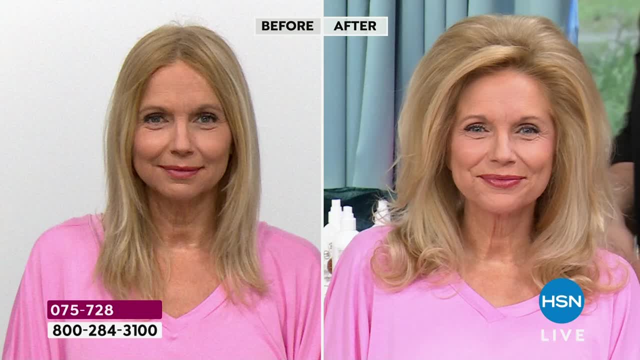 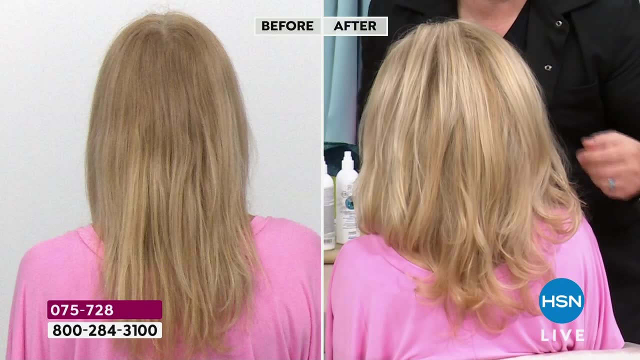 Um, my God, her hair is super fine too. So to see her with a transition- And I mean, like you, look at the before shot that we took yesterday, um to today, the next day, uh, the highlights, everything is improved. 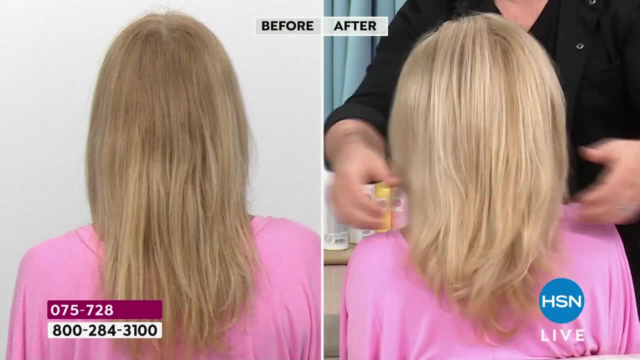 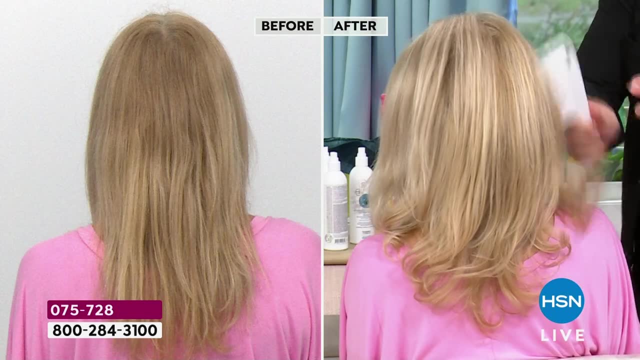 As I said, you get an instant improvement. You don't need to wait. This is more than just a leave-in conditioner, This is a powerhouse. Okay, Okay, This treatment that in 25 years, for me, I've never seen anything like it. 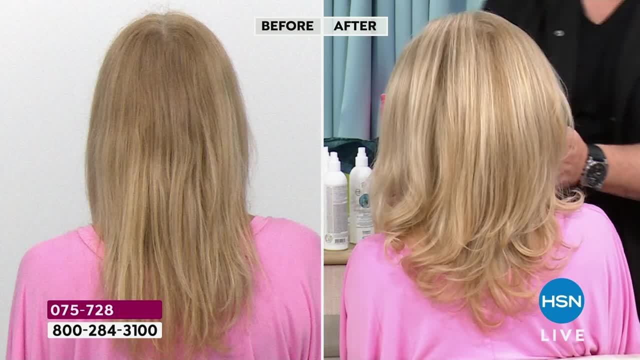 And you get to, it doesn't matter what scent you go with, but the Sardinia Magic Can we talk about, because nobody's smelled it yet. So I feel like we have. we have to explain it, because if you're like, oh have I had this one? You haven't. No, I was on a vacation, and just the aroma that you get in the morning sunshine, Um, there's also this, this dew that's in the air. It's, it's, it's, it's mixing in with the Cypress, the lemons, uh, the limes. 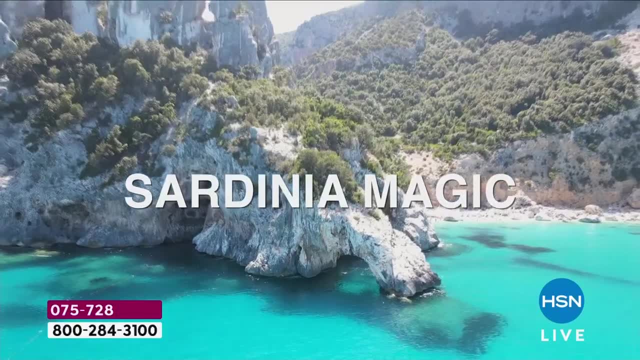 And basically it's kind of- and I was eating, maybe it's because I had Fruit Loops. I knew you said Fruit Loops last night. I always think of Fruit Loops. Yeah, I was like: did I hear that right? 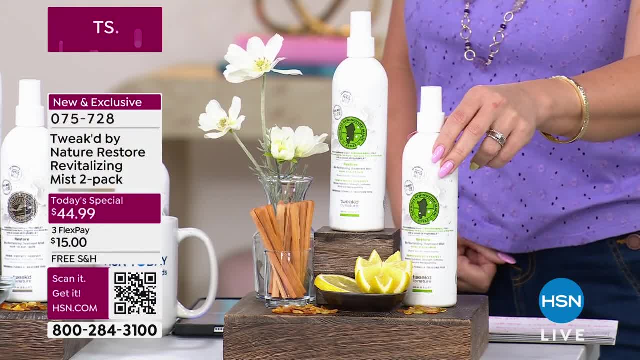 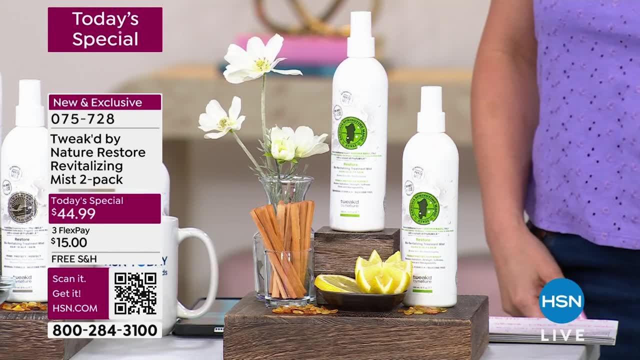 So now that I said Fruit Loops, when you get it home, you'll, you'll smell that like there's just a 10% and it's just the combination of everything. So I look, I'm, I'm weird. What can I say? 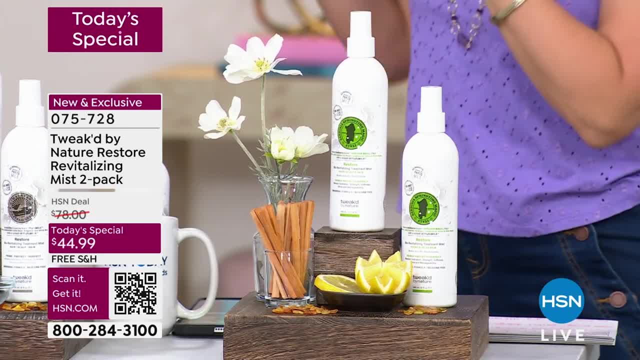 And I'll tell you I love Fruit Loops. When they asked me, when I got an early sample before anybody could get it, and they were like: which scent did you want? I'm just like you. I was like I want the new one. 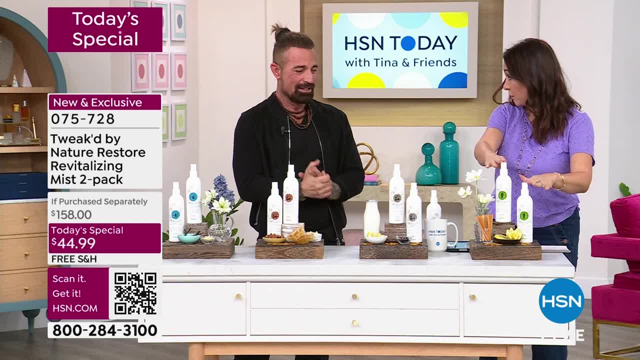 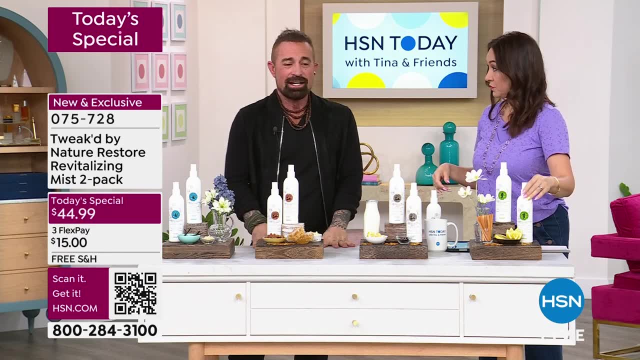 I want the new one that I've never tried and that's why this one is the most popular People that already love this for the 25 years you've been getting it. It's your only chance. Yeah, Because when we create a fragrance- me, um I- I literally get it from the source. 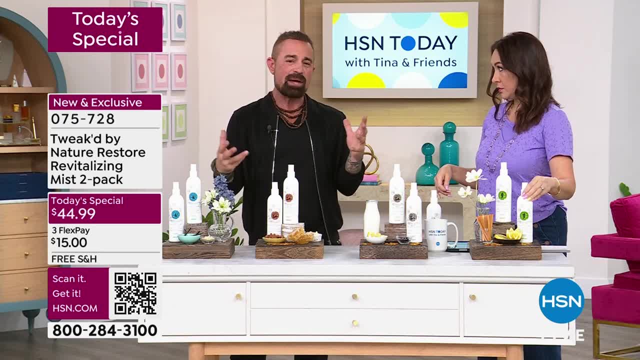 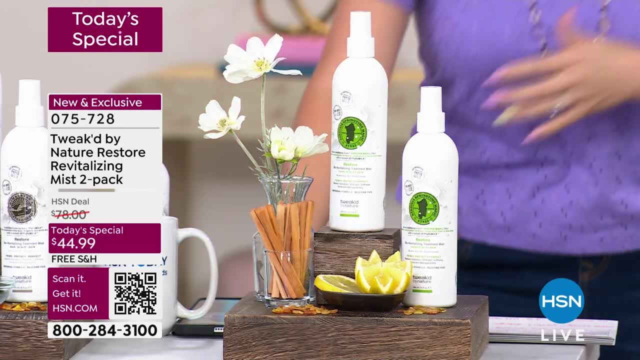 So same lemons, limes, and I dehydrate everything, turn it to a powder, Um, and then I mix from there so that you are literally smelling what I'm, what I smell, and Amanda smelled that day. Well, I want, by the way, before we go to the next, scent, if you're, if you're looking. 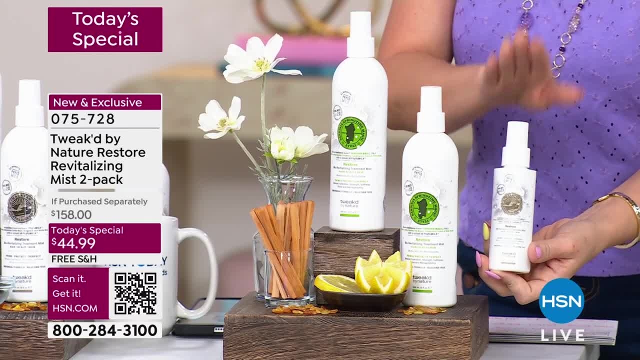 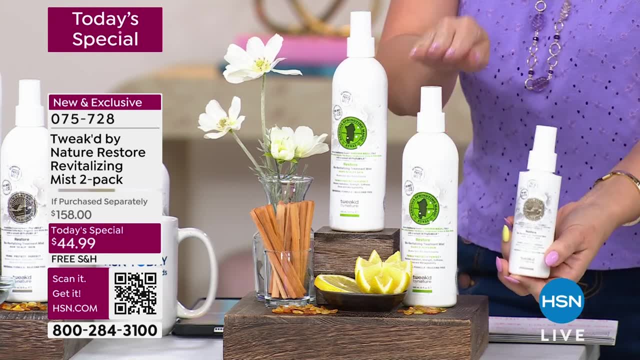 at this. We've done this in in a in a four ounce and it's $36 at four ounces. This is a 12 ounce bottle. So this is this is three $26 bottles that are in here, So right now it's $79.. 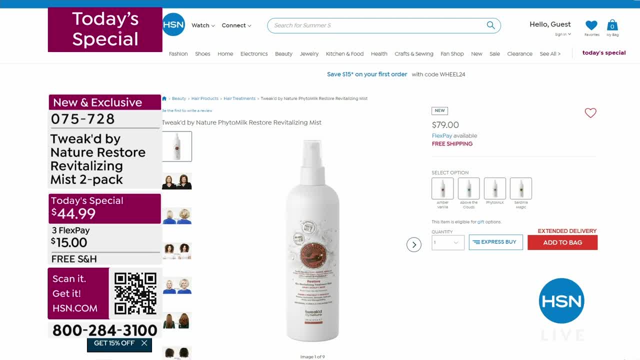 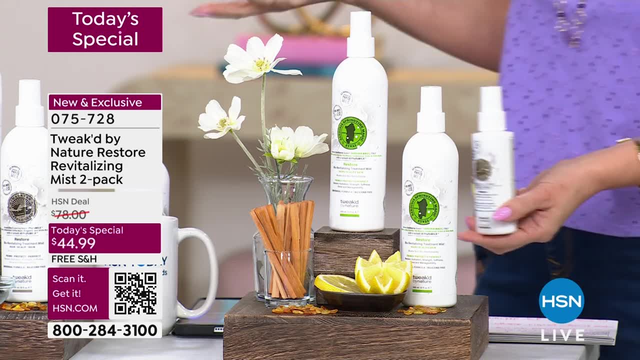 The cents are there for one 12 ounce bottle. We could have literally done the one bottle- that's $79- for 44: 99, and that would have been a today's special. That's an incredible deal. Yeah, absolutely No way. 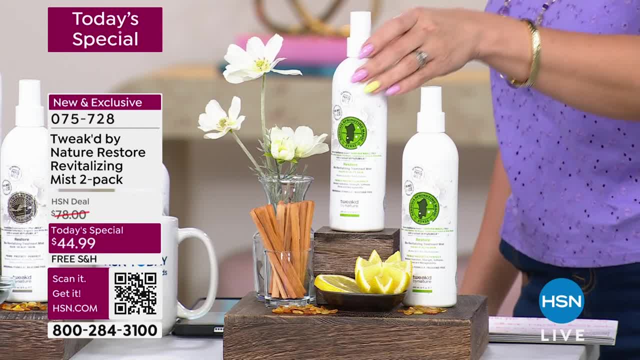 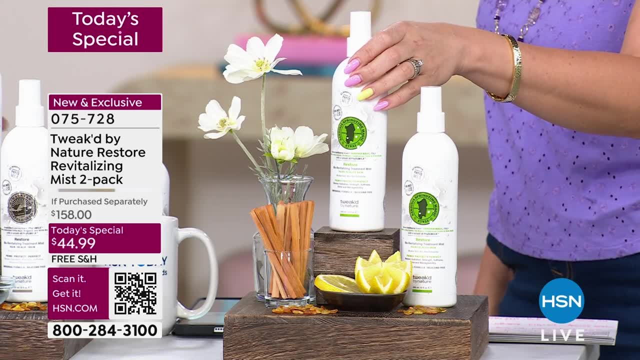 Dennis, are you giving us another 12?? Not my 25 year. There's no additional cost. You gave us the free shipping. You'll even let us lock this in on auto ship. No way, Yeah Well, because that Sardinia milk and even the uh above the clouds with the splash. 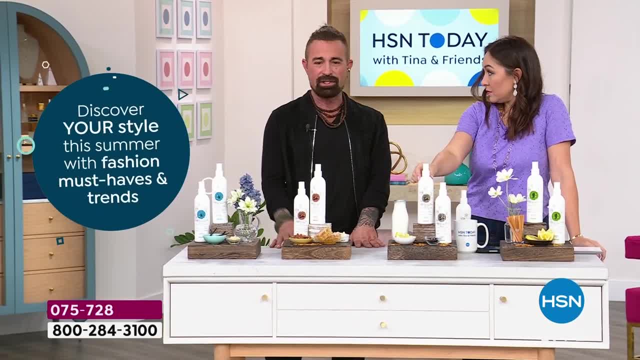 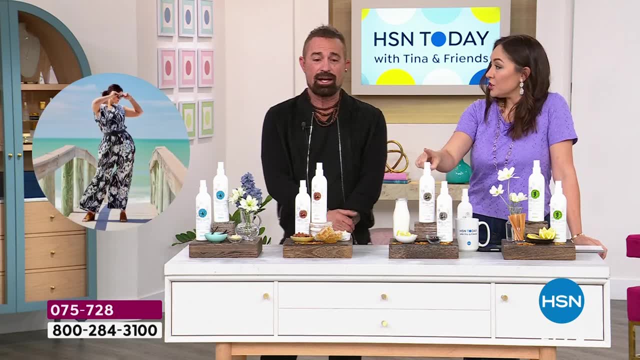 of milk. it's only in this, that's it. So if you get the auto delivery, then you're the only ones on the planet that'll have access to it. Yeah, It's just too difficult for me to keep maintaining put in stock. 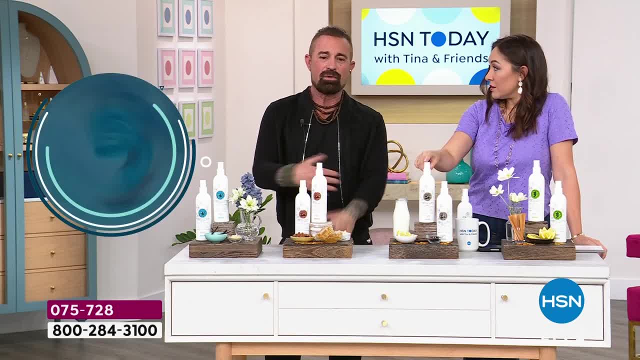 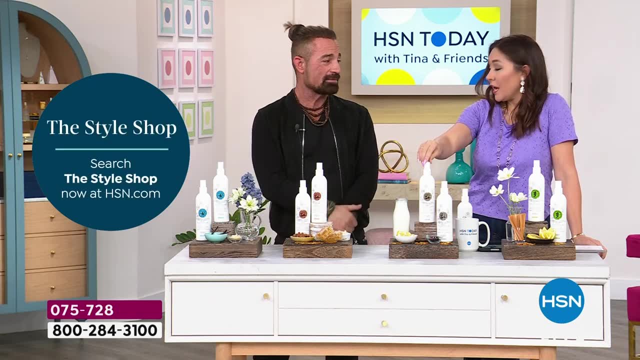 I look what we're. we're limited by nature and the more things that I do- cause I have 60, 70 ingredients in these- the more that I launch, everything becomes a little tighter. So that's why- And last night I heard you say you got ahead of everybody asking- you did the Fido milk. 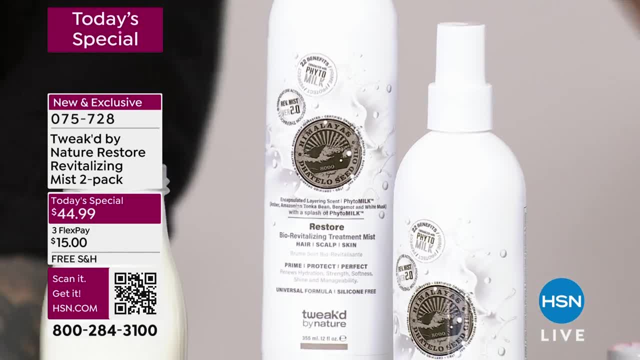 You were like I knew you were going to ask. let me just put it out there. It took 25 years, but I know how you guys work now. So cause you're going to smell the Amber vanilla and say I love the new Amber vanilla, but 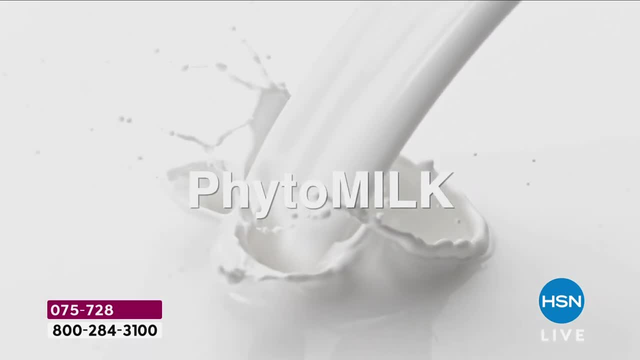 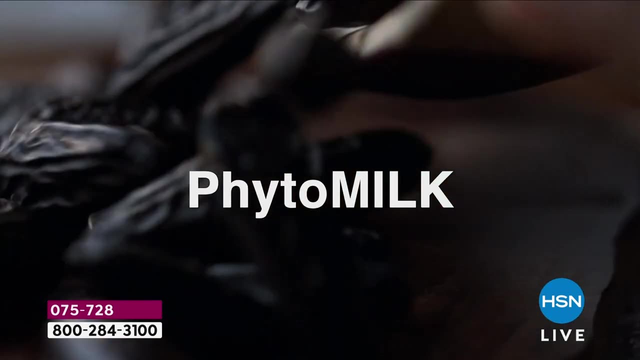 what it is. it's just the. it's the Fido milk that's been splashed into it, And that Fido milk it's the Ozone peel and that blended in, but it does have a tonka bean, Yeah. 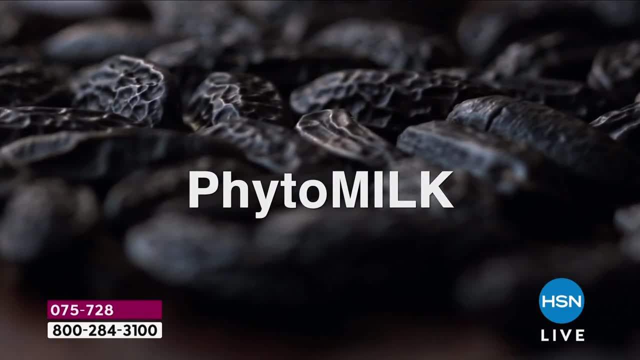 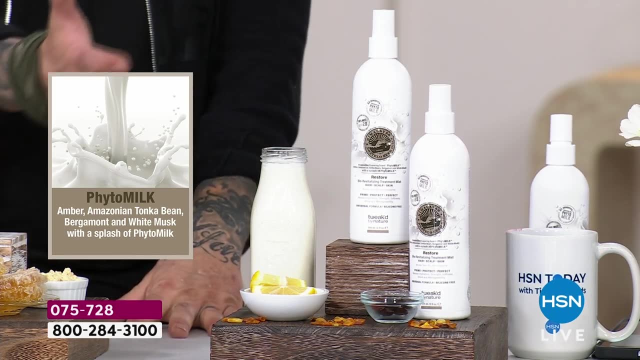 Yeah, I call it fruit loops in a way, but at the, at the end, mixed in with the milk, the best part. So I basically I'm giving you the Fido milk on its own and it's, and that's, the base of. 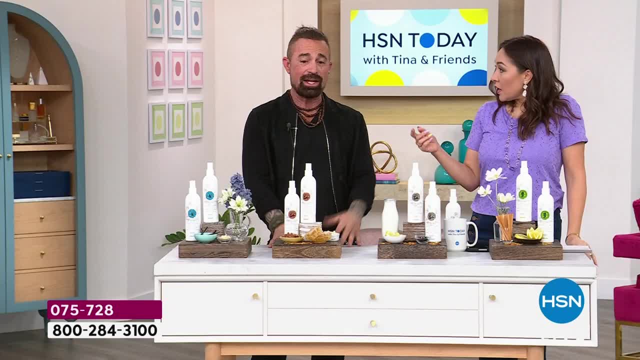 basically all of them, And it's phenomenal. It's, it's beautiful And it layers, So it's a layering scent. This, if this. if you're wearing just a Tom Ford fragrance, this will blend with it. 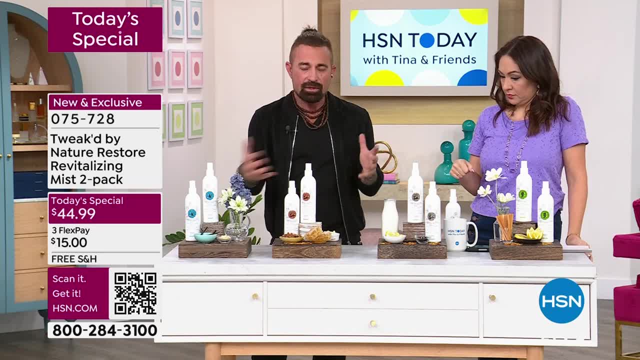 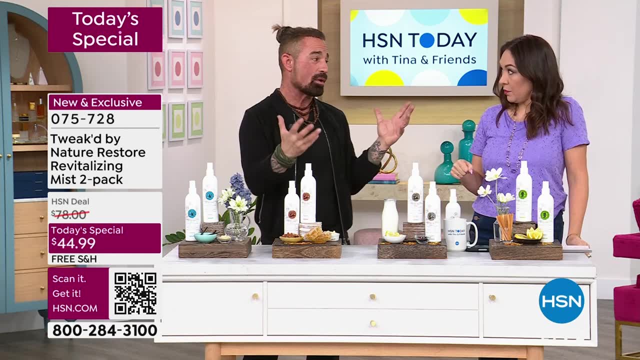 Kind of go, Yeah Yeah, Seamlessly So, and because it's also motion detect or motion censored, the way that it's going to burst as you move, it blends. It's because you're moving, so it blends perfectly. 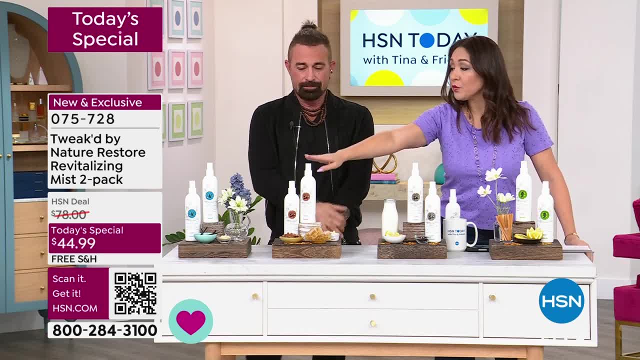 It's really, really clever. So Sardinia magic, the Fido milk, the Amber vanilla and the above the clouds, above the clouds, just went into the lead and not really like this morning. all of a sudden, everybody wanted that one. 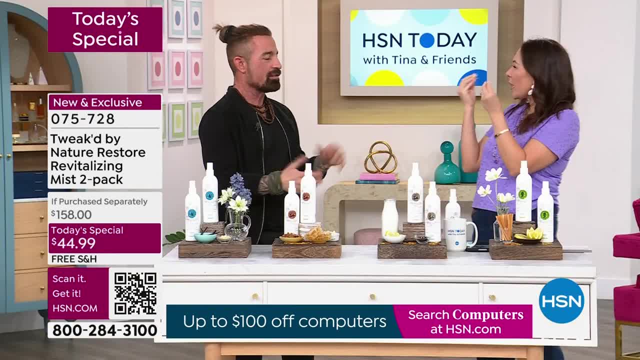 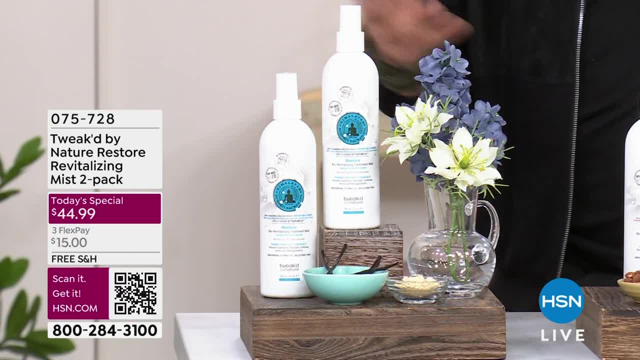 It is the fragrance you like, but just Floral. It's a floral powdery clean. and then you add this milk layering element to it Out of all the ones that I had. it blended perfectly, Of course. it is above the clouds. 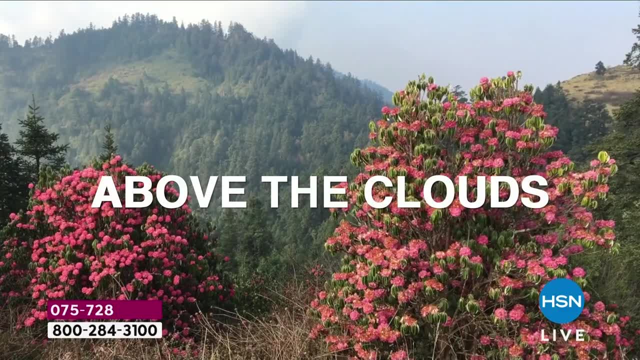 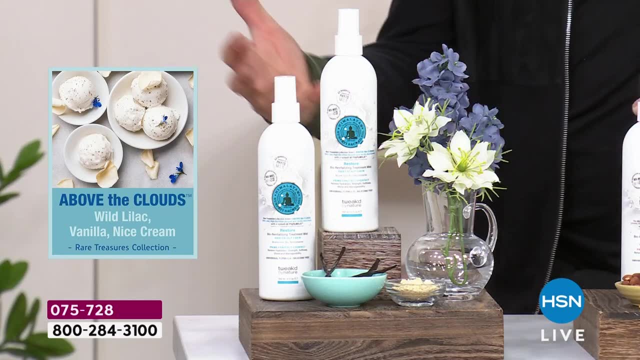 It's magical. Yeah, So you're playing with the Rhododendron Anthropogon, With buddhist monks, the florals that they use, they grab them for a reason. burn it in the smallest areas fills five to the seven chakras. 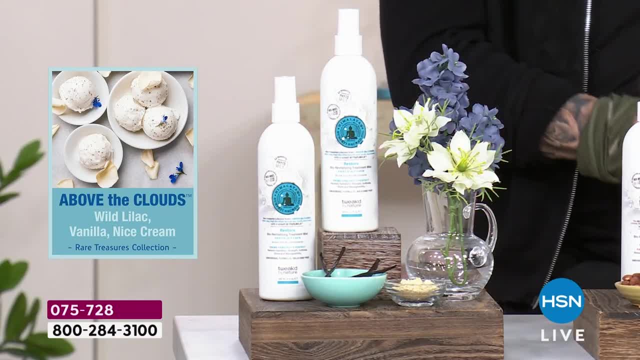 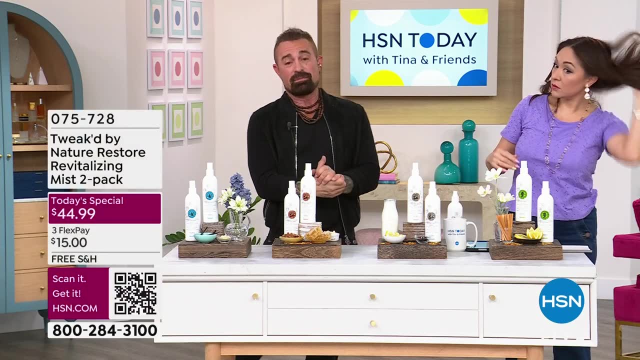 So the above the clouds, I would say it's more balancing, Absolutely, And it's the floral out of the bunch, but it's a powdery kind of like baby powder. baby powder, Yeah, A kind of just very, very light, but again, more movement. 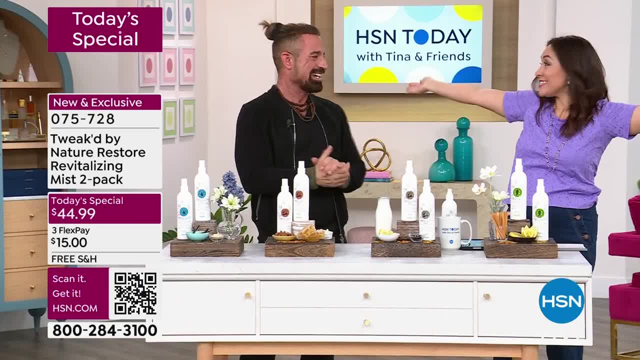 So if you're doing jumping jacks, you'll be like I smell amazing. Yeah, exactly, And I, I smell amazing. If you want to go and like, if you want to be like kind of undetected, then yeah, then. 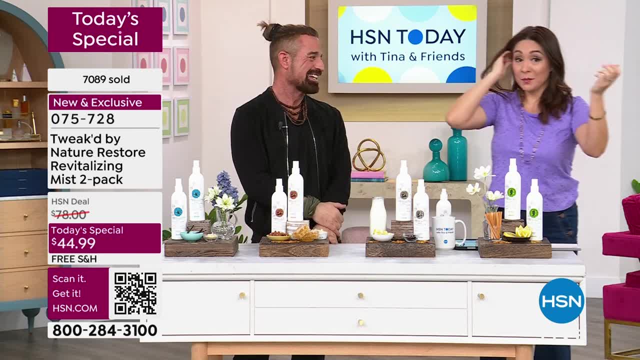 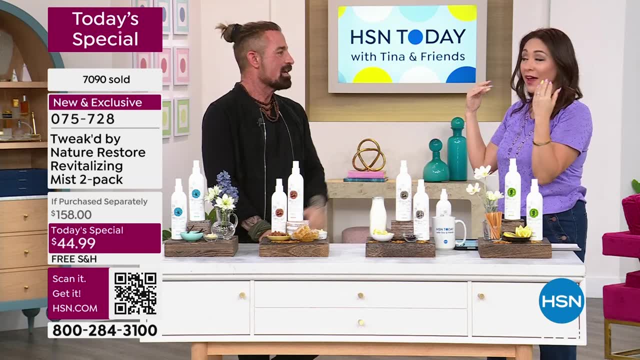 you just move really slowly, Mime, everything like very slow movements. If you were just waking up, this is our today, special 25 years of saying: Not yet. This is like a the big one's coming in June. What? 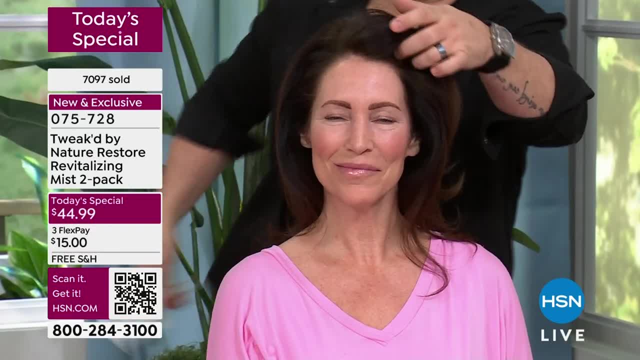 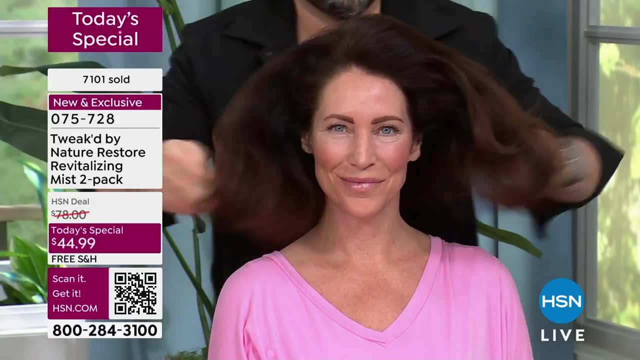 This is like an appetizer. Well, this one, yeah, it's so dear to me because I made it for my daughter 25 years ago as a detangler And I'm not a hairdresser, So what Johnny's doing there? 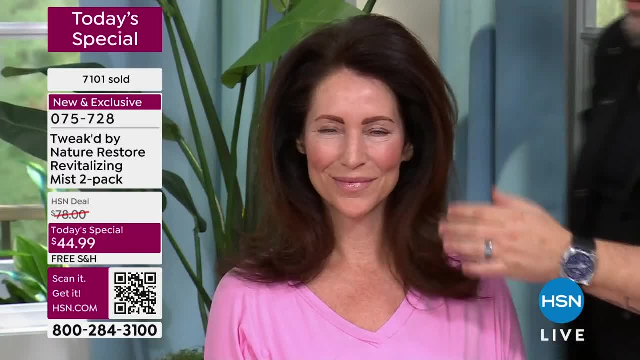 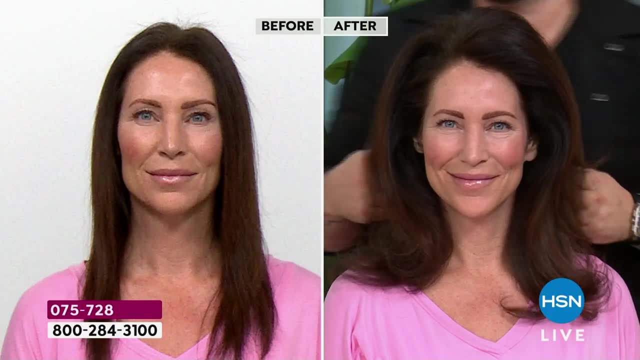 With his comb. you know, if you're a detangle, you want to start from the ends and you work your way up right. I was going at her from the root. Johnny was like: oh, what are you doing? She was crying. 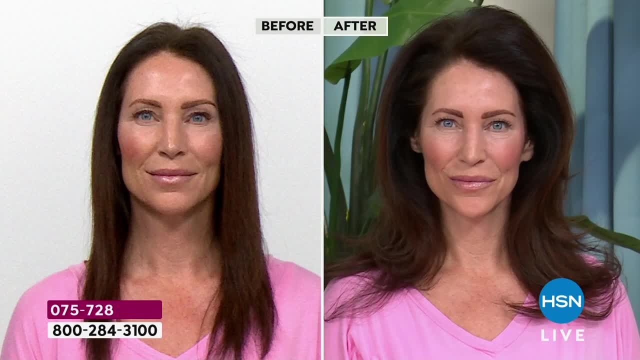 And then that day, when she started crying and I said I'm just going to cut it, And then she started bawling, I'm like, okay, I got to do something And I made a mist and it became so popular and survived 25 years. 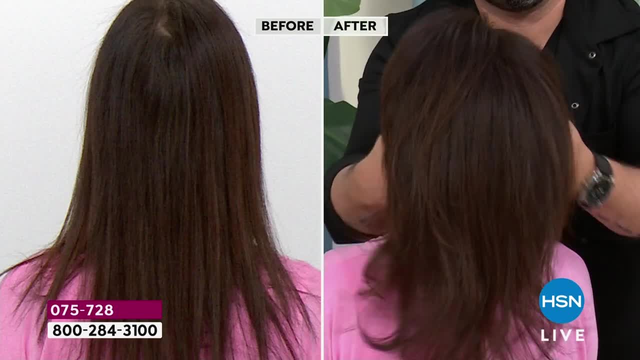 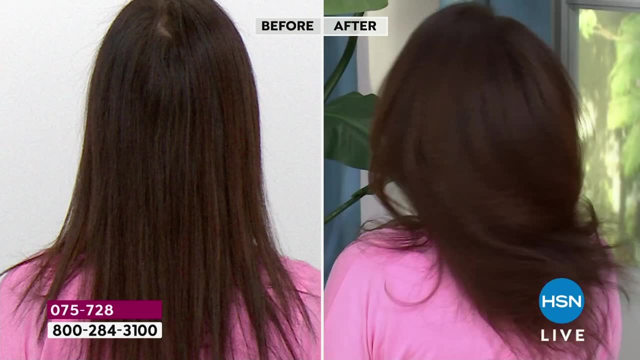 Then we had to kill it and resurrected it And and, but I knew this was coming, So I- I I needed to carry That Ozone peel- finally got to use it. I've been building it up, building it up and, oh my God, it's so good. 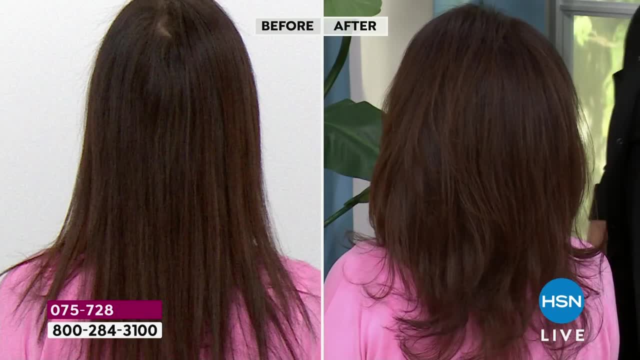 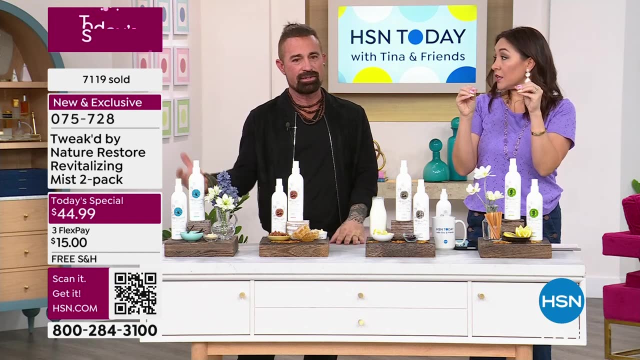 I will tell you people. I think, if you're waking up and you're, this is a whole, whole new thing. for 25 years you've never heard of this before You're I want to talk to like a brand new, clean slate, a clean Nano that, like the Nanos. 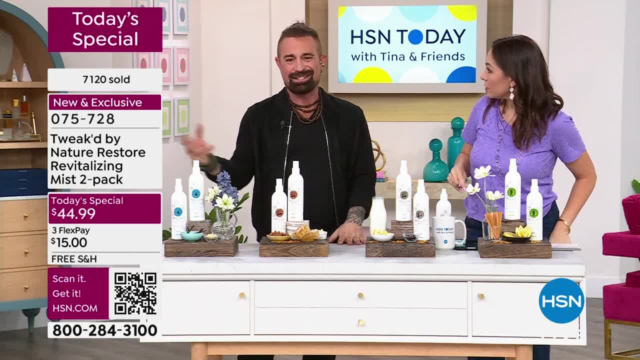 I think we've got a lot of bad press. but cause they're? they're made, or this. then the metals that are inside right, Who wants that inside? This is water. that's what they could react to it with. 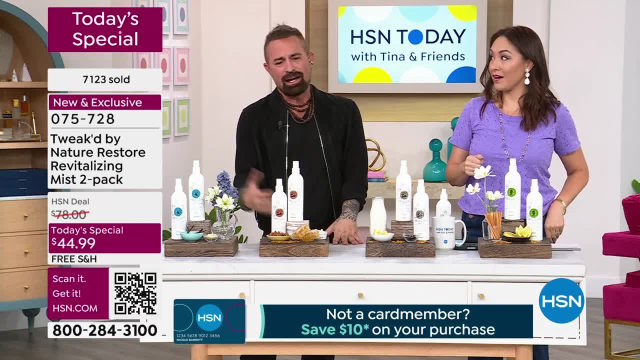 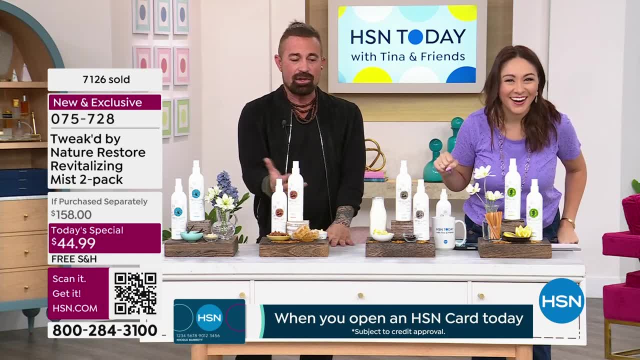 And that's why it turned into a milk. Ah, lost the orange color, um, and it's so absorbent and, of course, yeah, it's like, finally, i found it. it's a vehicle that holds and that carries, so it brings it in. the smaller the molecule. 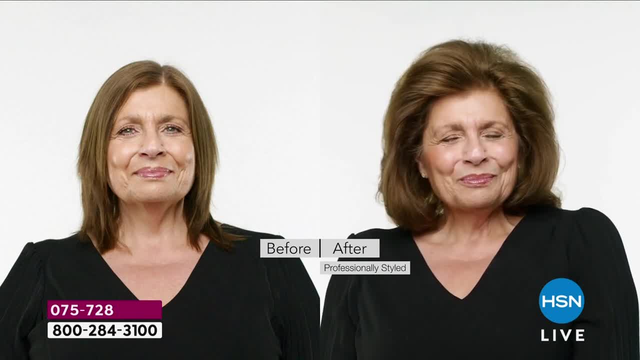 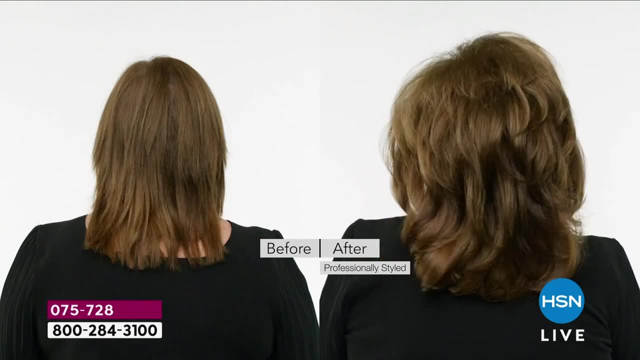 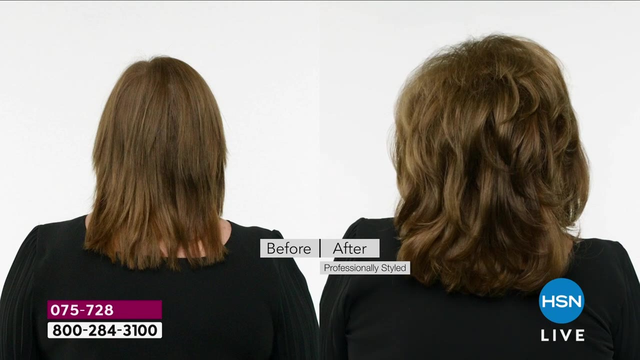 better. it carries. it's 400 sizes smaller then yeah, this is the ferrari for carriers, the only one as far as i know, the only one that is that clean. they're a an outfit out of brazil. they call it nanoscoping. um, do i have the bonus by out here? i wouldn't use it if it wasn't. if it. 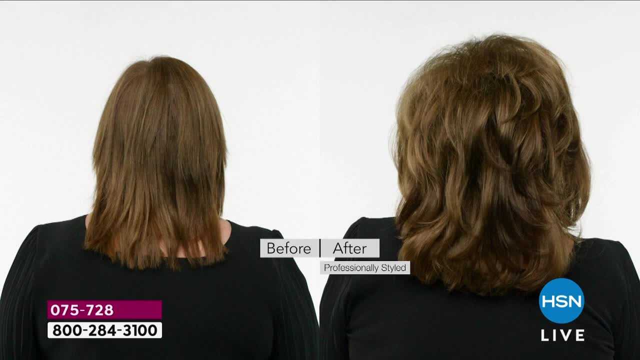 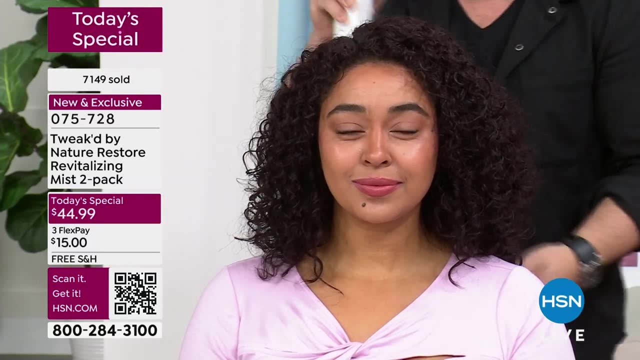 wasn't clean, so i'm, i'm putting it all over me. yep, i'm bathing in it. i'm telling you on my hands this morning and i was like: what did i do different? it was this, it was this. and think about your scalp. this is i'm. i'm a bad friend. well, i'm just gonna put it out there because i totally 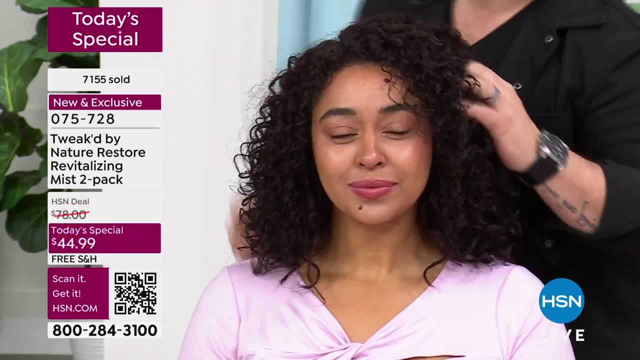 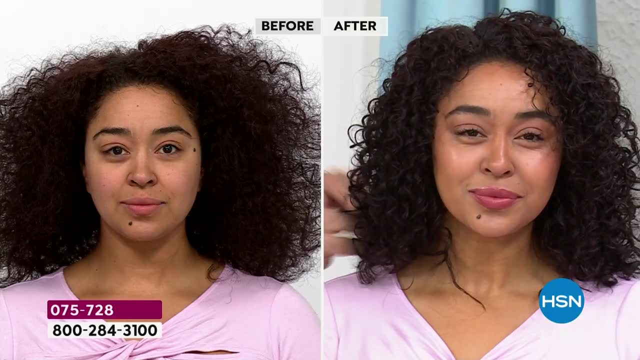 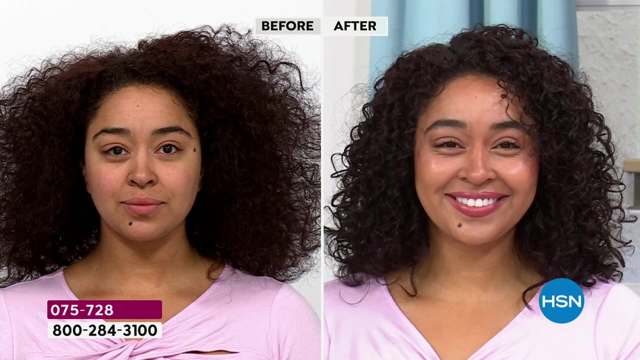 forgot to add this at the beginning: grab your today special. we were so excited about this again. look at kenya. she's got you know: thick, curly hair, thin hair, lifeless hair, super damaged hair, frizzy hair. this is gonna love me because you get definition to the curls. oh my god, yes, uh, look right, i have wavy hair. a man has wavy hair. then 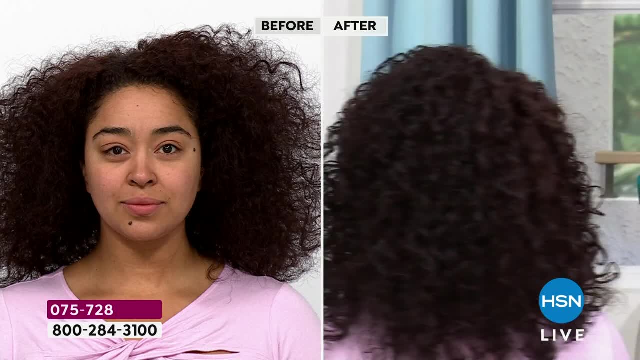 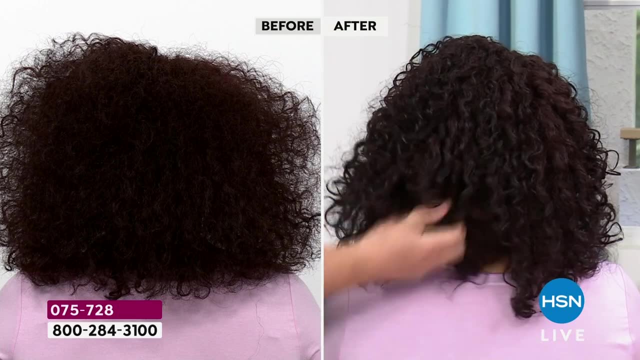 daughter curly. but every we always see a strike because we're always the opposite of like everyone else on the planet. but if you want the perfect ringlet, um, this is going to give you that. and the way it works. again, it's a creamy milk inside that bottle. really more, not even a milk, more of a. 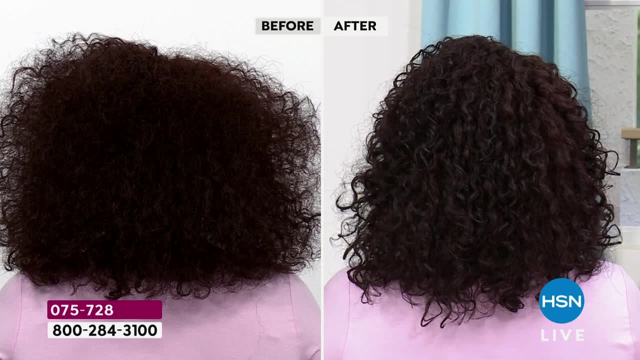 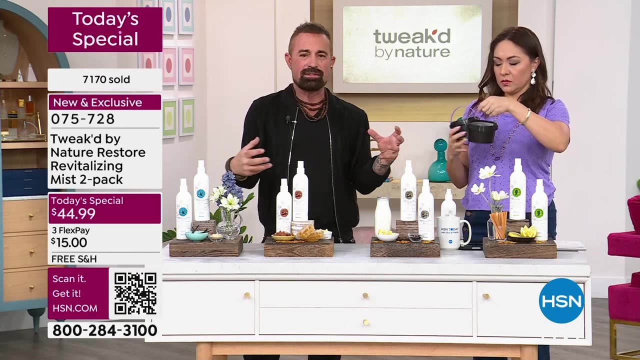 cream than when it hits. yeah, that comes out the chute and it has movement. it breaks down to micro fine liquid that now attaches and as it cools it solidifies again. so that's how you get the definition. but it's soft, there's no hold, it's. 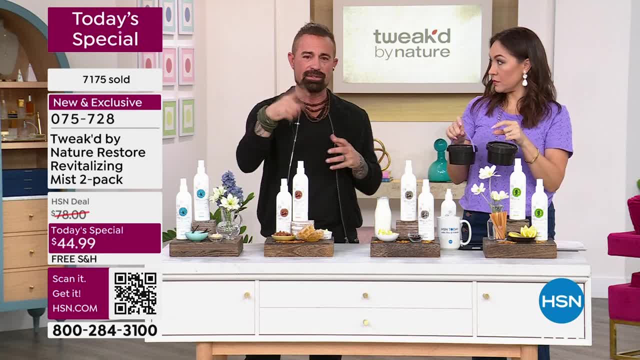 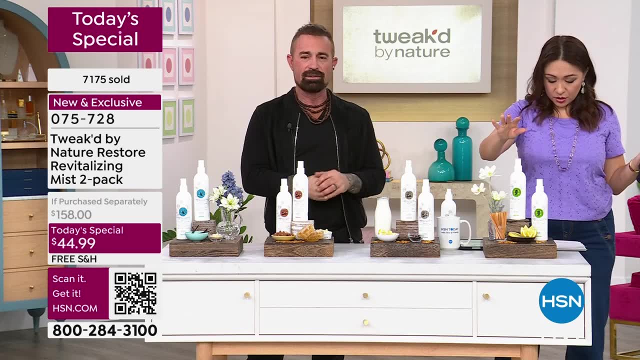 not crunchy. there's no alcohol, no silicones, and it holds. it creates this, this nano film onto the hair veil. that's breathable and it's you'll see. you can just use your finger to ringlet or trait the ringlet, or you can blow dry with it, set with it. you can't do it limitless, yeah. 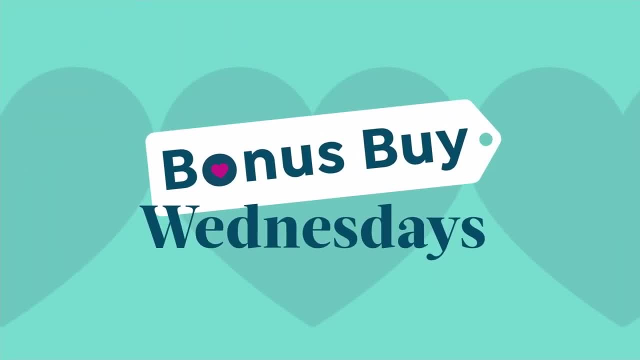 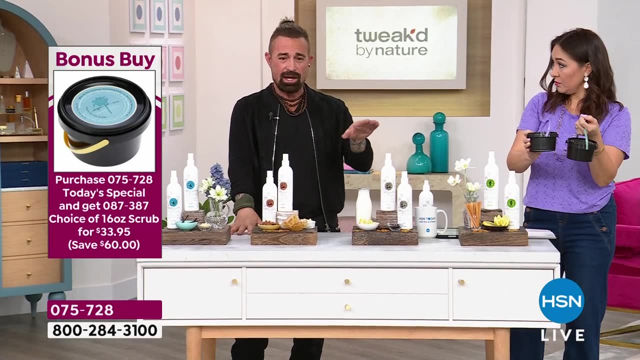 you cannot do this wrong if you're like: when do i put it on? you can, though, and that's why we did the bonus, because if you've got build up and it can't get through because, as soon as you get it home, if you're not seeing these before and afters, i mean 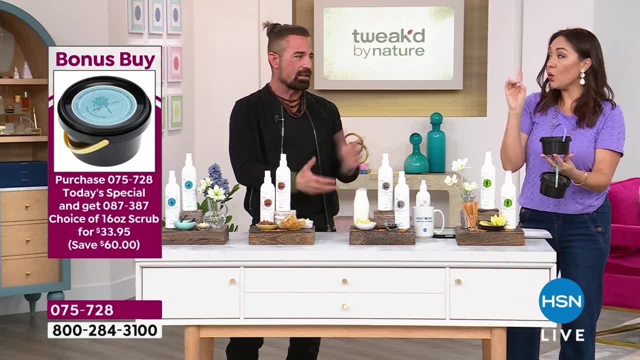 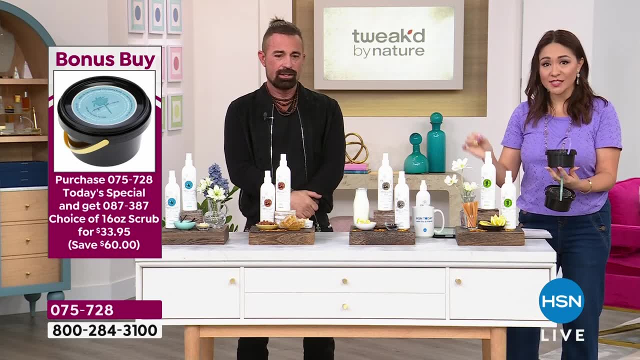 a dramatic difference. there's something. there's something in its way and that's why we did this: wednesdays for customer appreciation. we're doing bonus by wednesdays. so what this means is, if you were buying the today special, and only if you're buying the today special, this, this bonus, buy only. 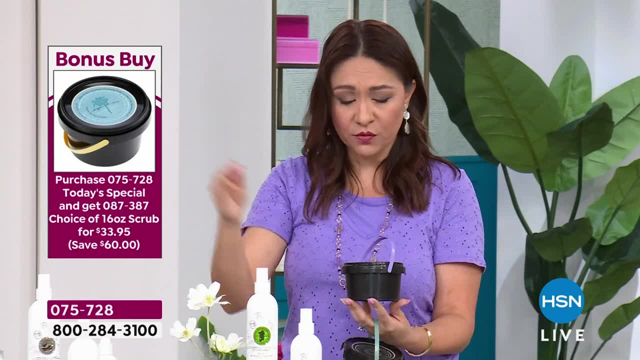 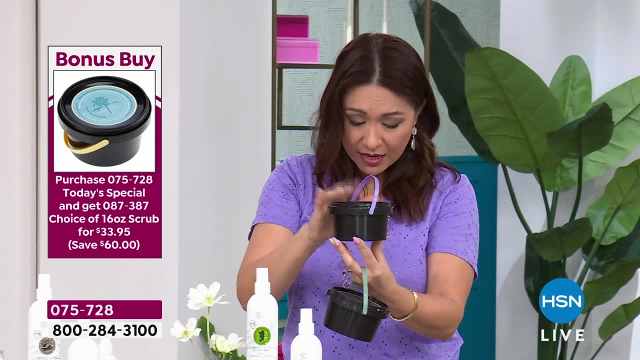 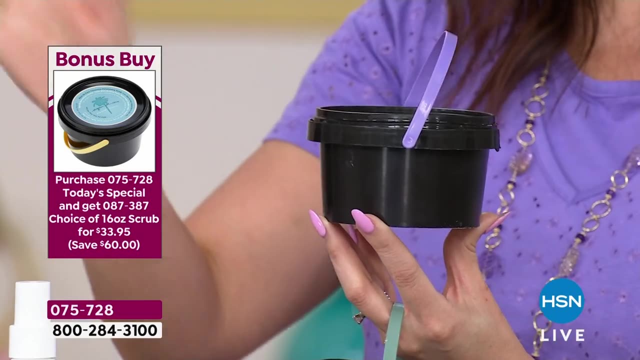 applies to you. if you are not buying the today special, you have to get this at full price, this cleansing, volumizing scrub. this would normally be 93.95 um as the bonus buy. so if you want to buy it for almost 94, by all means do that. but if you get the today special, your volumizing scrub now. 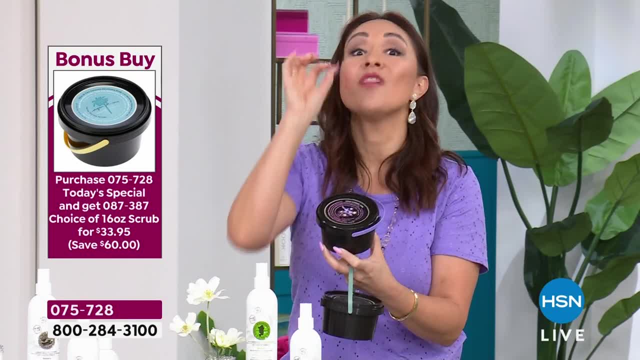 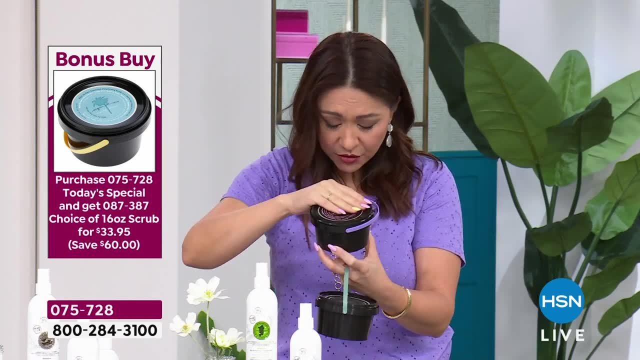 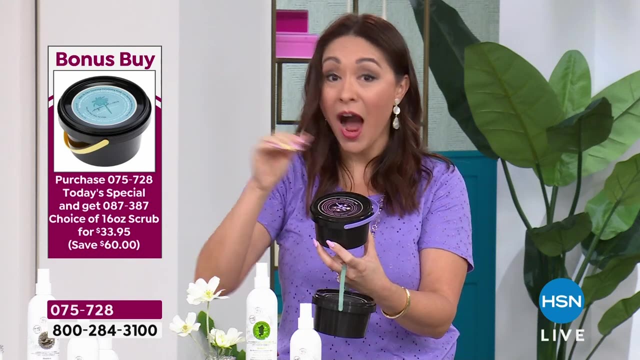 becomes 60 off. 60 off to get this only if you're getting the today special, which are also getting a great deal. um, i will tell you in the scrub. this is an average of eight hundred and eighty six percent increase in volume. i don't even know that number. it could. 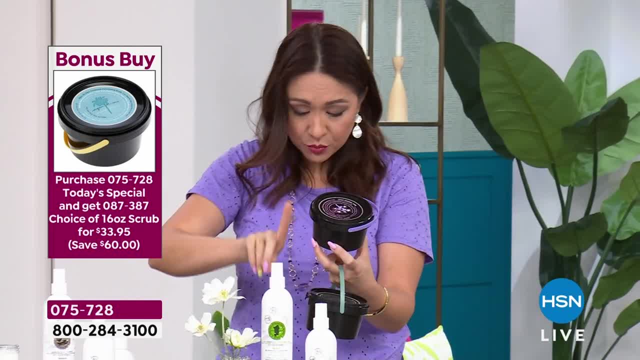 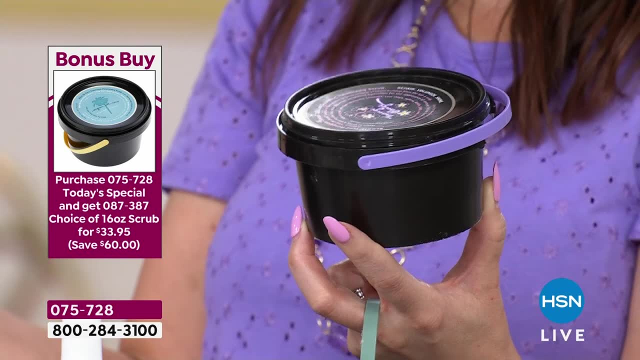 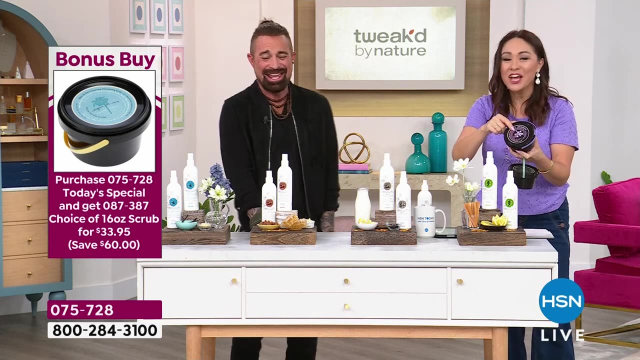 exist. right, i will tell you, i have lavender rain, we have the tulipia, we have the wild. how do you say wild, friend, friend, friend or friend? well, frangipangy, frangipangy, is it frangipangy, plumeria? so i always try to mess you guys up, so that's why i didn't. this is how you know it came. 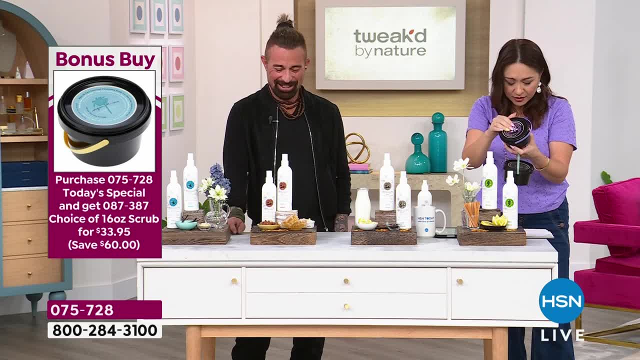 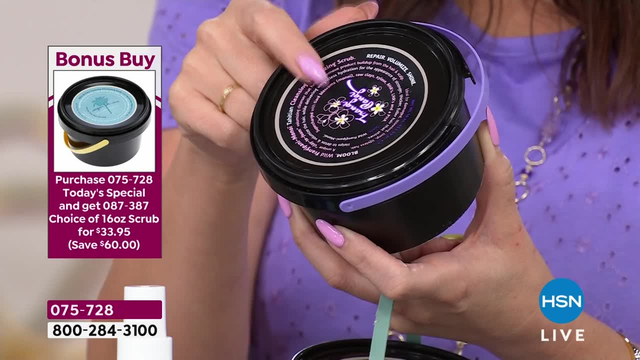 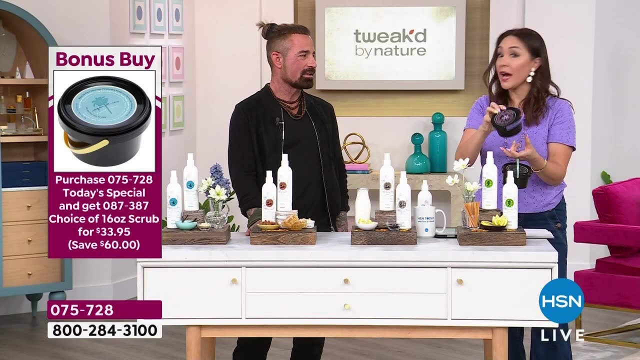 from nature, because i'm like, i don't even know. we do have the honey lux, the above the clouds, the wild, uh, summer apricot and the agua de coco also, and the unscented, yes, um, as well. yeah, the unscented, that's the unicorn, so it always goes. yes, it does have a coconut available still right now, yeah, but 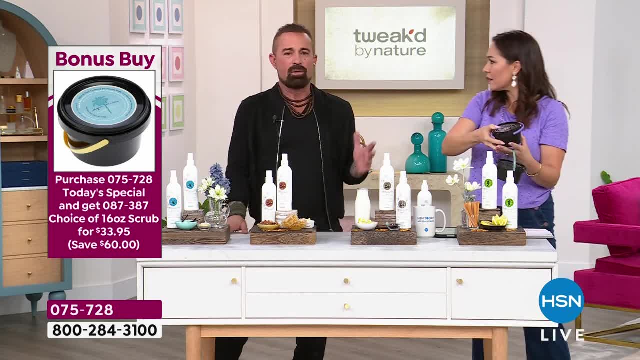 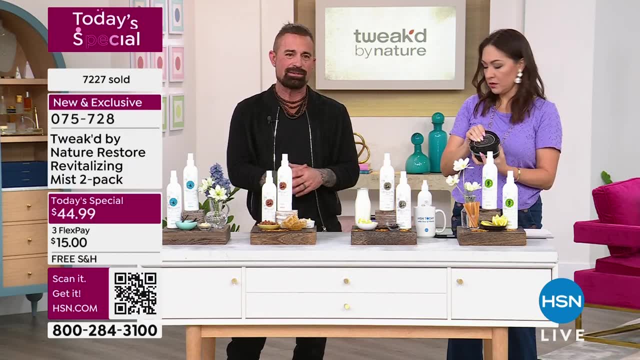 don't leave that free money. no, and look and- and i i'm not one to upsell- uh, if it needs it- and the only reason it might need it is if you've got a cell, there's no silicones in it. if you've got something that has dimethicone in it, you're gonna need it because that dimethicone takes a few washes. 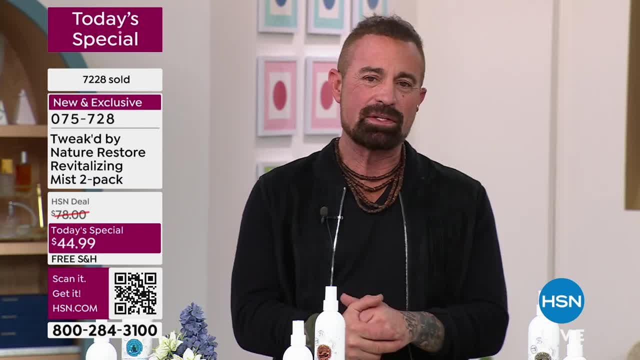 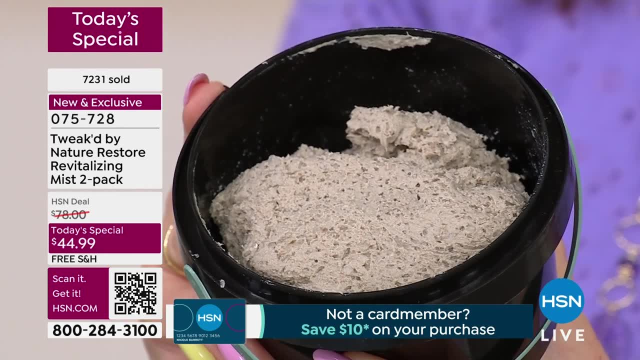 out if you're using a shampoo, this will eliminate it and gives me that clean canvas. and and when we do our testing, this is what we do, so we, even with the models, we'll scrub first, so it puts us at ground zero, and that allows now the product to work the way it's supposed to work, and then you. 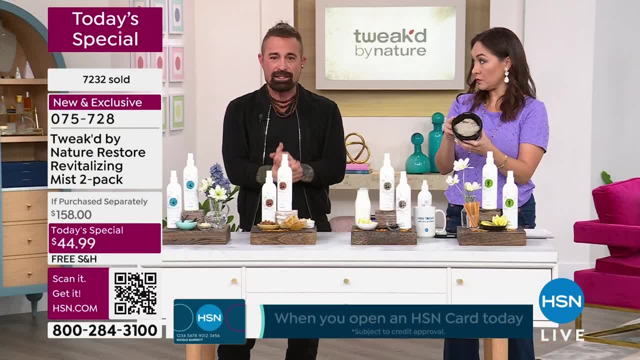 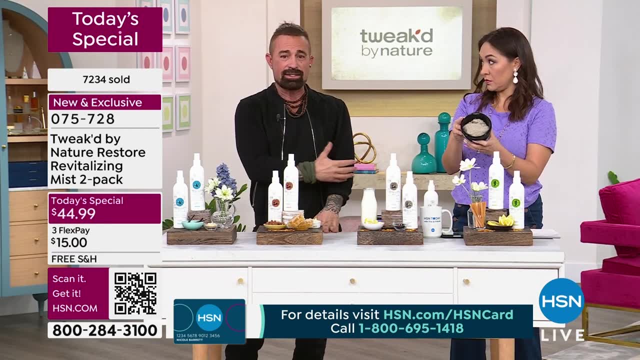 get, and it's not even just our, it could be anybody's product. yeah right, it's a clean canvas, and that's why i've done this, because i really want you to get the effect of how powerful this is. if you do it right, at least if the hair is equal right, because i don't know what's sitting. 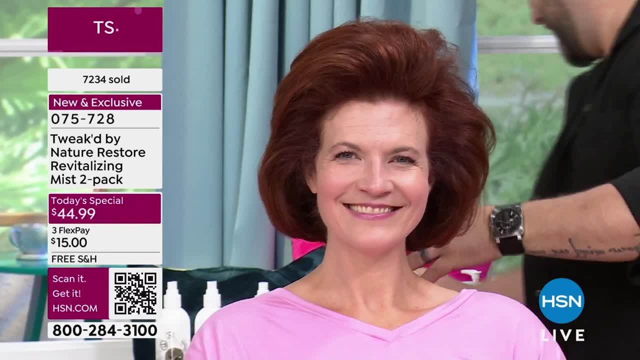 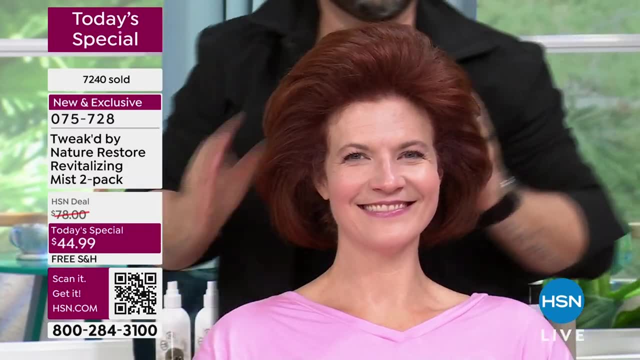 in your hair. this will this will allow me to know that you're not going to be able to do it right and that's why we do the price that we're doing right, so we're literally almost giving it away and it's removing all of that. on the scalp right. you have to start from like square one up. it's. 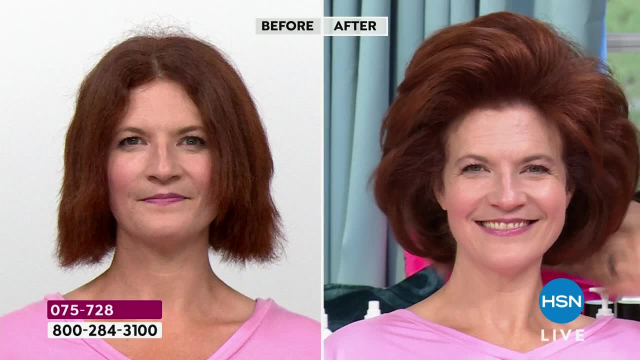 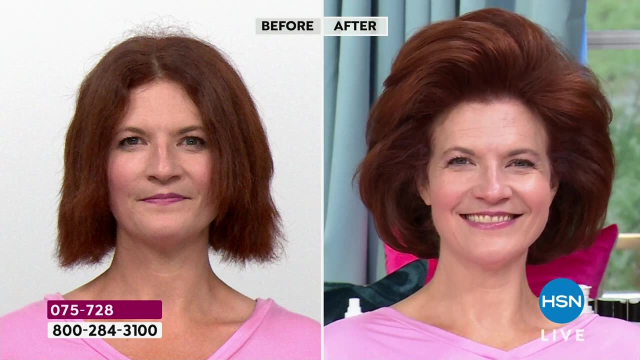 scalp all the way to the ends, right. so it's important. scalp wise, that's for tomorrow, the next day, right, new growth. but what if you want what you have right now sitting on the outside to work hair wise? that's why we scored a 900 increase in volume, without styling, but it's. 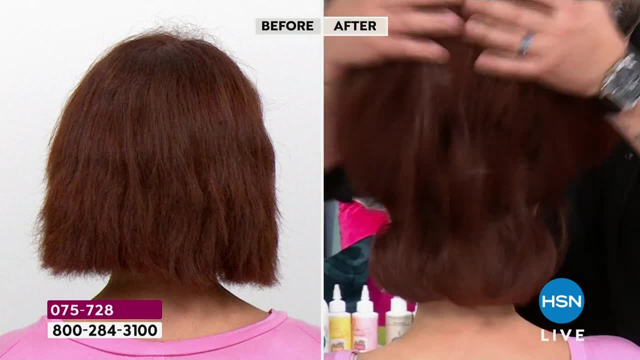 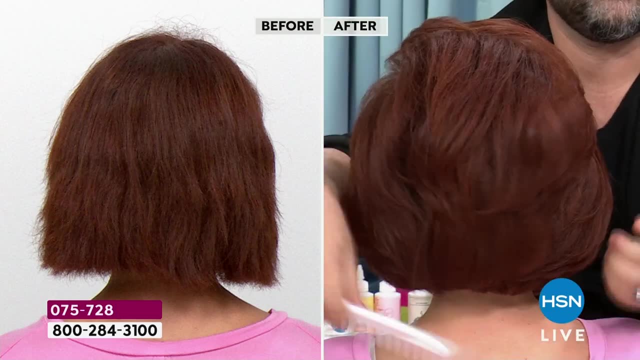 because we got rid of what was holding it down. yep, so this, even though the nano could get through. but for a full effect, you try it and you got a year's supply. in that bucket there's a hundred applications. you only do it once a week, right, it replaces your shampoo once a week and you bring the mist in. 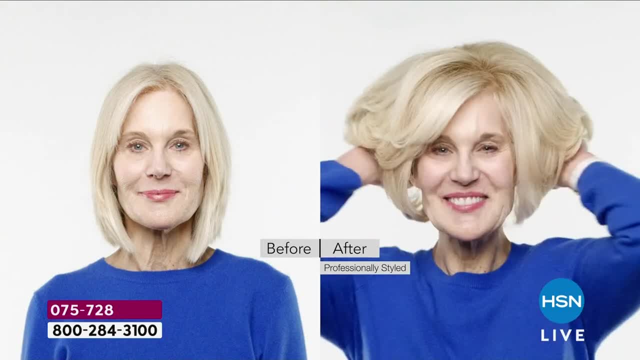 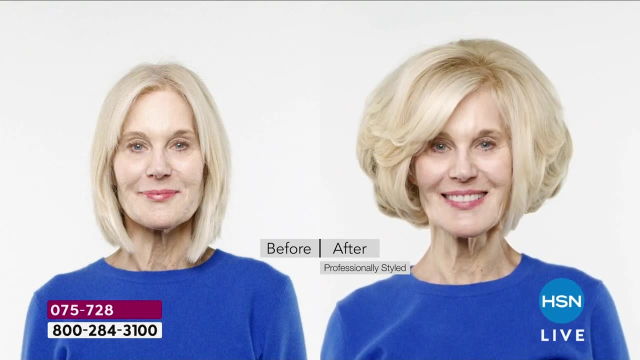 instead of your conditioner. you'll see, there's nothing better. lisa, on our facebook live now question, she says what is the least fragrant of the four options. so if somebody's looking for milk, the phyto milk, that's what i would have said. yes, it's, it's a layering scent, so, and it'll, it'll. 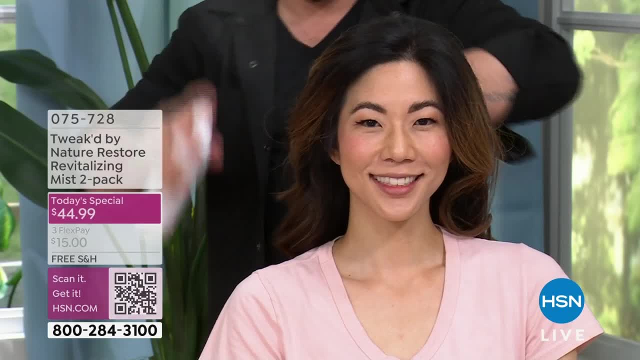 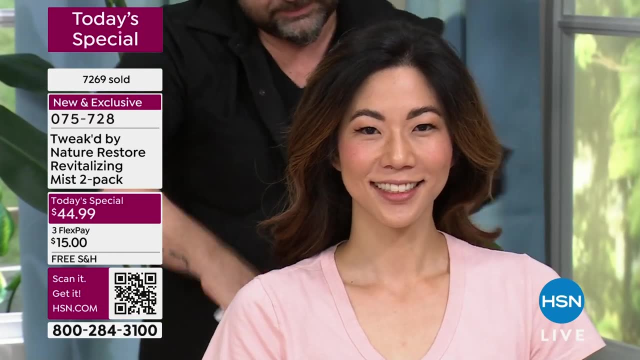 tie into whatever else you wear. it doesn't matter even how dramatic um or light it. it blends and remember you don't when you apply these on the initial burst, because it's traveling, so there's movement. you smell it and it's not that it's strong and you're smelling. 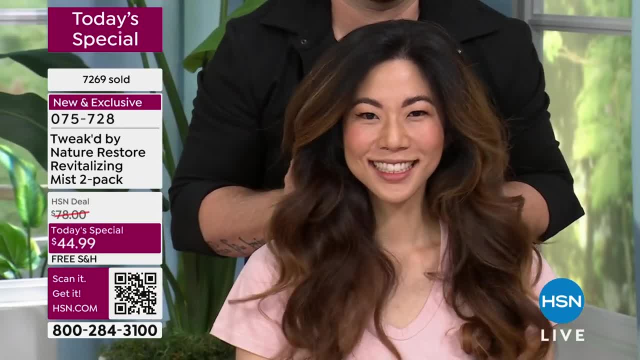 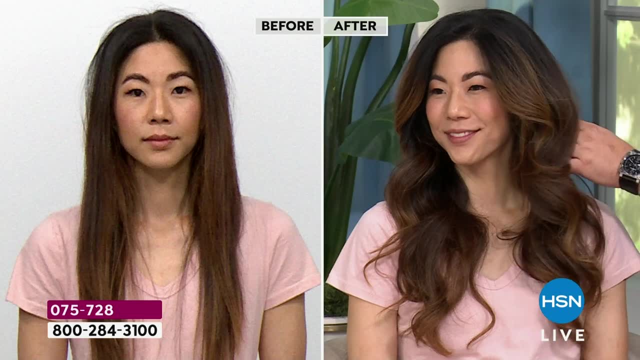 all of it as it attaches. it dissipates only when you move, and and there's a change, either temperature wise, but more movement, um, that's that's when the aroma comes back. so it's going to last longer as well, and that that's what's the cool thing about it. so, morning to evening, 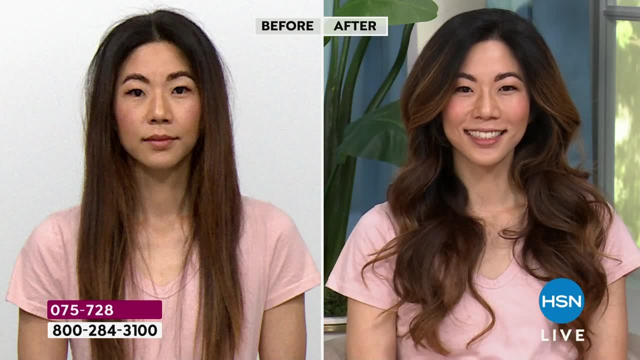 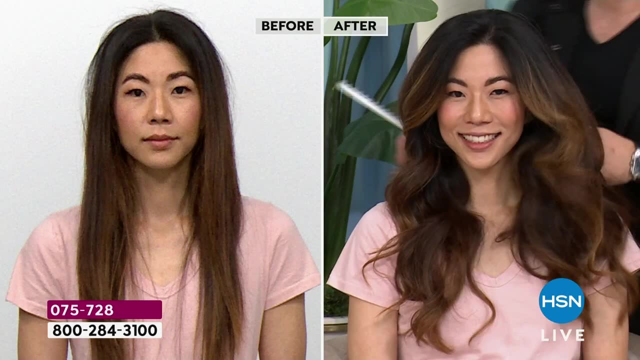 when you reapply for before bed, it'll still be there rinse. so this is, if you want to put it on right before you go to bed in the shower to help you detangle. if whatever you're using now doesn't work, you bring this in and it just makes everything. 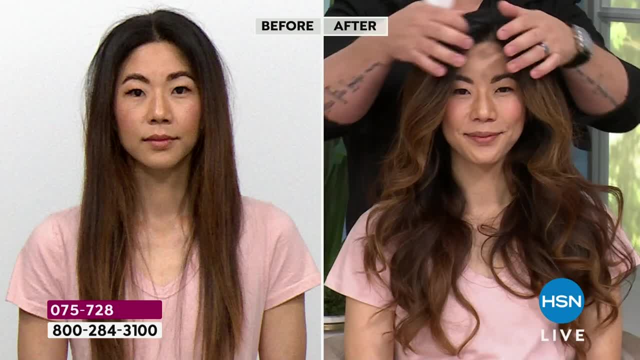 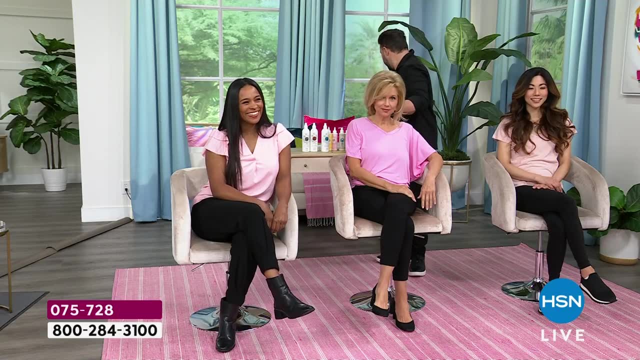 better. yeah, um, it could be your leave-in conditioner, but you can detangle on dry. that's how strong it is and i use. i did. i never tell you. i used to have the other bottle, that we the original, the original bottle, yeah right, and i used to keep it in my bag. i did for you, do you? 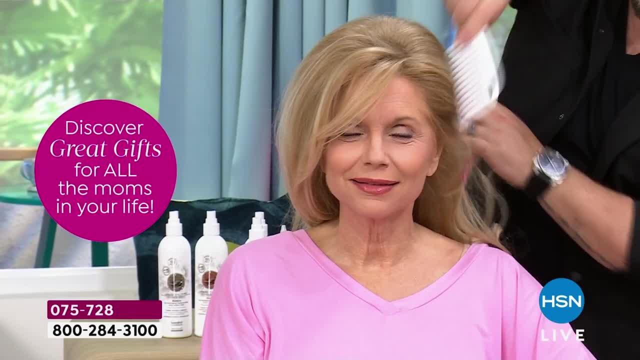 want to know who always stole it from me. well, let me get amy morrison. she'd always ask: do you still have that in your bag? and i'm like you're amy morrison, don't you have like 18 of these? and she's always like i need it all the time. 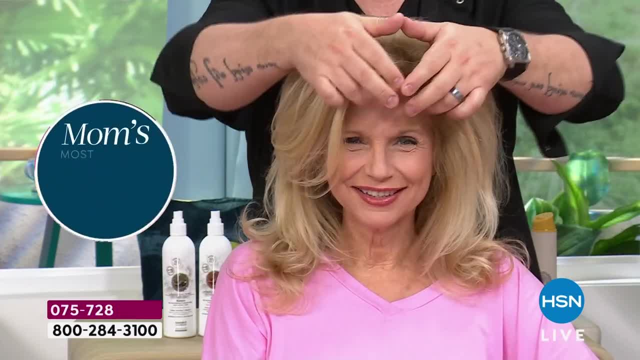 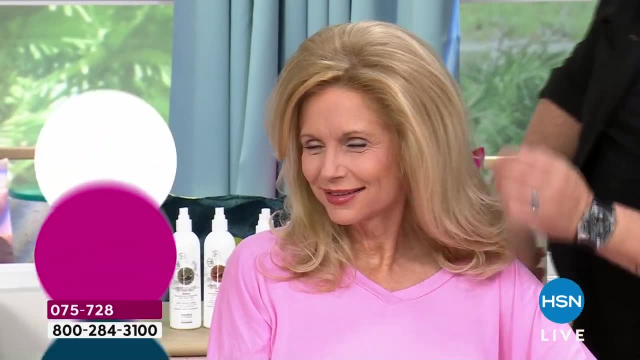 yeah, i used it because i would get flyaways. i would get kind of like that hair that needed like, just just like everyone. yeah, well, you're in florida, so it's all about you. know, how do you? how do you go against that humidity? well, you have to fill the hair shaft. well, this fills it because 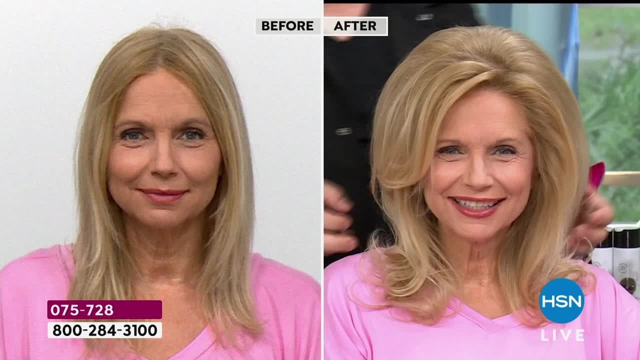 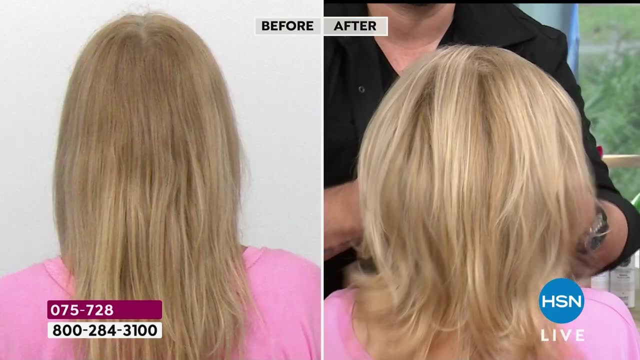 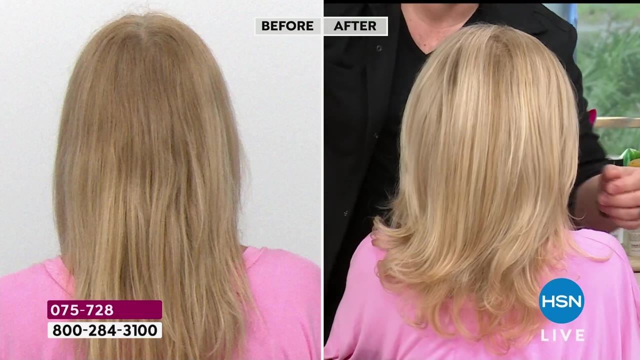 it's 400 times, almost 400 times smaller in particle size to you know our ojian oil, right, so both combined, um, wow, it's, it's. finally i got to put them back together. i've had them separated for 25 years: the shell and or the nut and the peel. the peel is a bright 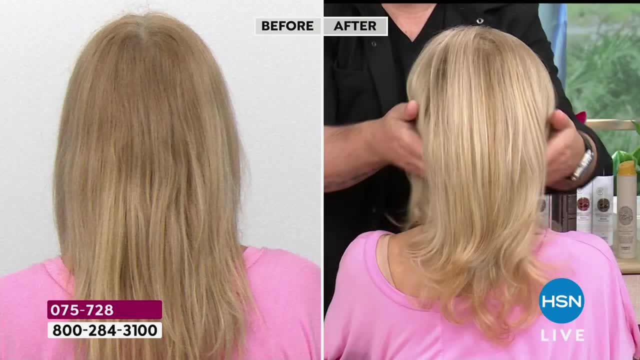 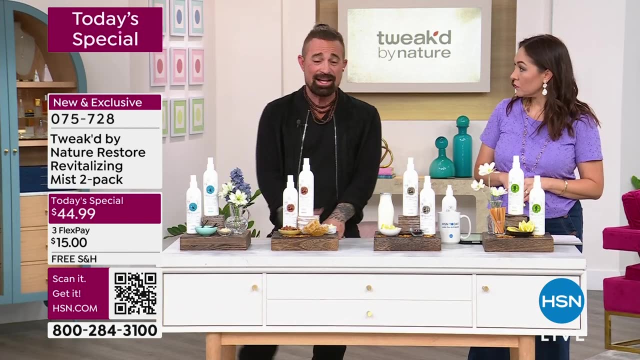 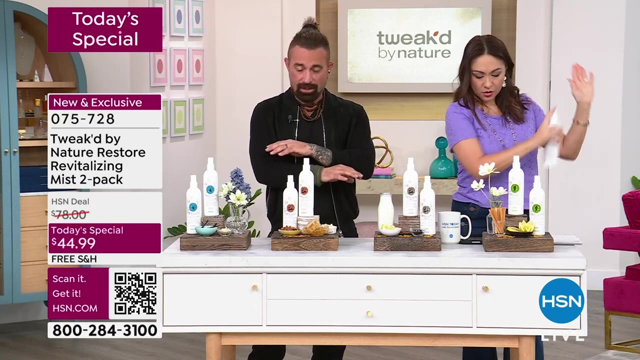 bright orange, so the milk is actually like a beige color that when they magnified it, it turned it into a milk and the first thing i noticed is where the orange go. yeah, um, it's there. it's just now encapsulated like inside. so it's just a beautiful thing. performance wise, it's. 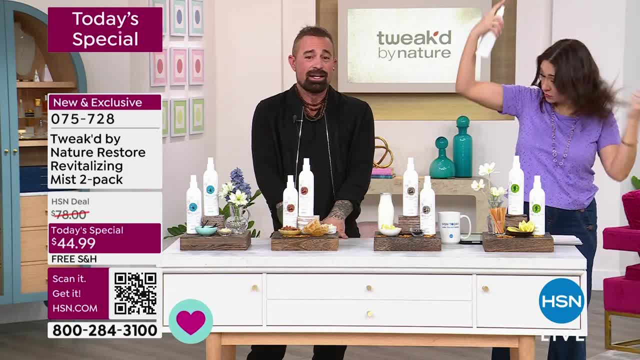 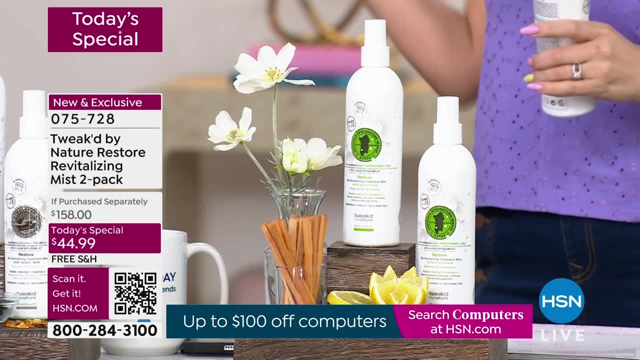 that's why i was going to wait to do not. i had to do it now. never see anything like it and a mist so easy to use. you just have to. you don't even have to shake it. no, the old one you had to shake this one. it'll shake on its way to you and it's ready to go. and then it'll shake. 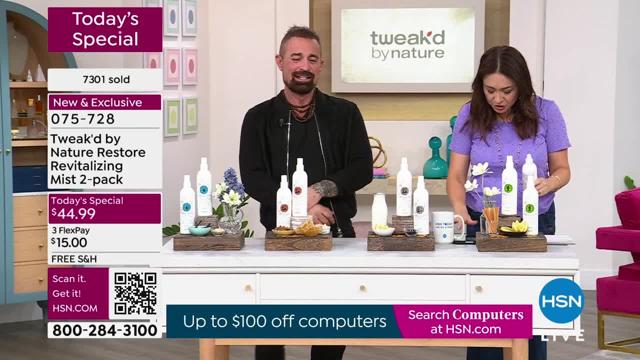 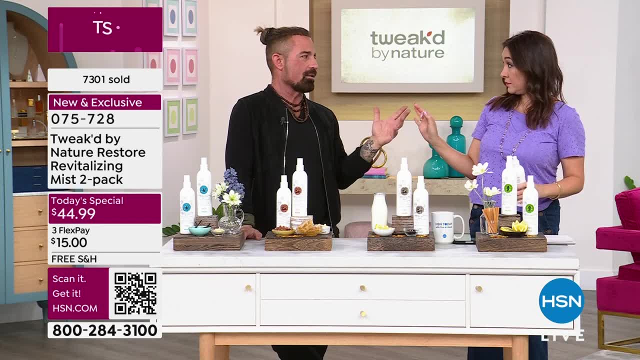 on the way to you. uh, gail is saying right now- i'm just tuning in- is this replacing the revitalizing it was in the past. so, yes, i see them retailing a thousand fifteen hundred. yeah, oh, are they aligned? yeah, well, that's what happened. it's discontinued gone. 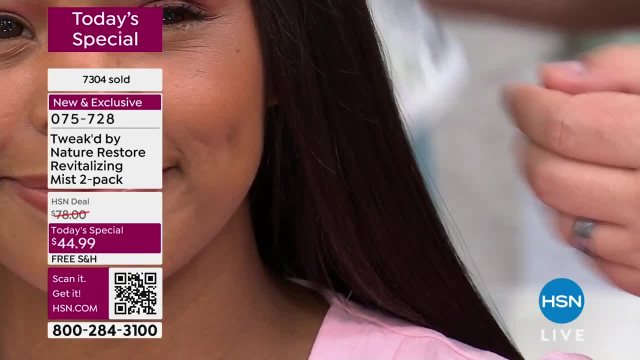 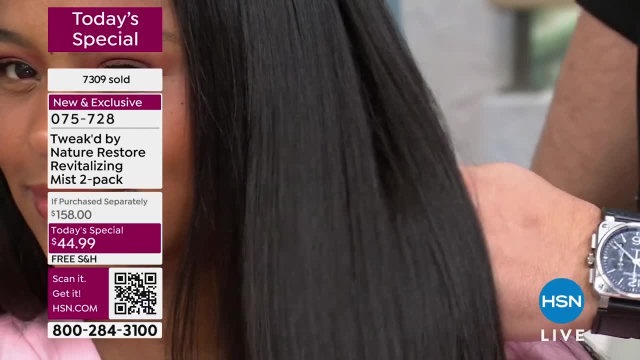 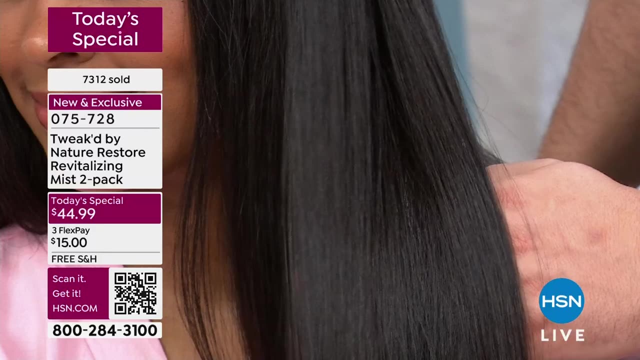 so yes, gail, that is the the first answer, but it is everything that you loved from that, but better. we've added one more element to it. it'll have a milk aroma to it, and there's no way around that, because that's, that's the magic. but look, look what you get like i can see myself. i can see that. 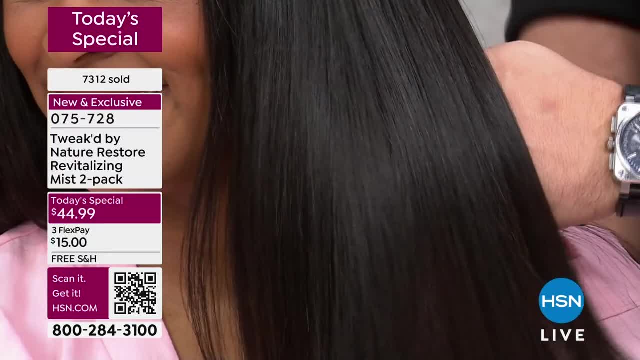 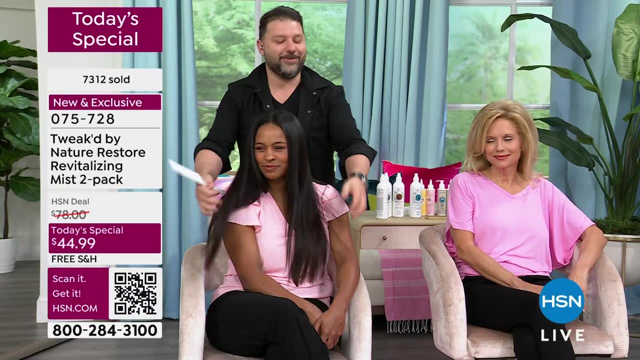 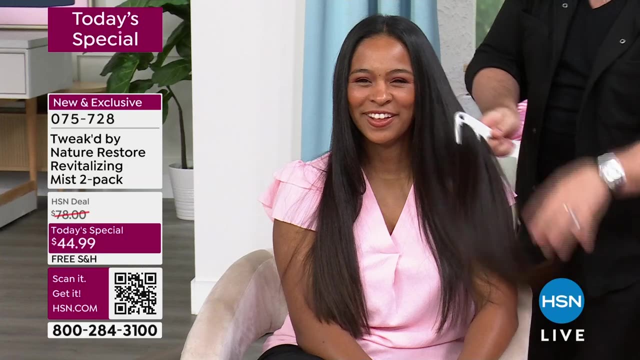 i'm wearing the same clothes yesterday. are you wearing the same clothes? are you lying? no, it's in texas. your luggage is in texas. yeah, that's what they, the airline, did you have. is your luggage here? they said: oh, we have a new worldwide tracking. uh, you know equipment and software that we just put in. okay. 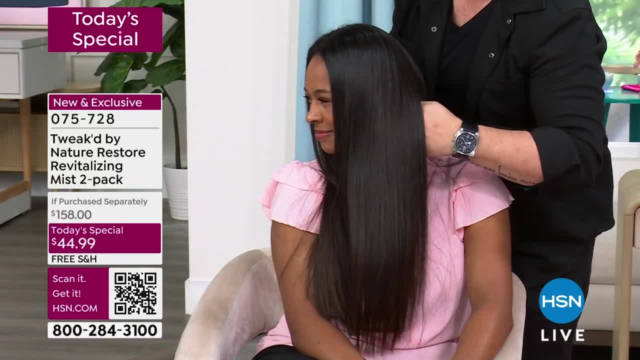 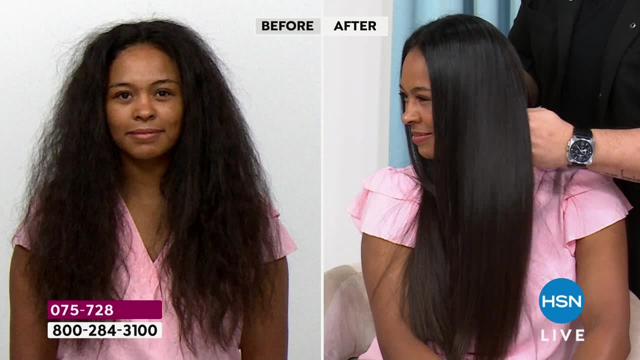 cool, so they were able to find it, but the problem is getting it to your eyes. that wasn't solved. look at this before and after. by the way, last night everyone said dania's before and after was the one that everybody was like oohing and aahing over because well, when you go this extreme from curly 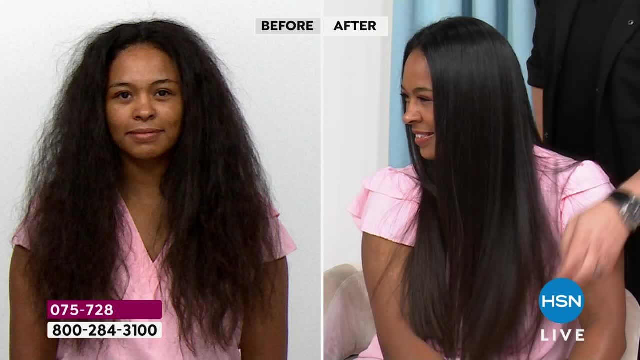 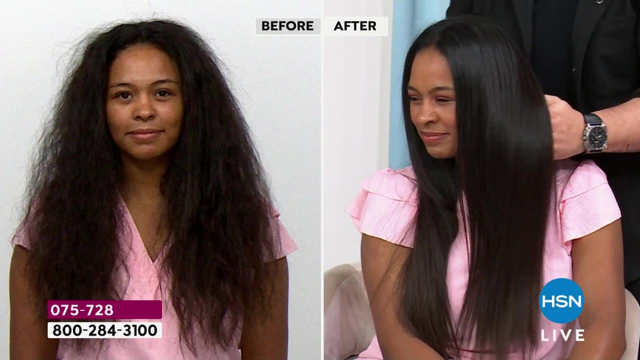 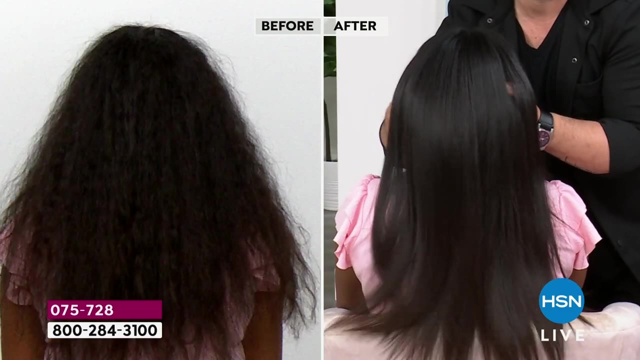 to perfectly straight. uh, heat appliance wise, you'll even find that that's even you know. you don't have to go as long, like, in other words, as high, even in temperature. everything is going to be easier, faster, and look in the end result. it stays with you as well and it's a qo of so like. 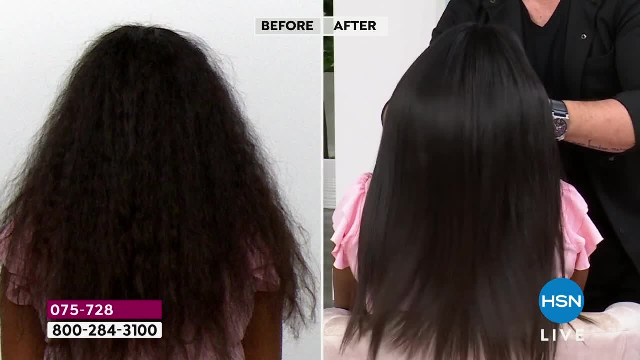 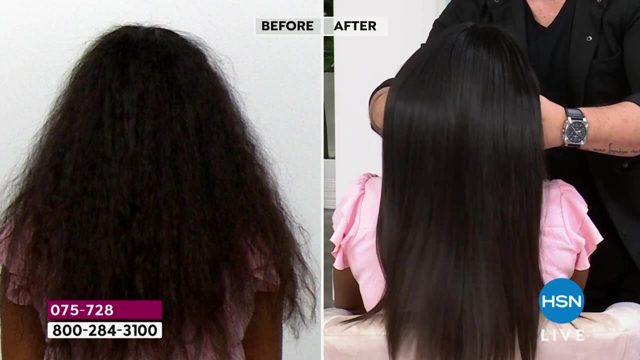 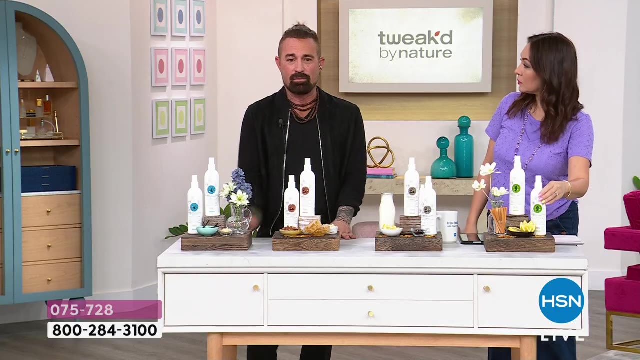 right there there's a film, but it's not silicone, it's this, or basically our ozon, that it was made, ozon so famous. the same fatty acid, same fatty acids, lipids that have found a healthy, virgin hair. that's what. that's what's coating. yeah, that's why it loves hair, because it's almost like a liquid. 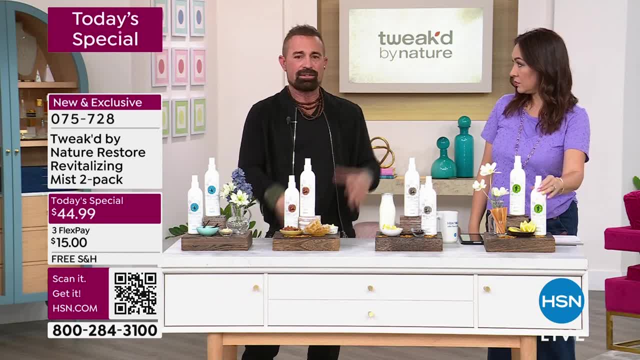 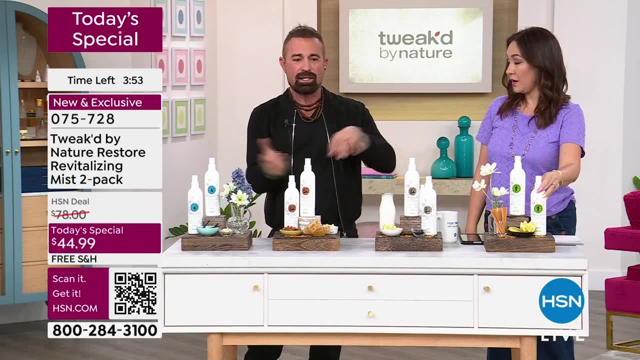 hair, really. so then, whatever's missing out of it, that's what i put in there, and that's what i put in to basically make it perfect, and that's the carrier. so that's what holds, and because it's such a smaller molecule, it's encapsulated, it travels to the air, attaches and there you go. 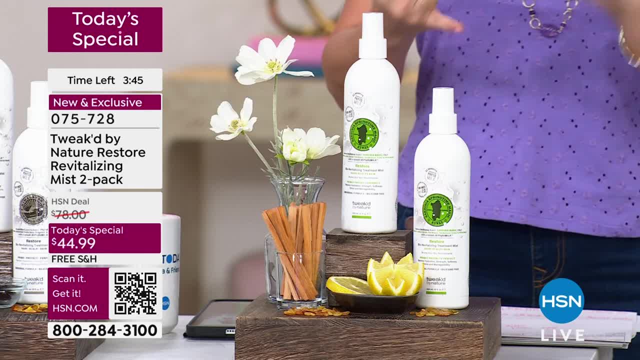 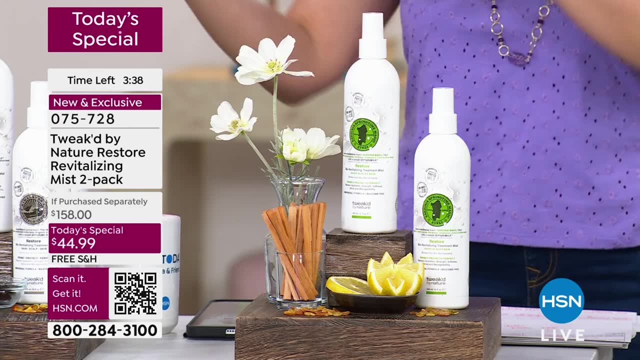 it's not a band-aid, it's a real deal. no, literally protecting your hair, repairing your hair. if you are those people that are like i- am so damaged, i am so brittle, i am so dry- this is almost, like you know, taking the hands of time and going back to a healthier version of it instantly, simply by 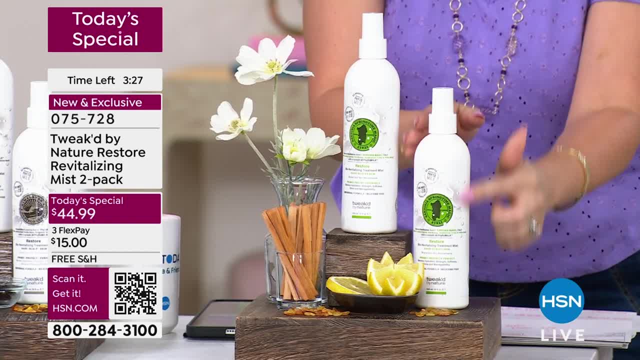 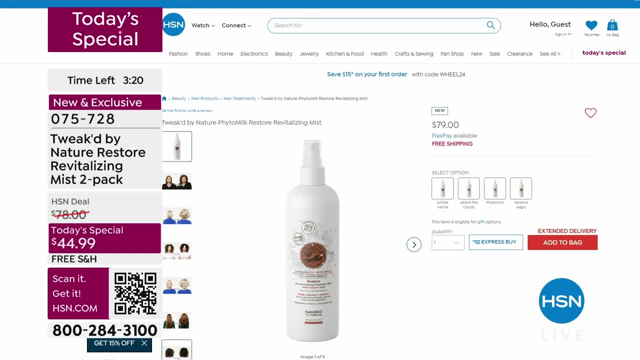 that's why it's so easy to use. you can just take it off and you can just put it on your hair. that's why one of these bottles is 79. this is 12 ounces. 79 normally there's all the scents, it's at. 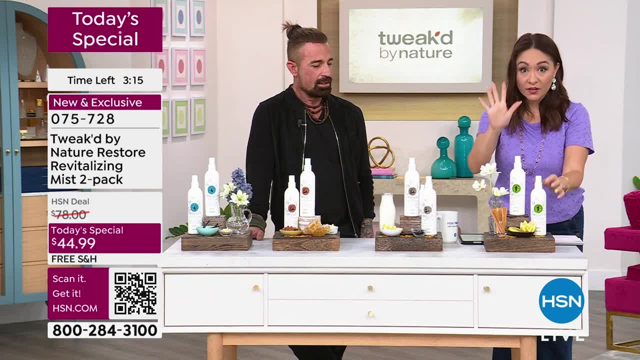 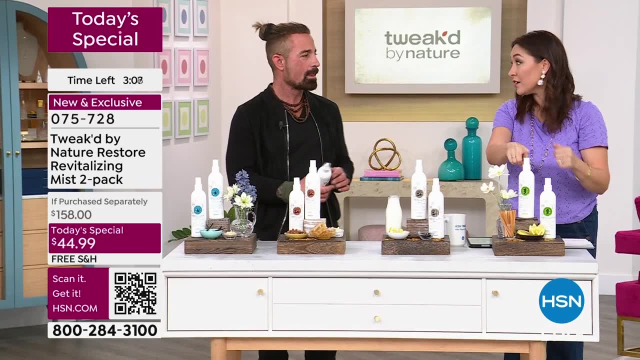 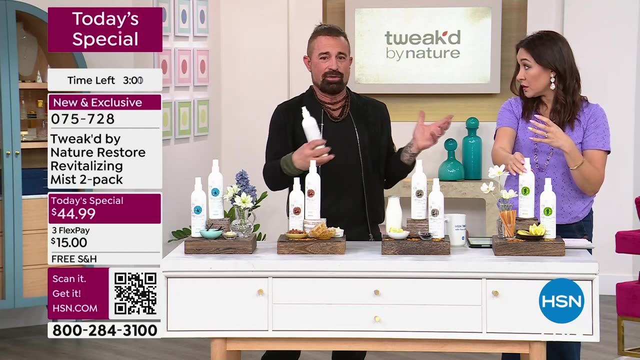 hsncom. i really hope nobody just jumps on the website and happens to see this one today, because, as our today, special one day, value being able to take a 79 bottle, take it down to 44.99 and give you not a travel, not a heavy right. there's 12 additional ounces, it's not? it's you think? it's like? 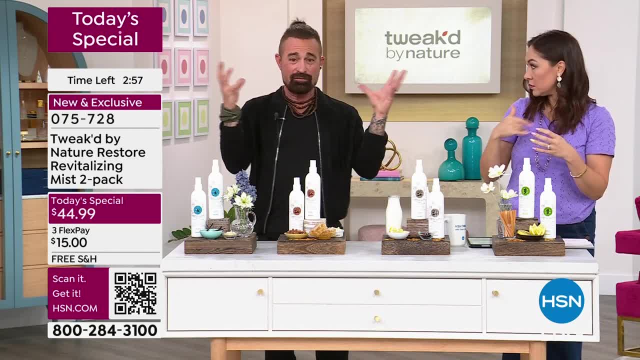 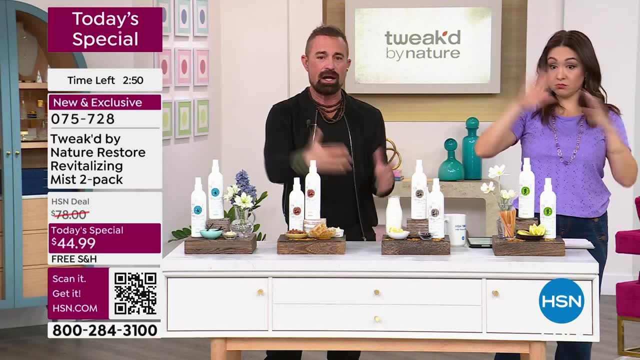 cream. it's so creamy inside but it jets out, as it's fine, fine liquid that you'll see it does not weigh down half the dose of what you were using before, so it's basically it's almost like double of what we used to have, because that's how potent it is and scent wise. yeah, so the sardinia magic. 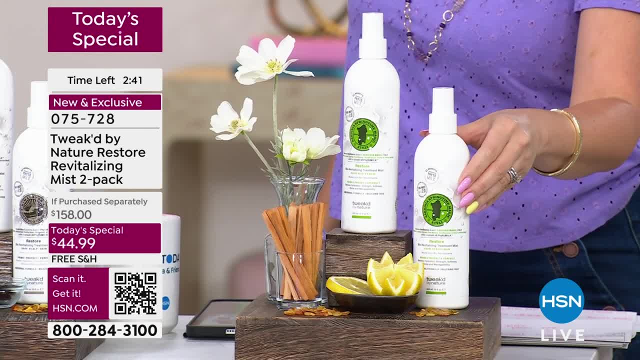 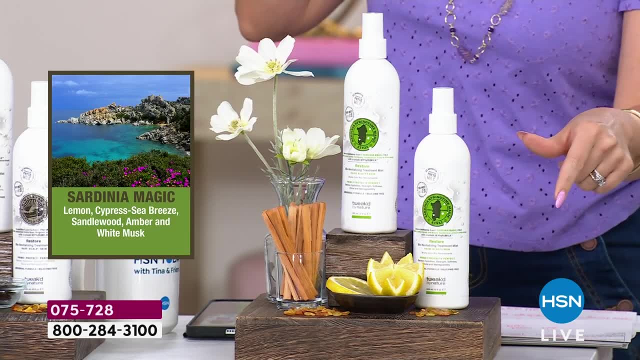 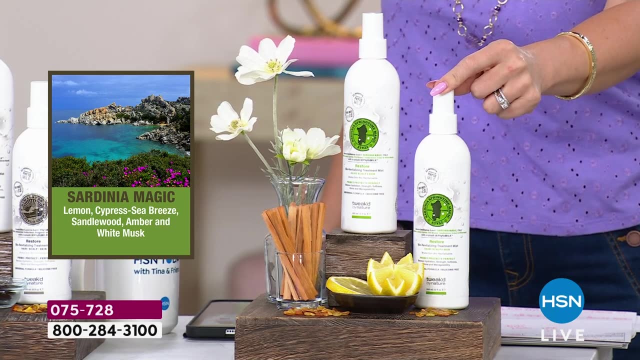 it will transport you right there. it's a morning terrace having breakfast. in this case i was eating fruit loops and at the end of the bowl so that mixed in with cypress, yeah, lemon limes, the sea breeze, the salty air- all combined with that amber as well, it's to die for it's. it's beautiful then. 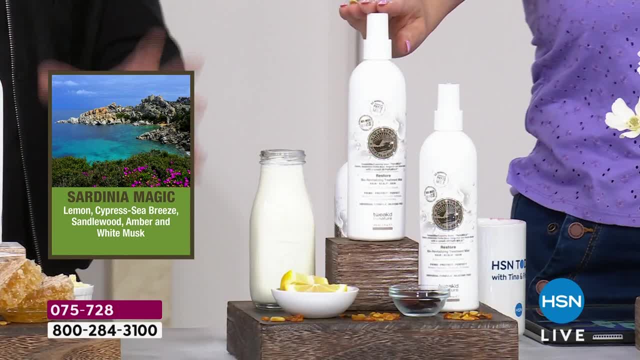 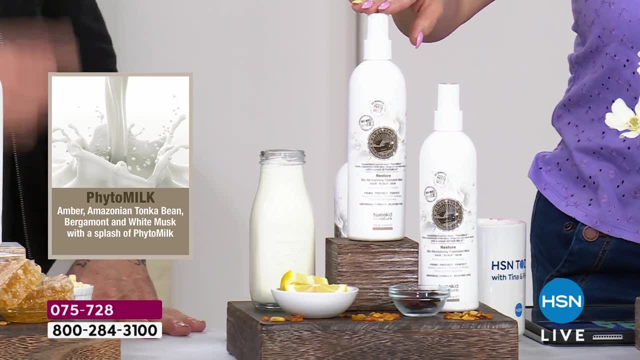 you have the milk itself, the phyto milk, so that is the only scent, it's a layering scent, so that's what's in all of them, so that's the splash. uh, performance wise, all the same, although i would say probably slightly better, because it's just yeah, it's just pure. there's, there's less to it. 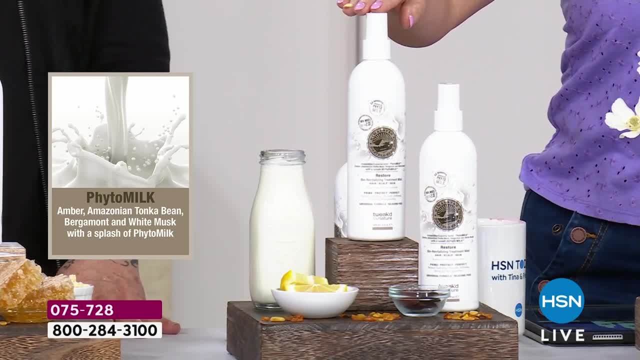 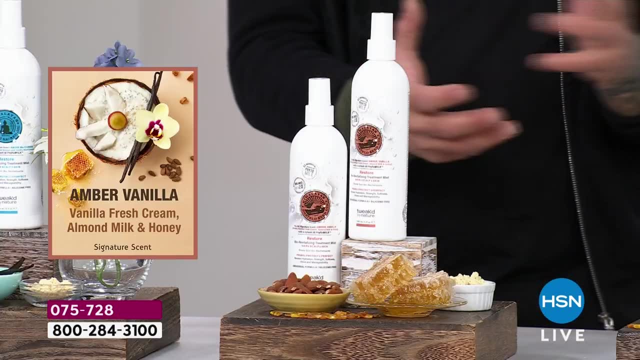 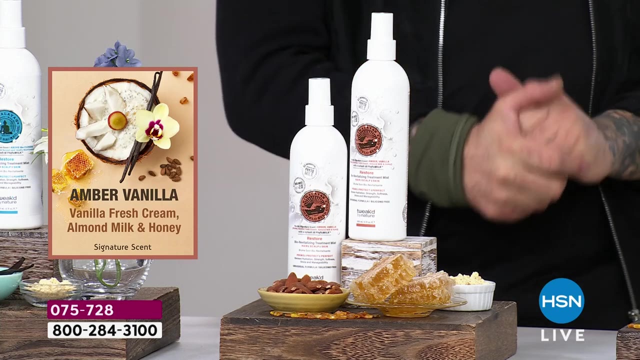 interfere, um, and it works with every scent out there and it only gets again activated as you move. so it's all done by motion. and then the amber vanilla and that, if you want to. how would you explain the scent? a creamy tonka, um, almost not baby powdery, but clean, clean, yeah, that's the. 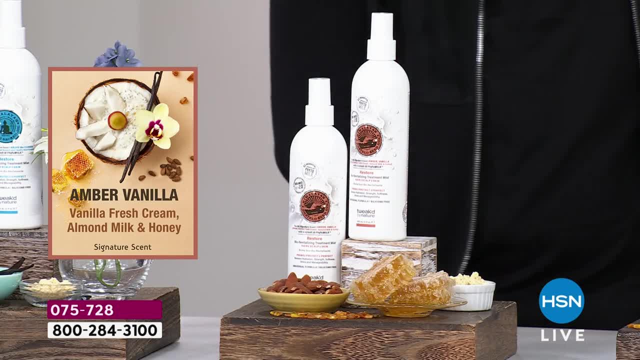 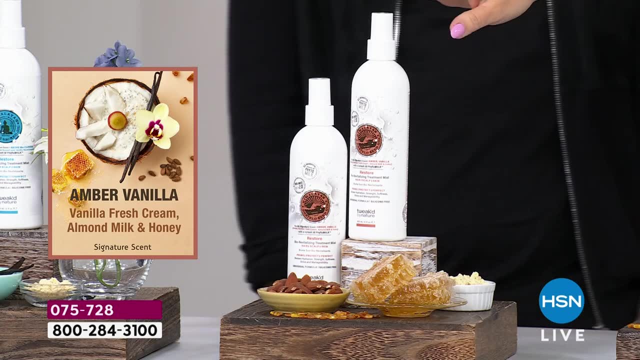 word i was using. i love it to use- beautiful. somebody had asked um online what was like the most um least fragrant or most neutral fragrance. i would say the phyto milk as well. now the amber vanilla. you're like, i'm very confused. we don't have the amber vanilla in the original. it is still that scent. it's the. 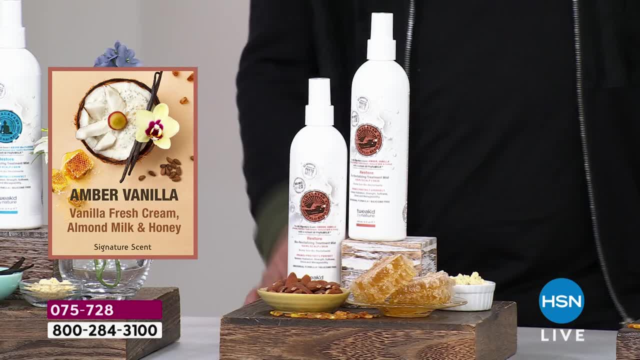 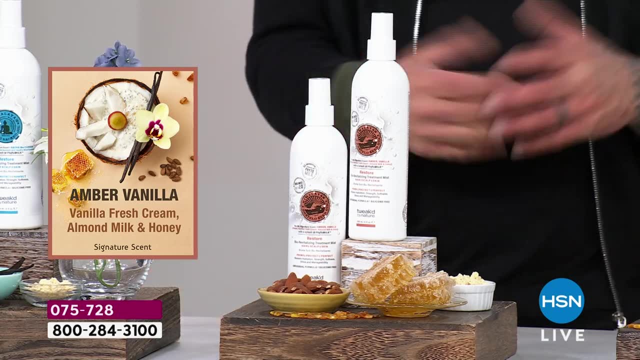 original. yeah, just that we added a splash of milk, right, so it made it creamier um more. it brought it more. to the vanilla side: yes, i love my amber vanilla, but- and i i'm always looking, can i make it better? yep, and i couldn't, up to now, have i made it better. well, yeah, i wish i could be make. 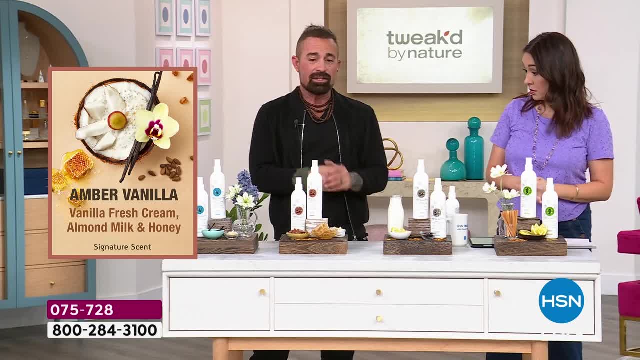 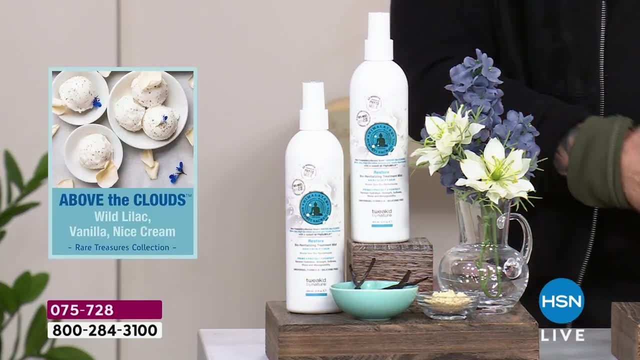 this as the amber vanilla. now that's how much i love it. yeah, the splash of milk, uh, phenomenal. and then same thing above the clouds, like it's a beautiful light lilac aroma to it, powdery again, has that clean baby powderish kind of scent to it, or in. 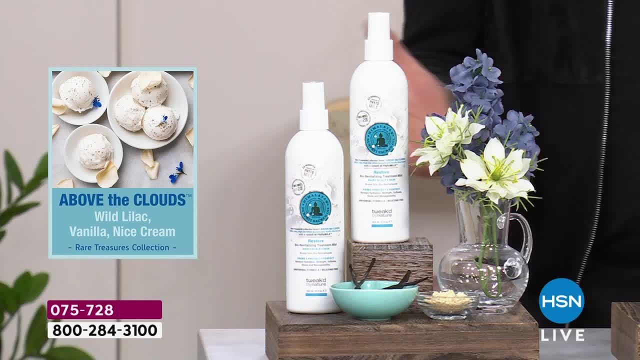 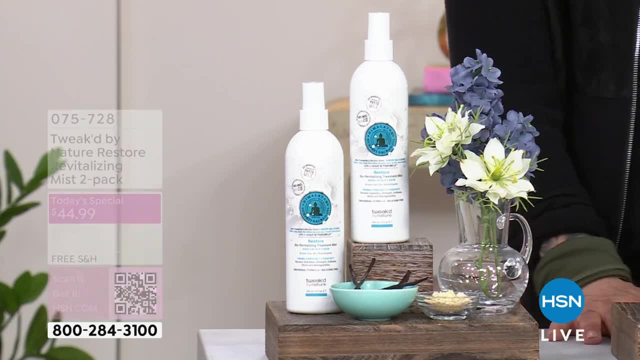 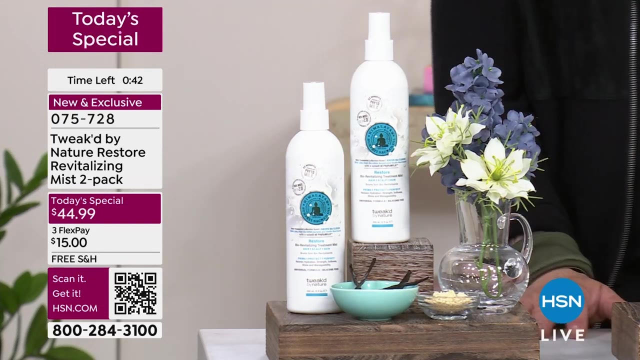 that same family. um, the, the milk that we splash now, the phyto milk. oh, if you loved above the clouds, you will love it even more now and you'll just be upset. okay, i want it in everything. yeah, give me time. but if you get into the auto delivery, you'll have this for the year. but 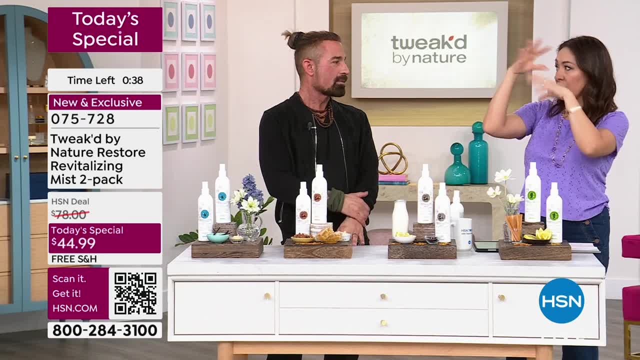 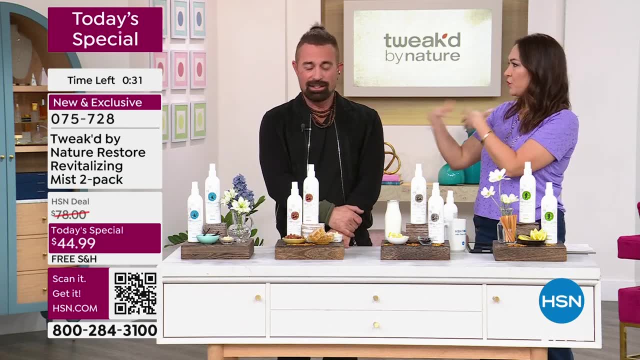 this blew my mind, i'm gonna be honest. when i saw the listing of our today special- and it gave me all the information- i thought it was a typo that it said auto ship, because there's no way 158 dollars worth. that we know comes from ingredients that are brought to you by nature. yeah, it's not. easy. and what auto ship. if you're new to shopping at hsn, you're like: what is this auto ship thing? that means you get this one, you can put it on. you know flex pay, whatever it is that you're doing, you're going to ship it to you for free when you are ready to get another shipment in. you know 90. 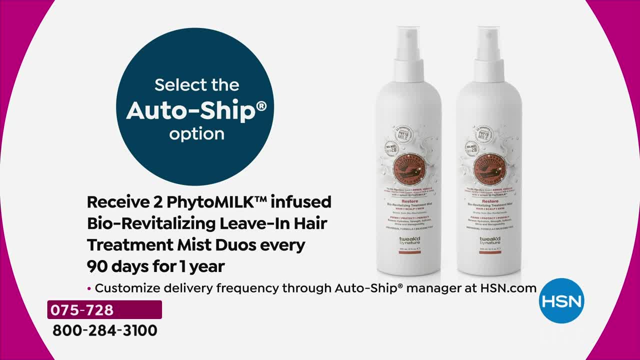 days, 60. you are in control. yeah, you're the only one another shipment you're going to be able to get in the year. you get this today's pricing. you're not doing 79 and 79 for each bottle again, but you're the only people that can do that if you don't do auto ship and you're ready for another. 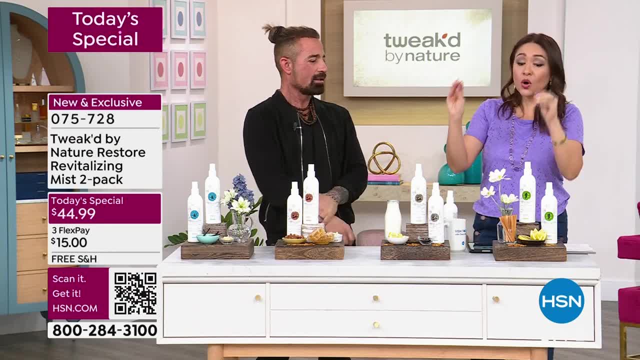 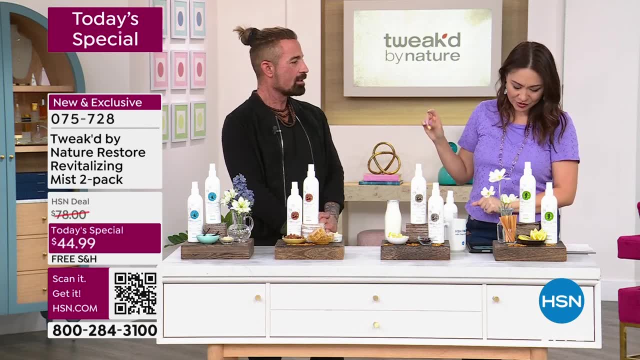 one. you're like: i got the first one as a single ship. that's not how that works, so i would do auto ship, no matter what it is that you're doing. by the way, the person that asked the question about the original and if that one's discontinued, she said: i'm so excited. um, this is the only thing that. 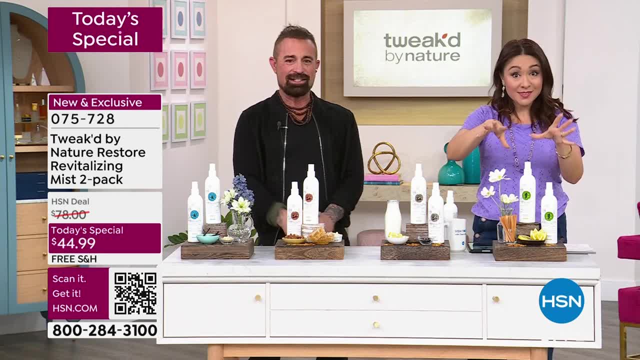 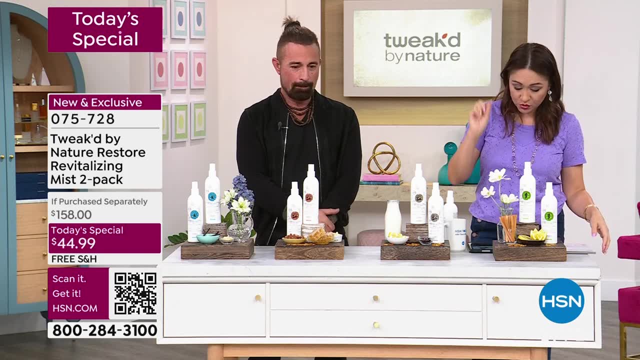 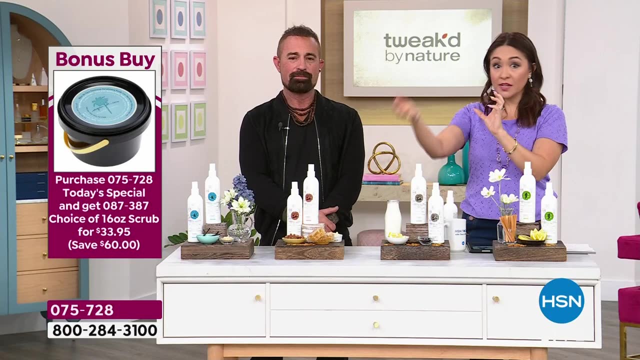 works on mine and my children's hair. so yes, this is that. take it time. you're going to be so happy. and then lenny said: how do we add the bonus when we check out? so put your today special into your cart. you're going to go put the today special in, just like. 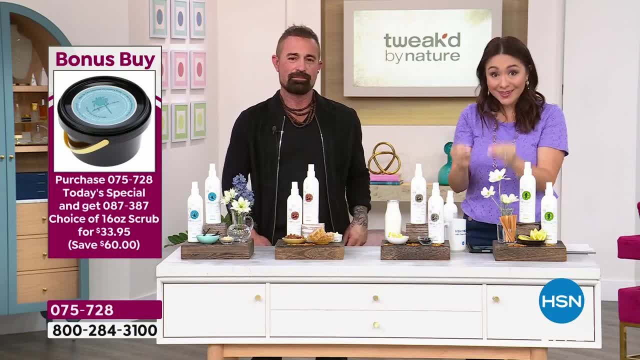 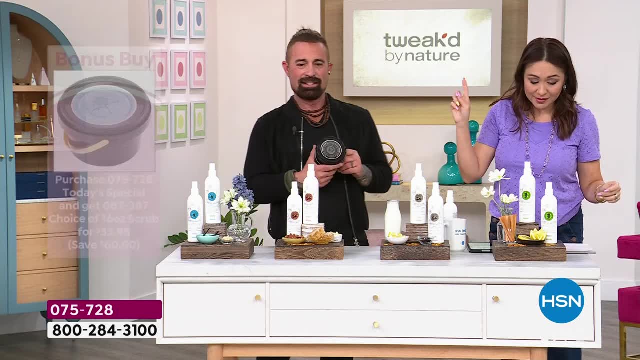 you're going to put it in like you're making a purchase. your cart will recognize that you have put the today special in. now i'll let you hold this one. dennis, you're able to get the cleansing, volumizing scrub. not for 94. it'll look like it's 94 for you. it will not. it will recognize you. 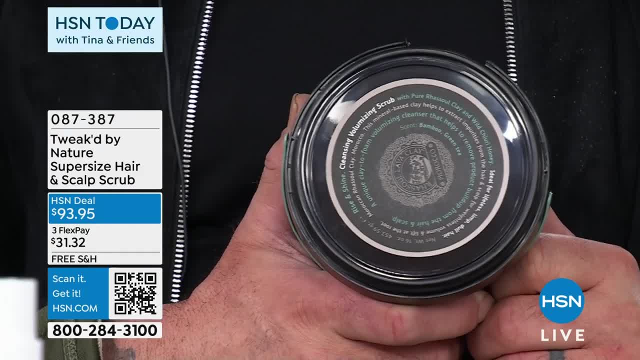 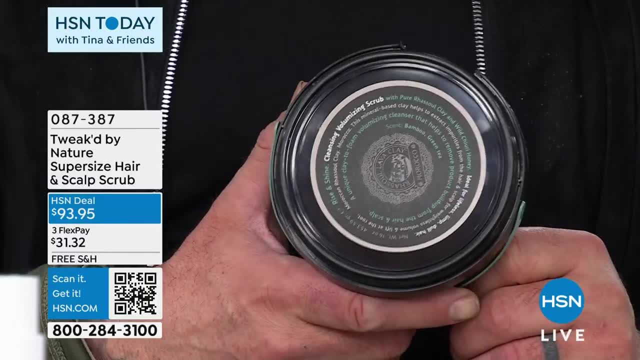 you're able to get the cleansing, volumizing scrub- not for 94, it will not. it will recognize you the today special and make it 33. yeah, i really want you to use it together and you'll see, because i don't know what's on your hair. so if you're using, you know, silicone based products. 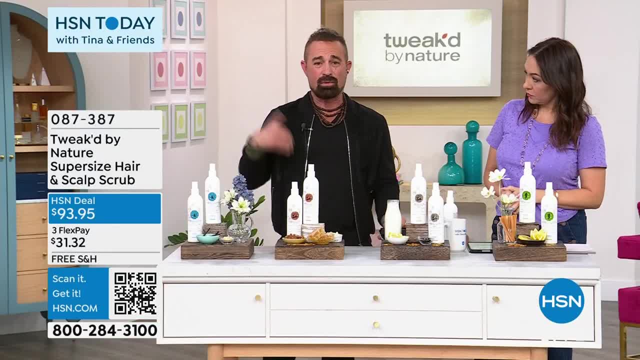 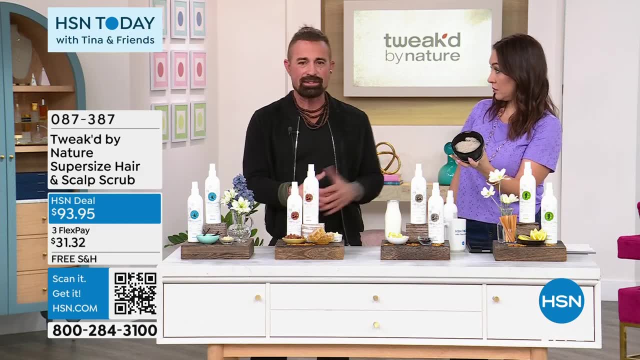 or products that are designed to really adhere to the hair. but you might not be washing them out because everybody's making their shampoos in that milder, but it doesn't allow like. you don't paint on a dirty canvas, right? so when we run the testing, it's always on clean. that'll make it, yeah, that'll. 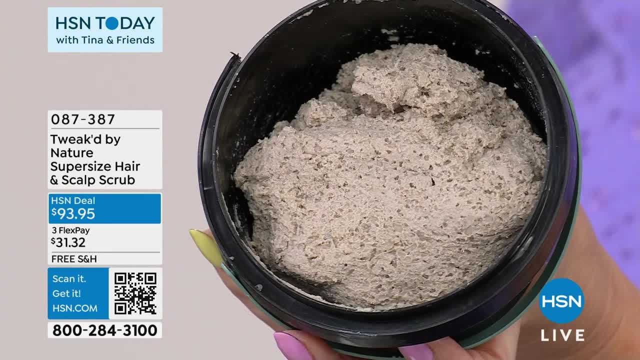 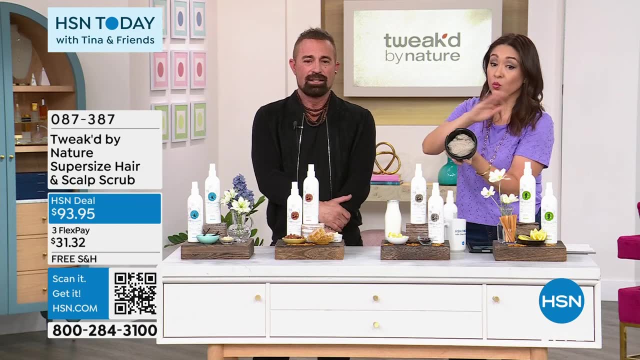 make it neutral. so that way, this, this, will get you exactly what it's been designed to do and you'll, your jaw will drop, you will see the hair that you're seeing. that's what you got to be getting. it's not 94 for you. i don't don't even look at the screen because that doesn't apply to you. 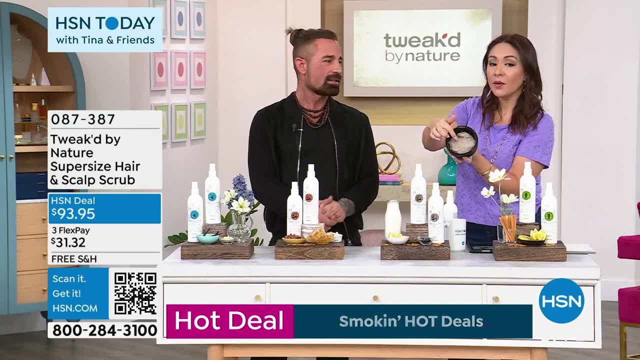 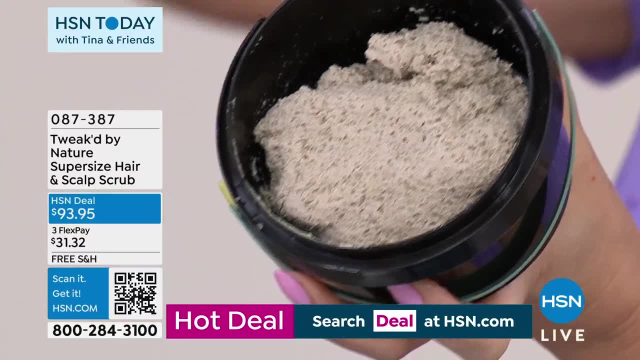 it's 33, if you're getting the today special and, by the way, i want to get ahead of it and i've asked, i've told everybody that i've given this to. i said you take the scrub because it's like mud, it looks like a big clay. i said you add it with the water and then it'll get splashed, the water, but the more 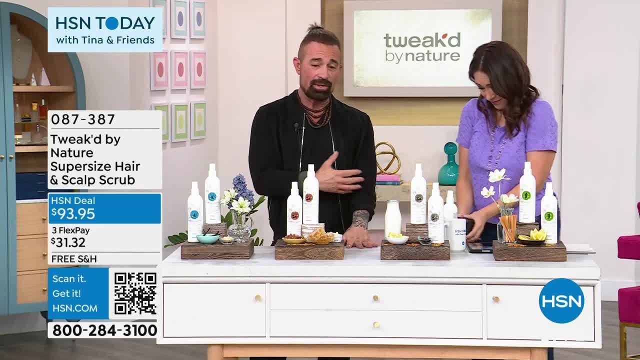 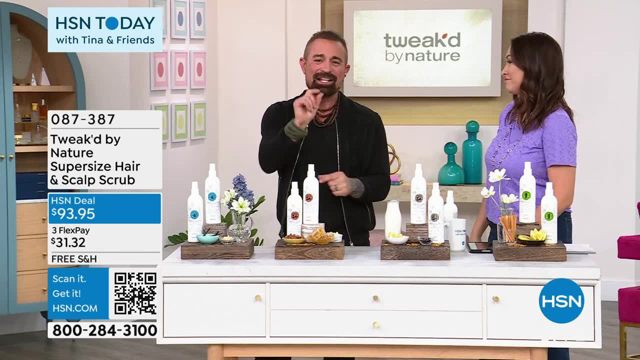 you use of that less lather, because it's potent. there's no water in it, unless i picked up the whole thing. yeah, made a ball out of it, just it's clay in a way, so that rhymes. a little bit water, lots of water, so water's free. we will keep seeing dennis in this outfit because his luggage, yeah, when it changes. 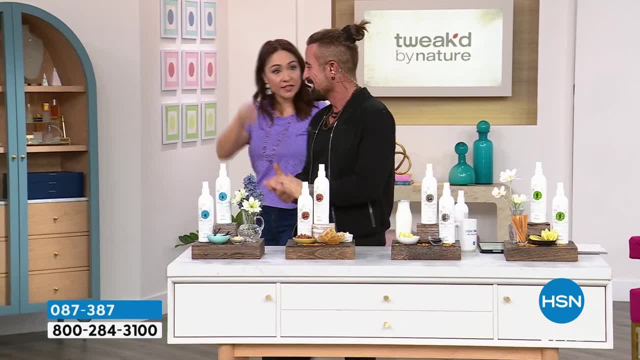 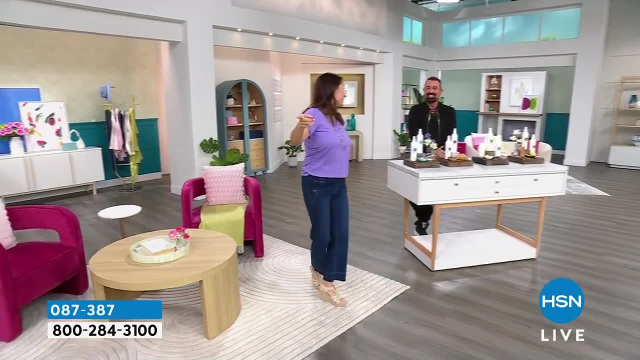 and you know. okay, you got his luggage. are you up next to valerie and wake up? beautiful, yeah, we'll see another presentation. they told me just camp out, so just hang out here. yeah, watch this, dennis, you're gonna love this. okay, cool, he's like: why is eddie in a robe? whipped cream challenge. 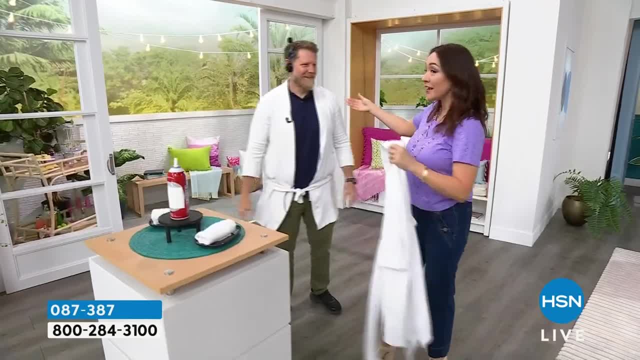 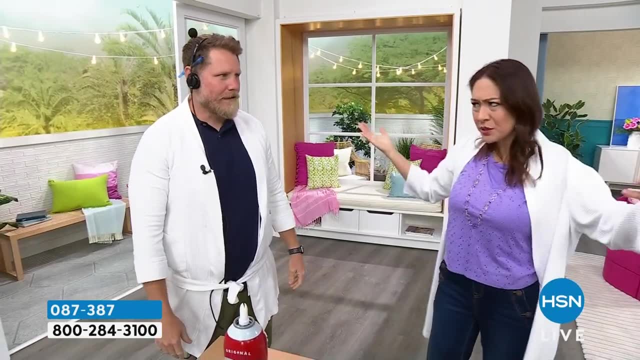 in a tiny robe. it's watch. this is amazing. okay, eddie, who we all know i love- he's one of our producers- uh, decided. i said i practiced with my husband last night in our kitchen and for some reason, he was really good at this. so i don't know if like boys get pulled to the side in fourth grade to learn how to do this game. 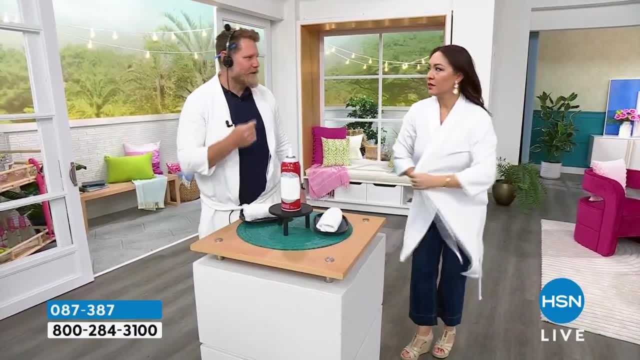 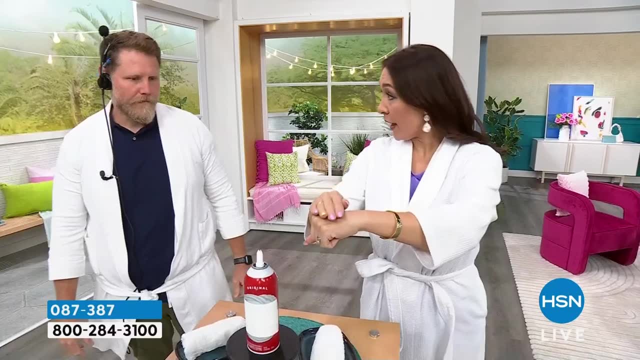 i never really threw a lot of this stuff up. i did it once with an m? m and i almost chipped my tooth. oh then, no, maybe you won't be great. i might not be great. okay, whipped cream challenge. you put the whipped cream on the back of your hand copy, then you flick the whipped cream into the air. 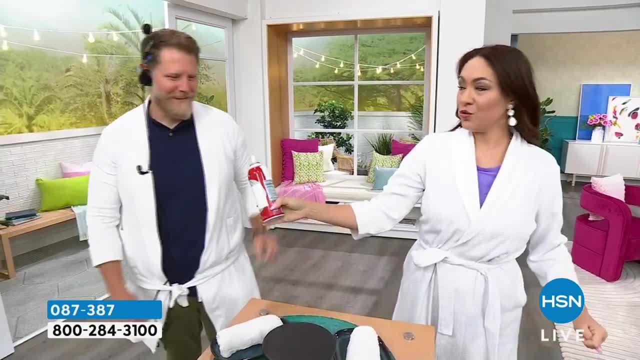 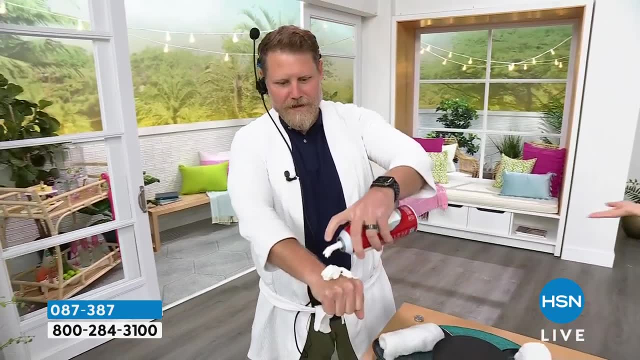 and then try to catch the whipped cream with your mouth. it's going to be free fun. you do first. okay, I go first. by the way, no pressure, I did it yesterday, yeah, and you also said you're practicing last night. I don't know if I like that all. 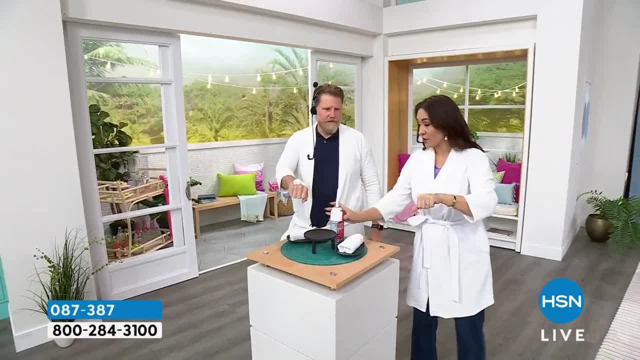 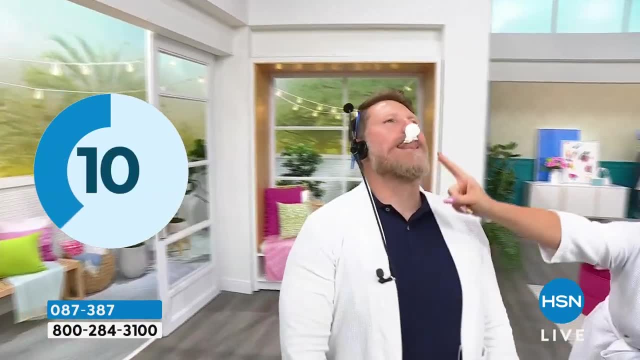 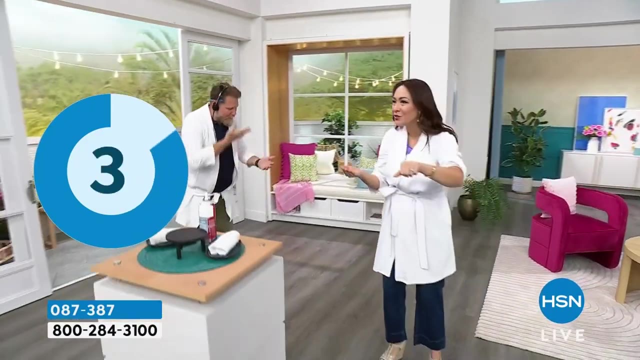 right, we're gonna have Eddie. you go first, so I don't want to embarrass you by doing it right. yep, do we count that? do we count that? does that count? that's good stuff right there. oh man, I told you why are guys so good at this game? this is my. 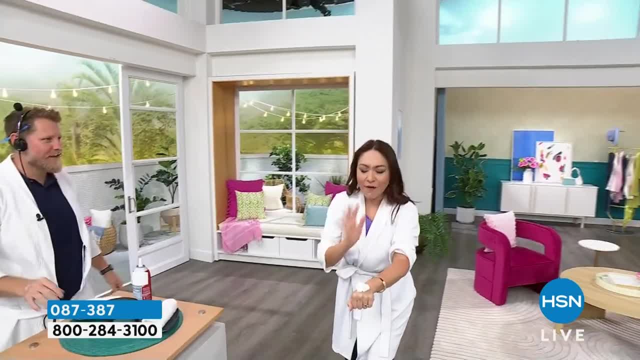 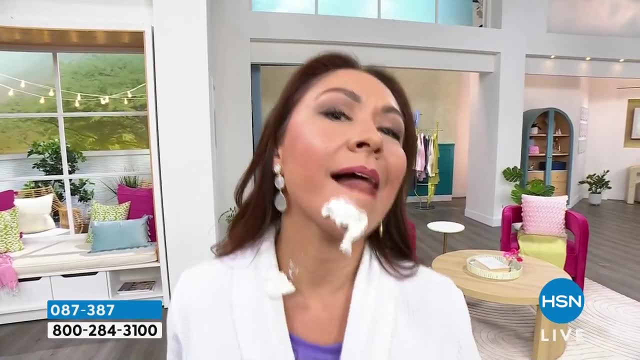 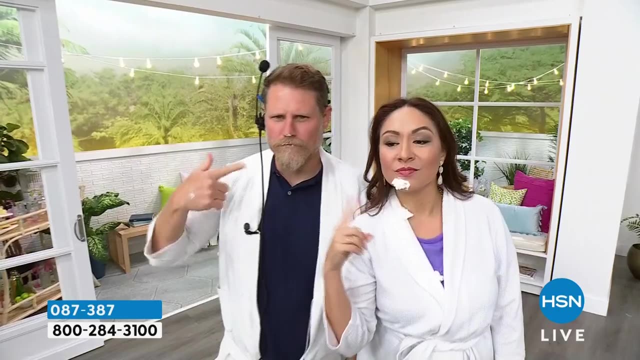 okay, my husband tried to give me pointers last night, ready. now I feel too much pressure. you were saying you went too high, so I think you gotta count that which one of us was closer. my mine's like mostly: oh no, it's still there. Eddie wins: yeah, his was on his lip, yeah it. 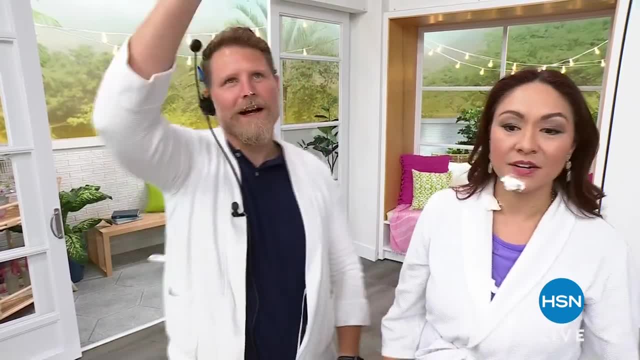 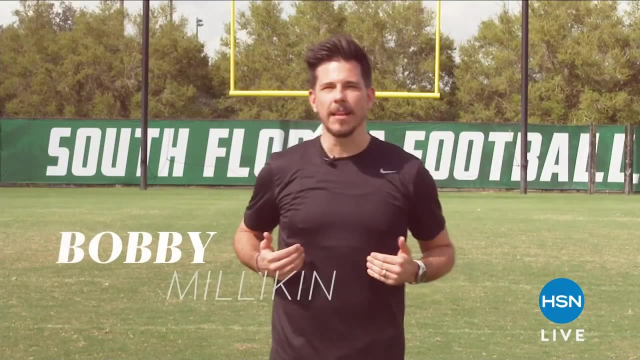 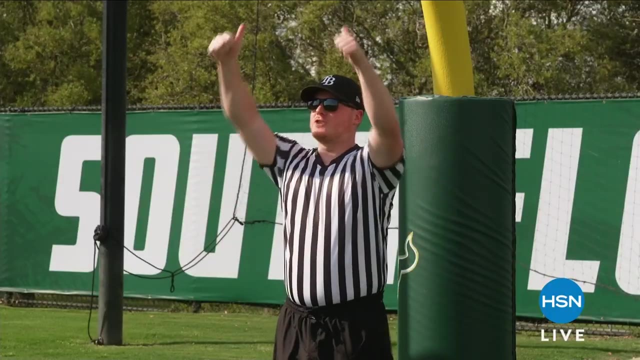 was upper lip and nose. I tried to. just my husband said you went too high, went too high. he said, direct it the champion and friend of the Tina and friend show. and this is a 50-yard field goal. Harrison, are you ready? let's do it all. right, let me walk this off. 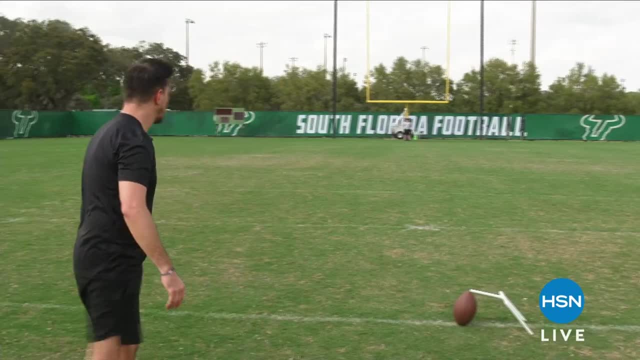 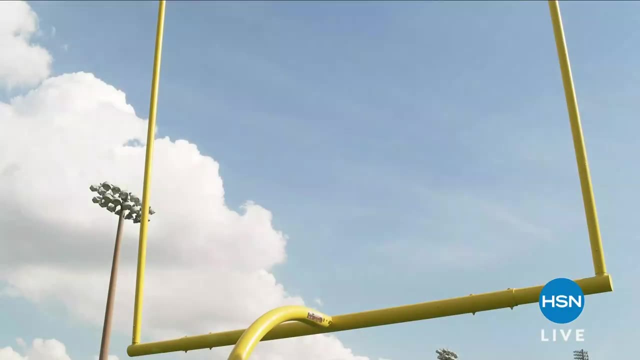 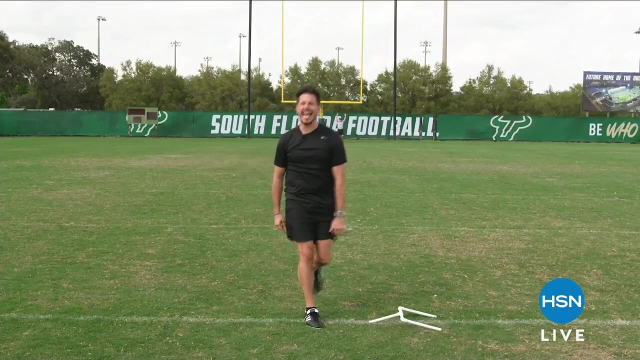 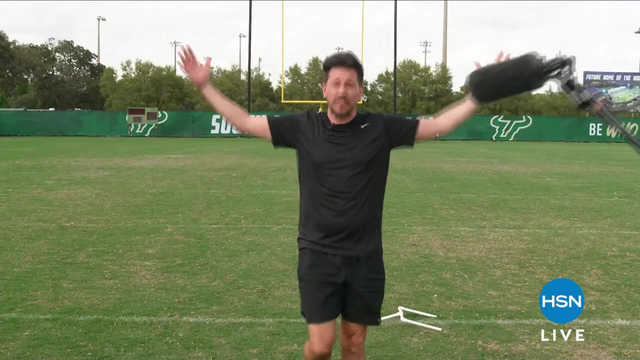 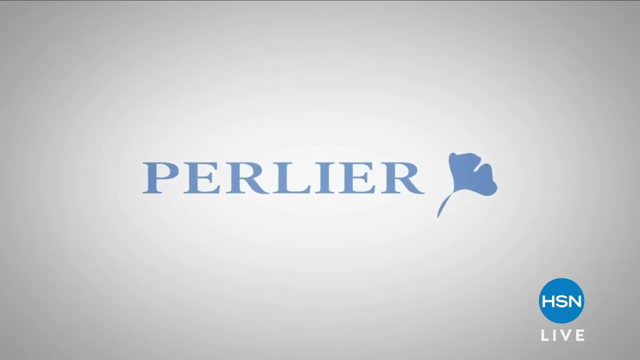 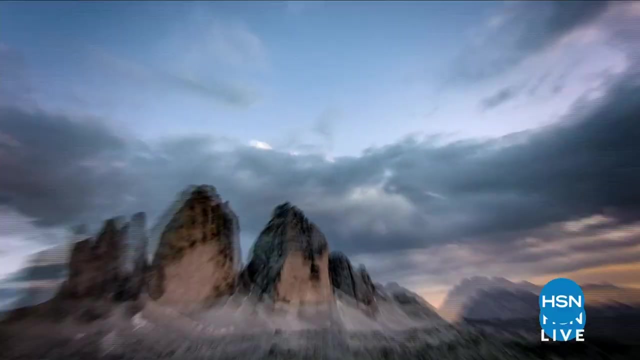 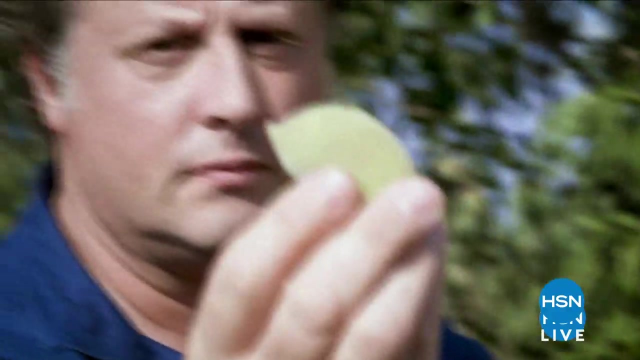 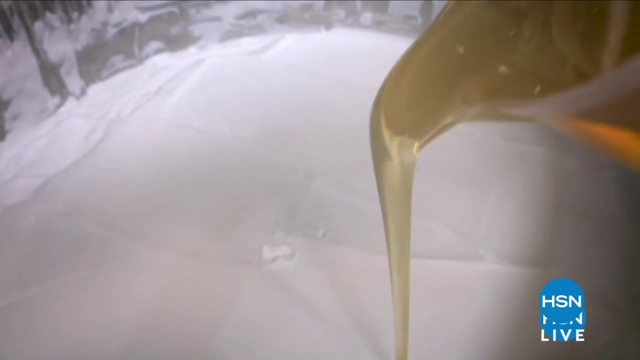 looking good. here's how you do it: boom first, take what I tell you. boom, baby, literally boom, what's up. that was Bobby Milligan 50-yard field goal first. take. no lie, Tina, what'd you think? yeah, you, yeah, you, what's up? you, you, you. 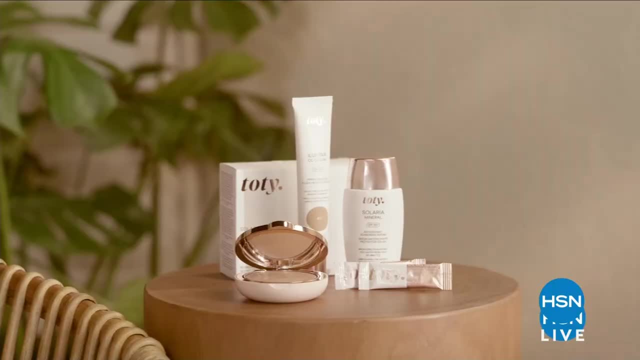 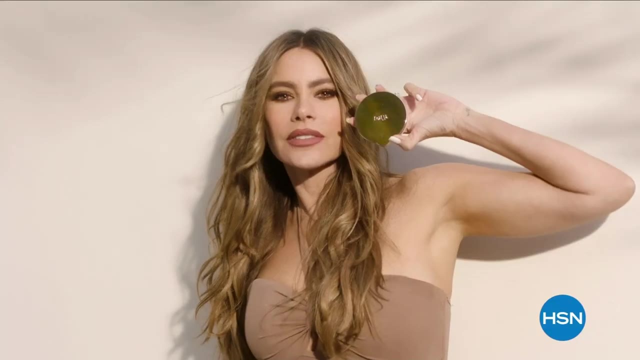 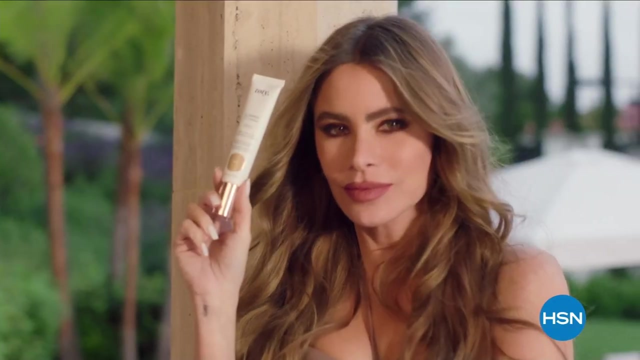 I am Sofia Vergara and I am so excited to introduce you to Toti, my new range of advanced sun care. Made to protect your skin from photo aging and visible signs of sun damage, Toti is designed to enhance your belleza. 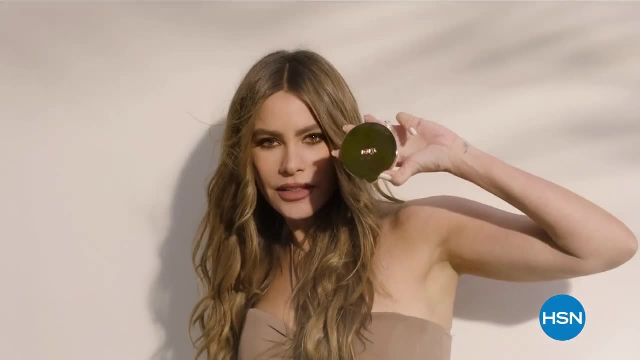 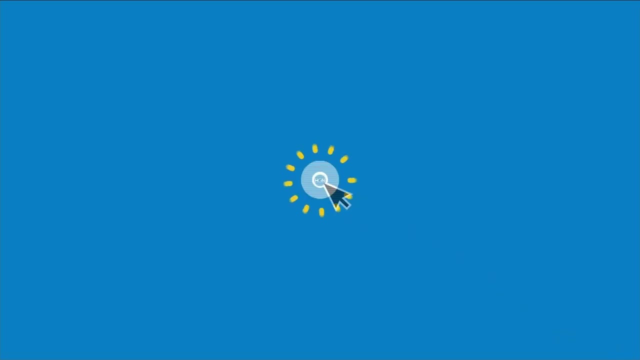 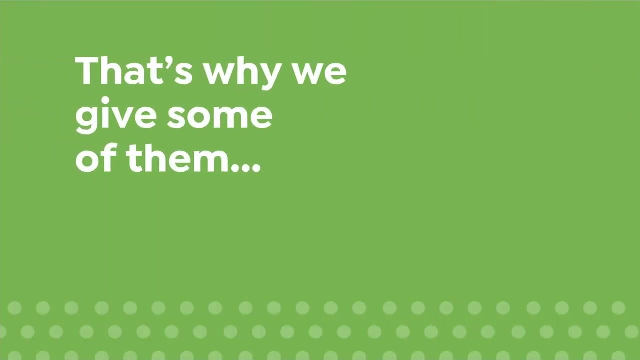 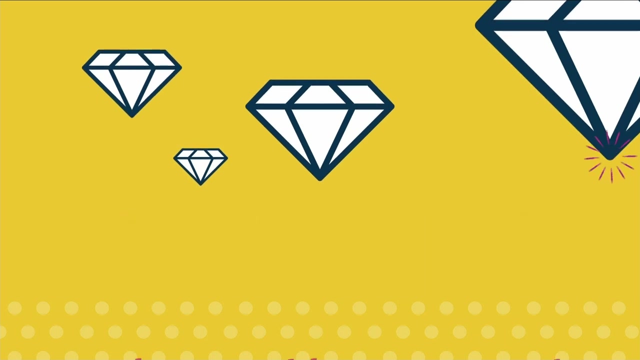 Become your most beautiful you with Toti. Watch Toti by Sofia Vergara, Only on HSN. We love our gemstones to be beautiful, colorful and durable. That's why we give some of them a little more love. Enhancements may require special care and may not be permanent, while others may last a lifetime. 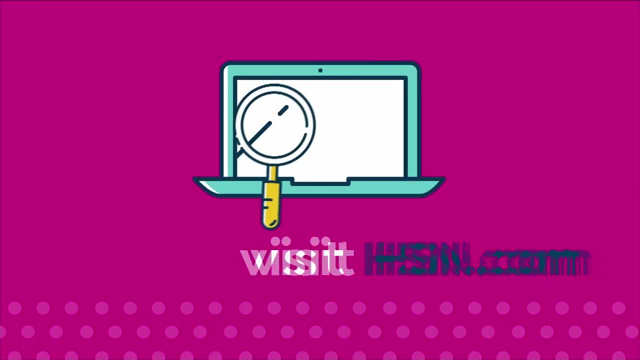 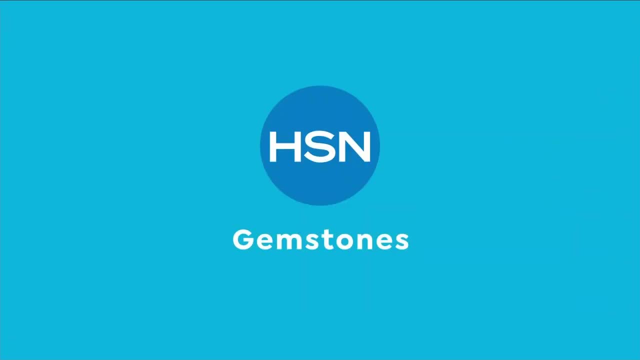 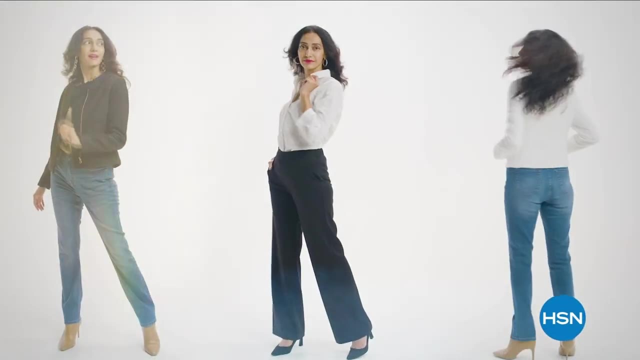 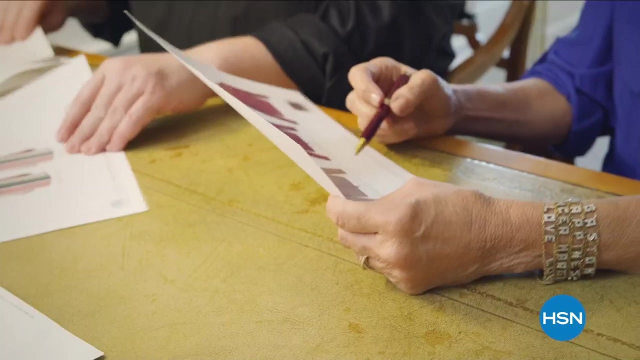 For more information, visit hsncom and search gemstone care to see our gemstone enhancement chart. I am beyond thrilled to partner with a company like HSN. It's a true honor to share my closet. I surround myself with the most talented team possible. 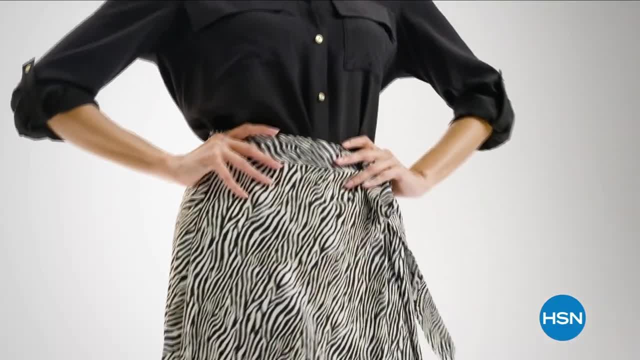 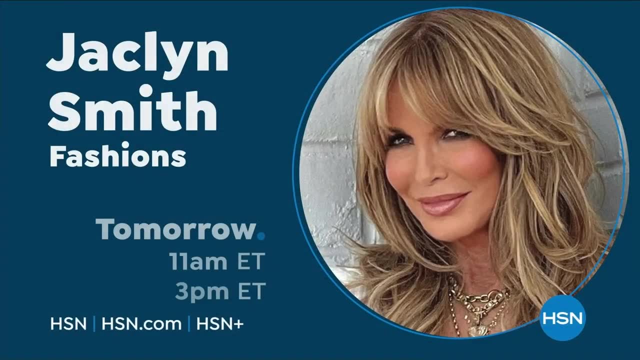 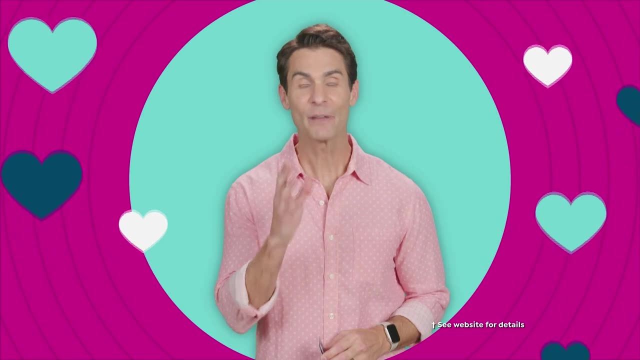 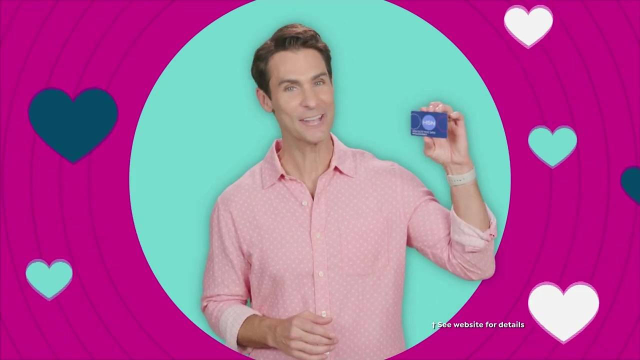 Design essential pieces that are stylish yet comfortable. There should never be an expiration date on looking and feeling beautiful. You're going to love this. Get more of what you're shopping for now. It's bonus by Wednesday and be sure to check out VIP Thursday to cash in on exclusive HSN card offers. 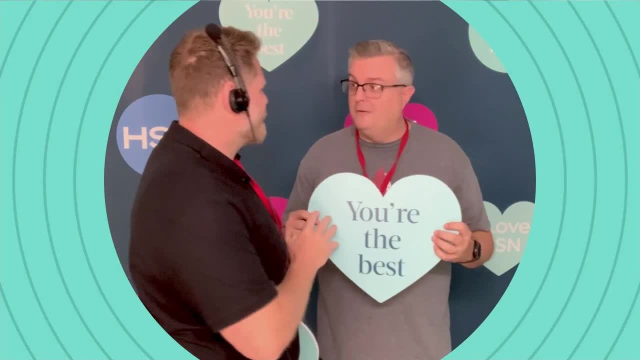 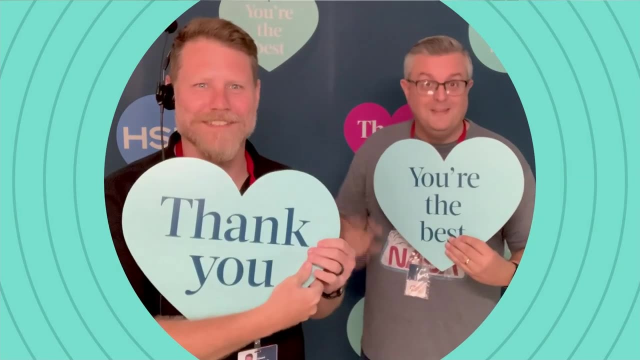 Hi, I'm Jared and I'd just like to Hey. you know what, Jared? You're the best. No, Eddie, They're the best, They are the best. Thank you, That's backwards, Thank you, Thank you. 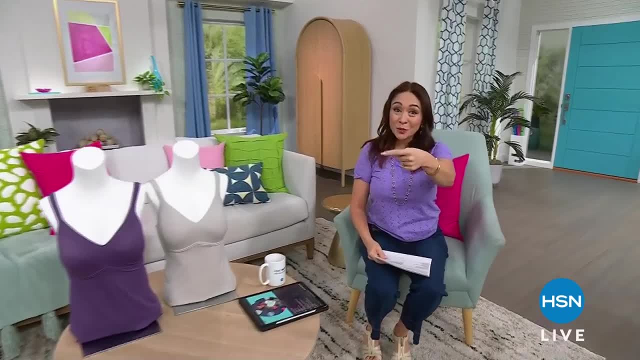 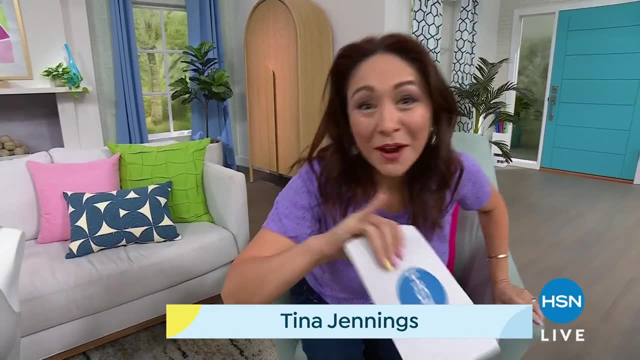 That was Jared, That's who's producing The world-famous Jared, And that's Eddie, who just played the game with me. That's the crew I have- the best crew in the planet, By the way. I want to do one more kind of like: get your eye on three additional products. 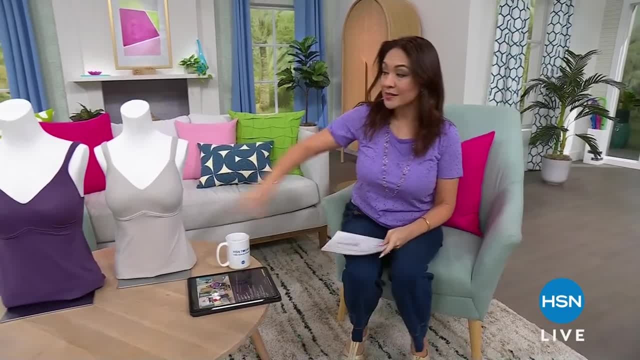 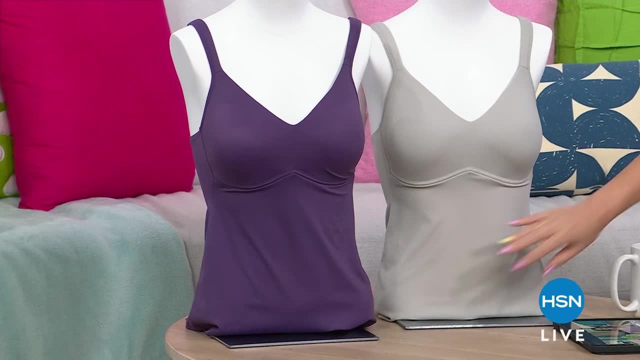 We're going to call this a little mini three-in-three, because these are also on a great price. This one we launched at the beginning of the week and it has been screaming. It's from Rhonda Shear. It is your new kind of tank, cami, but it's a built-in. 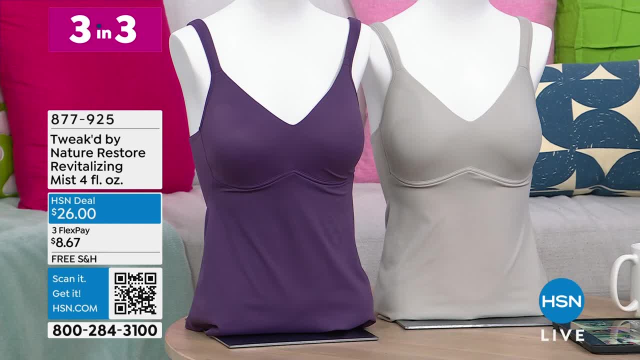 It's a molded cup to this, so you do not have to wear a bra with your tank or your cami, so you don't have, like you know, four straps and you know running at the top of this. 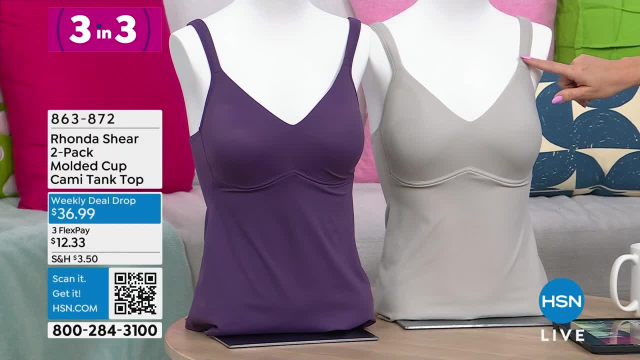 It is adjustable straps and it's actually padded here in the front. These are extra small through 3X. These are $78 for the two-pack, but as a weekly deal drop it's $36.99.. This is the option we're calling gray with wine, berry purple. 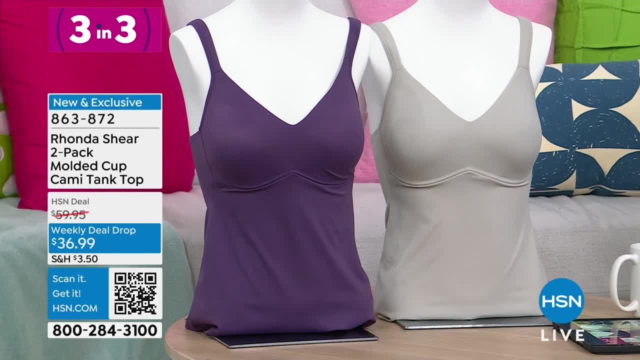 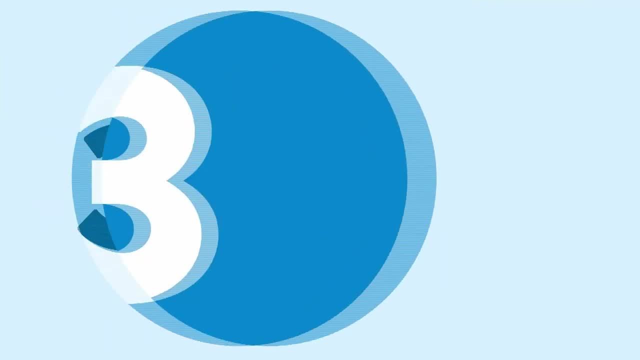 We also have a black and a white combo and a beige and a rose combo, But grabbing these, it's got a little smoothing control. that's in there as well. So this is your tank slash, cami. Let me put something you can layer on top. 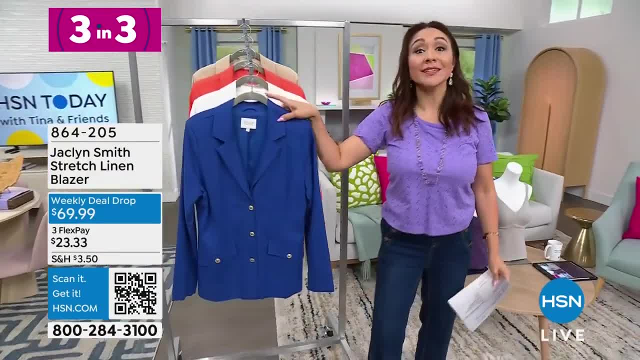 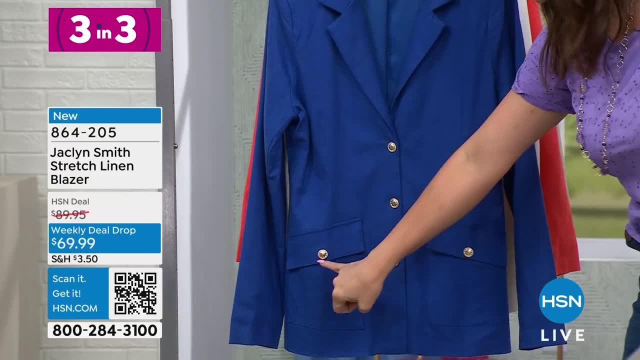 See that transition Layer on top of it From Jacqueline Smith. it is a gorgeous, beautiful linen blazer. Look at the button details that are on here. You get the little button detail on the flat pockets in the front. It's 27 inches in the length. 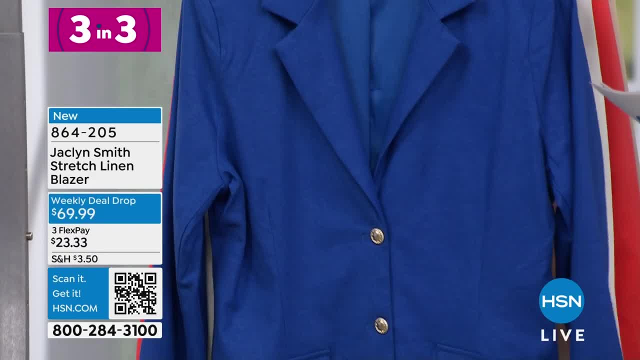 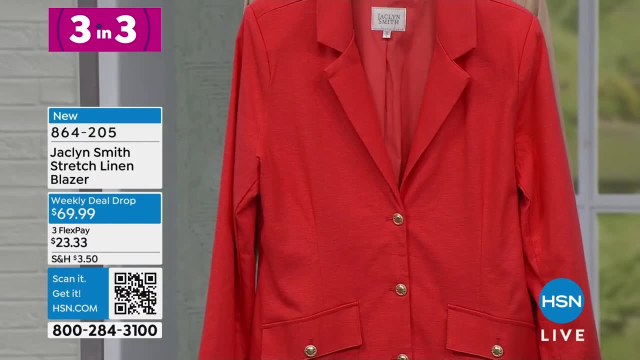 This is actually machine-washed, tumble dry, extra small, through 3X. This is what we're calling the Beaucoup Blue, Beautiful, bright white, And this one's called Ember Glow. So unique, so different, And we have in what we're calling Oxford Tan. 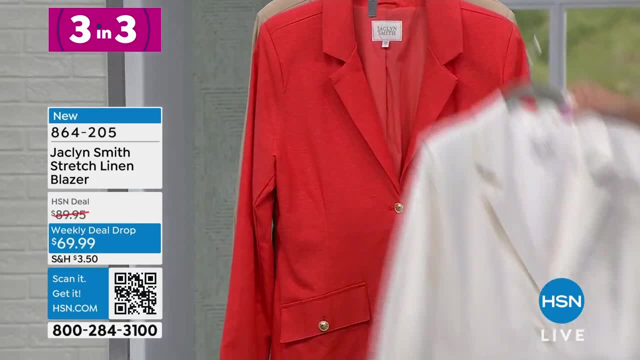 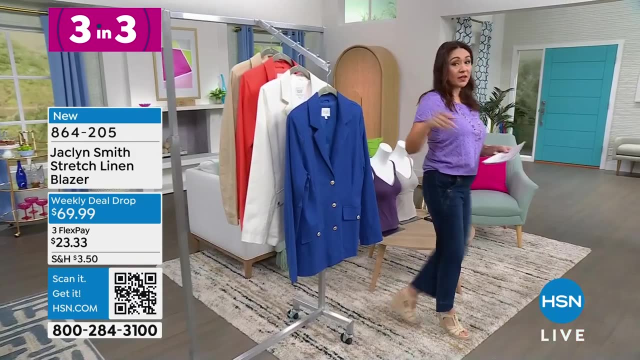 This is a $90 linen blazer for $69.99, but it does have about 3% spandex in there, so you get that stretch as well. So I have a blazer. I have the cami to go under the blazer. 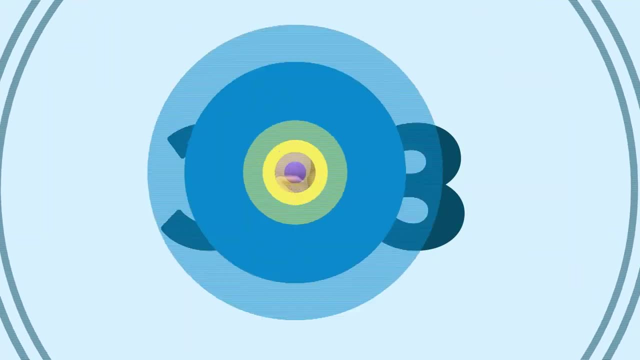 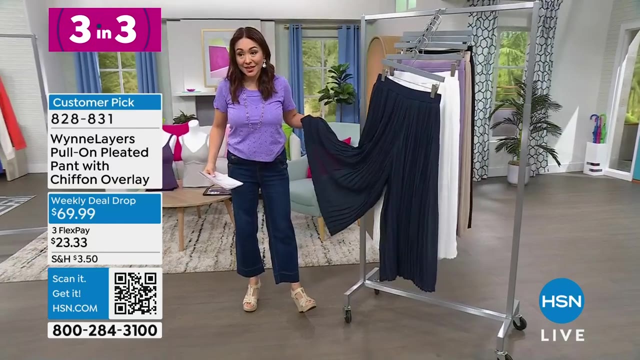 We're naked down here. Let's get some bottoms. From Marla Wynn this reads like a skirt right, It looks like this. really cute, like chiffon skirt. It's pants, Isn't that crazy? So there's actually underneath here like a lined pair of like super soft. 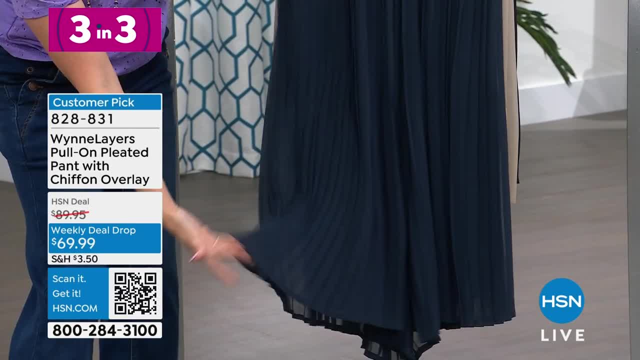 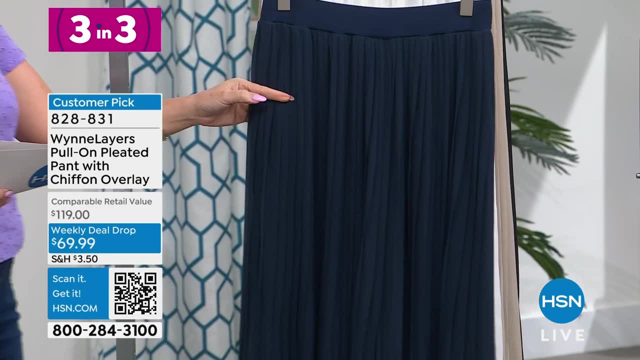 almost like pajama: bottom pants and then a chiffon layer on top, So it's like wearing a skirt, but having your favorite pair of pants on. These are a customer pick at $119.. Weekly deal drop at $69.99. 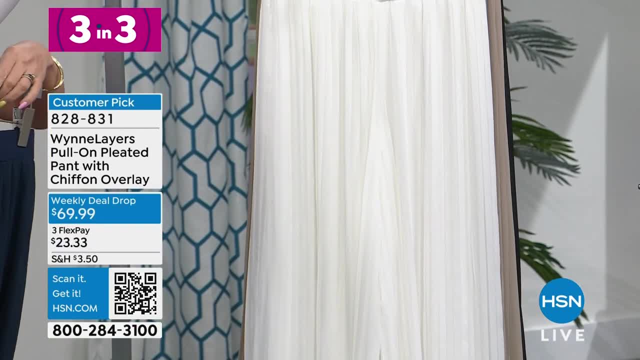 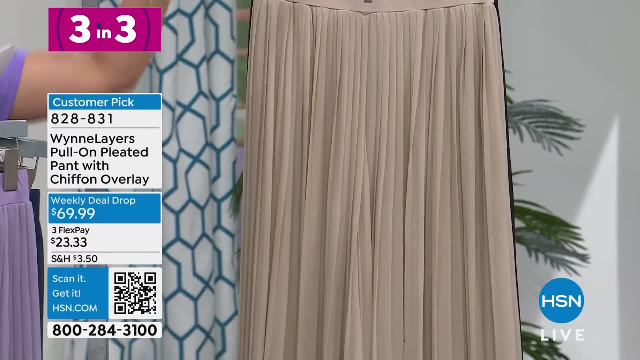 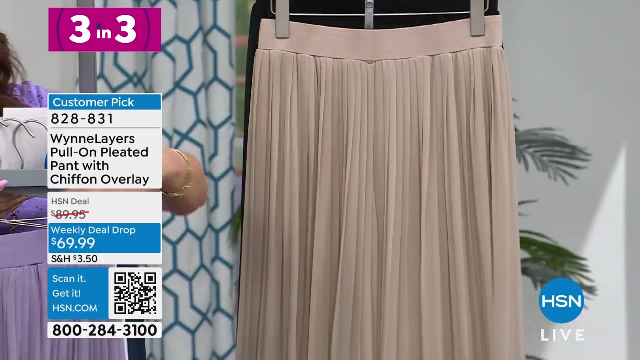 This is called Midnight Blue. There it is in Cloud, which is our lightest color. This is called Dusk, a beautiful dusk lilac. We also have it in Sand and I wore it earlier this week in the black. It's average length at $25,, petite at $21.50, and then extra, extra small through $3X. 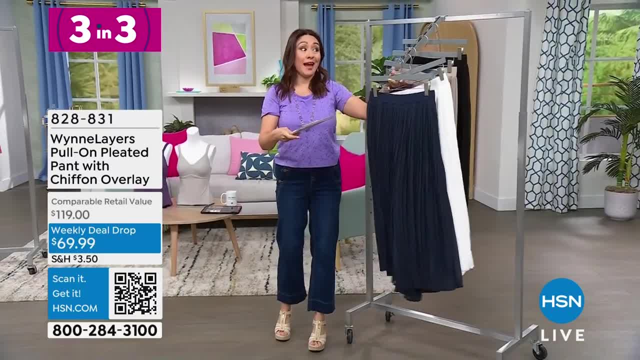 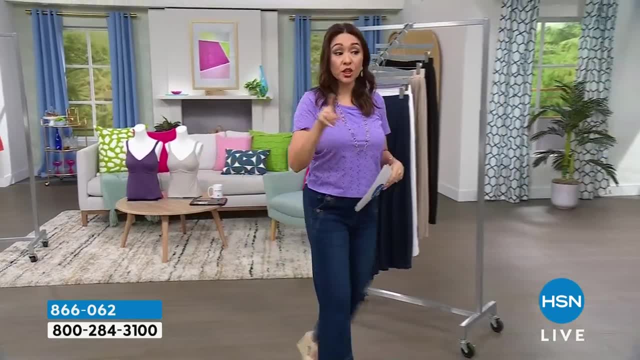 Read those reviews. Everybody talked about how much they love it. I just gave you a complete outfit. I didn't even mean to do that, but that kind of all worked out Okay. I gave you all these weekly deal drops. Let me give you a launch of something. 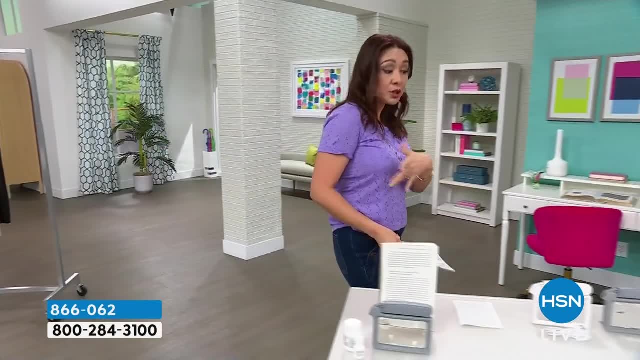 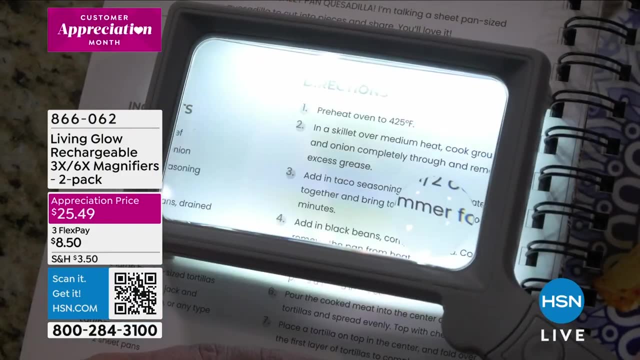 And I said at the beginning, a lot of these items would be great options for, maybe, Mother's Day. This is actually from Living Glow. These are magnifiers and you're going to get two. You can magnify by three times. You can magnify by six times for those teeny tiny things that you need to read. 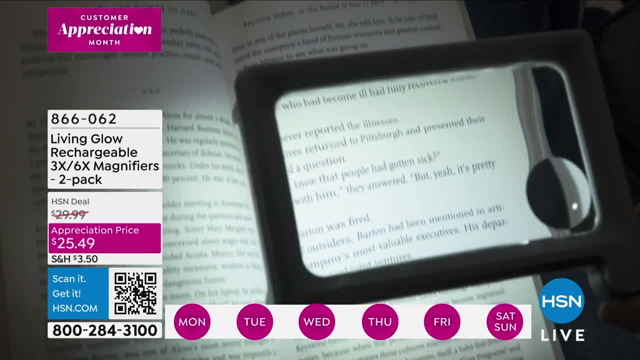 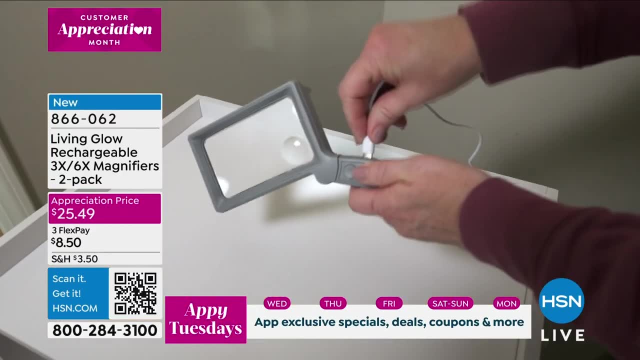 And it's actually going to have light: 20 LED lights, three brightness levels. It is all going to be in daytime lighting. It folds up, It's got a little handle, It's rechargeable, so no batteries, And you get up to 10 hours of light on one single charge. 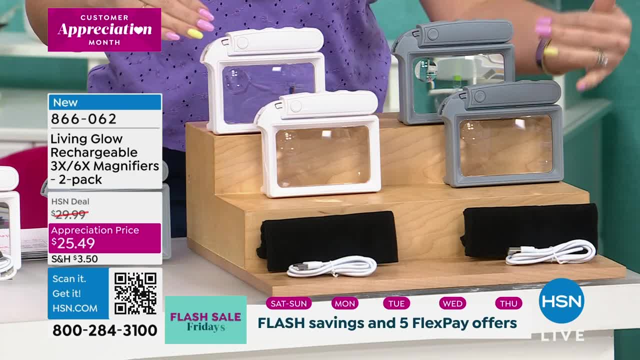 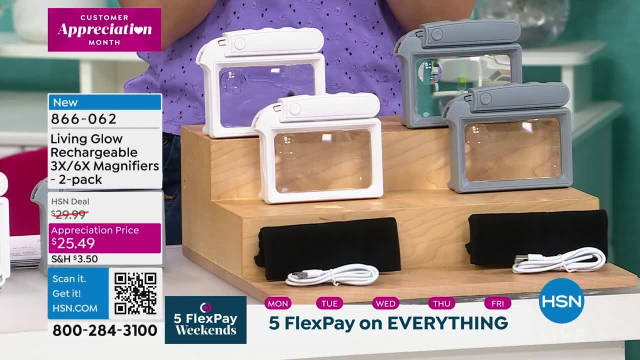 So you're going to pick. do you want it in the white or do you want the two-pack in the gray? They're going to come with the cords to charge them up and little pouches On appreciation pricing because it's a launch: it's $25.49.. 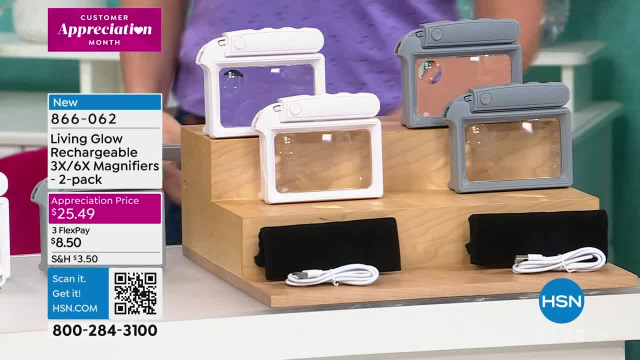 Julie Truster is going to show us. I walked in and I said, Julie, is this really the launch? And she said yes, And then she goes: these are really good. They are really good, They're made out of all glass. 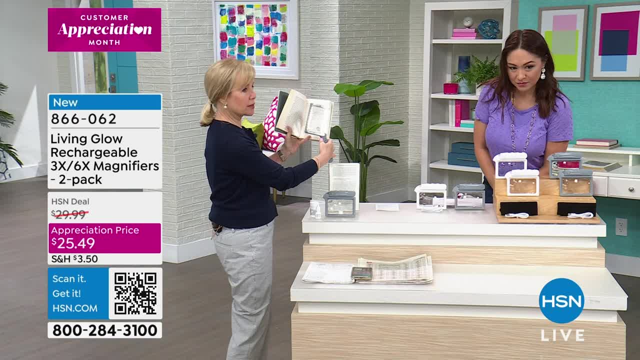 And I want to show you too. Okay, so the LED lights are on the back. It sort of looks like a mirror. Oh, it does kind of look like a mirror. Yeah, now I have it backwards. I'm just showing you the light. 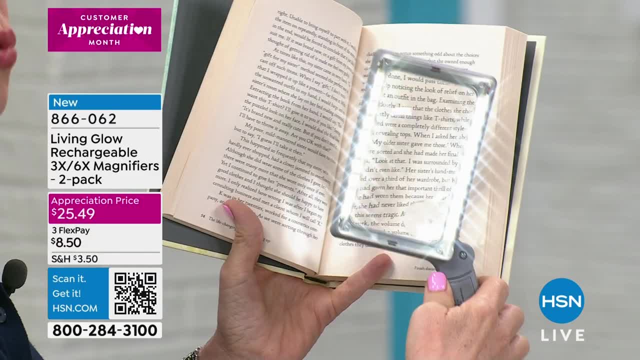 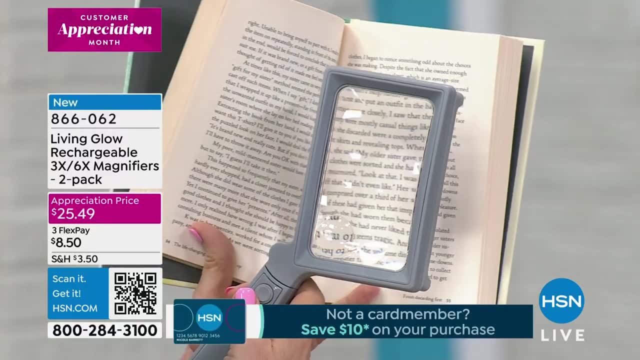 There, we go Off, And then you can turn the LED lights on. There's 20 of them, And then this has that three times magnification. So hold on, Let me turn. Okay, let's see if we can do a good shot of the studio. 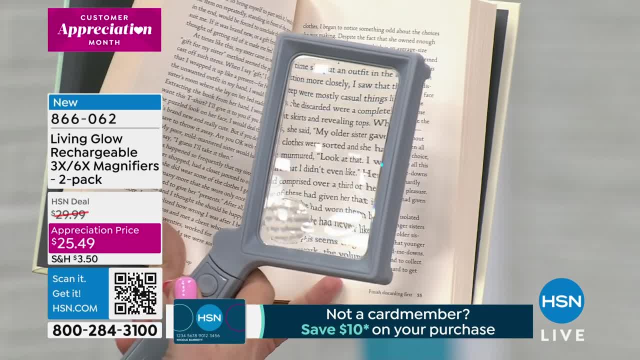 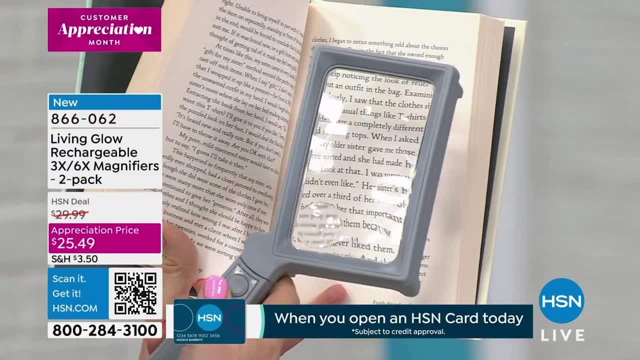 And the great thing about it is, you can turn it this way And then the further you pull it out, the bigger that it gets, Or you can do it this way. So, depending on what you're reading, Are you able to see? 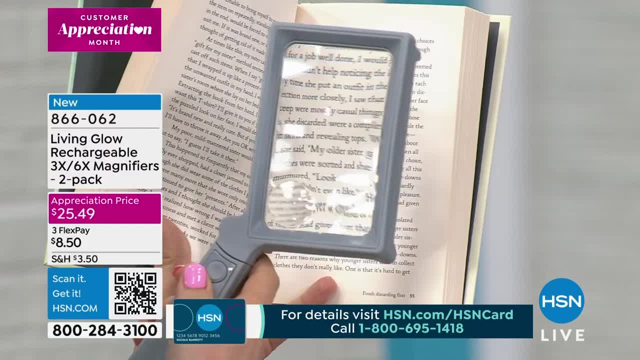 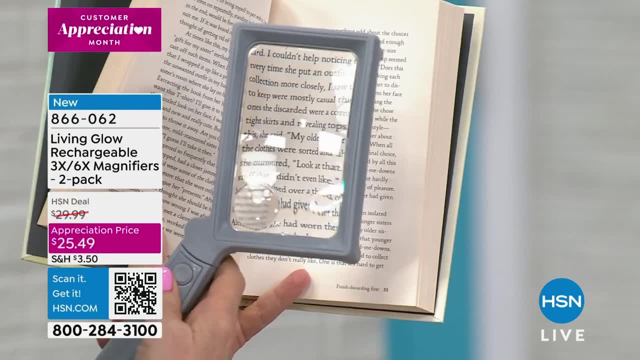 Yeah, Okay, perfect. So yeah, so up close, Or you can pull it out, You can read. You can read those medicine bottles. Maybe it's a newspaper, a magazine, just a book. Maybe it's your phone. 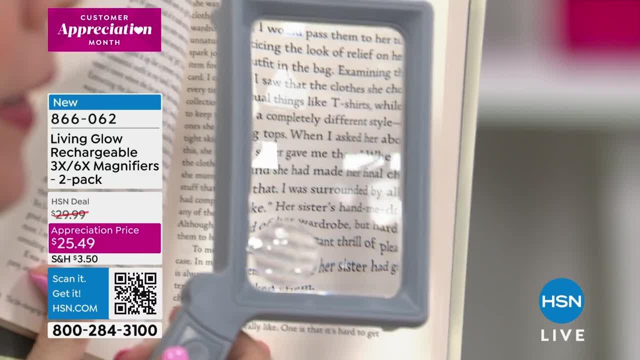 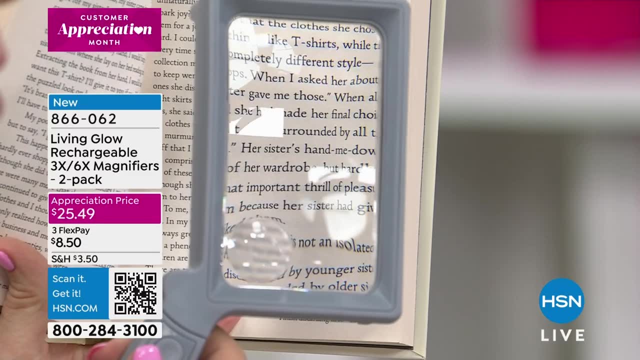 And you can see how much better that it looks. Okay, hold on, There we go. Look at how big that looks. Yes, Look at how big, even if it's just your phone. Now, if you see those little thingies on there. 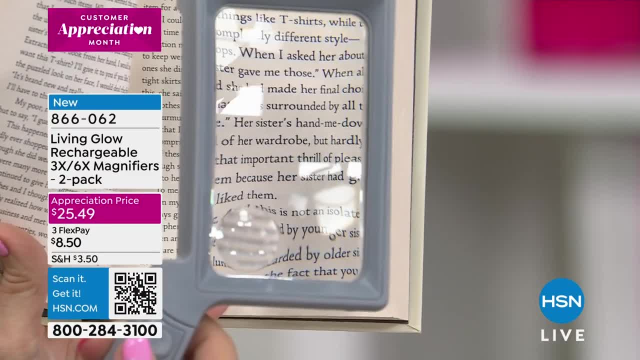 the light in the HSN studio bounces off of here. Yeah, That doesn't happen at your house. This is an anti-glare, I mean, unless you, You live in a place with 20 million lights in there, Exactly. 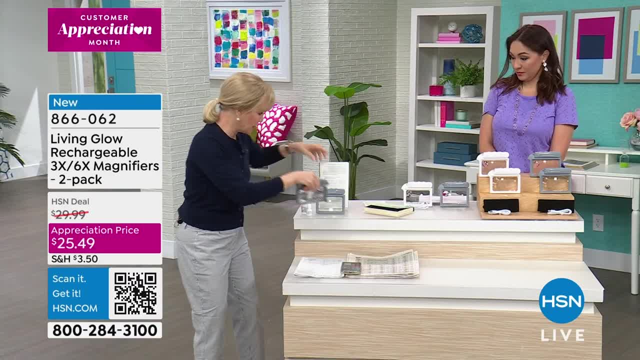 This place. Okay. so look at this. So it folds up like this. It even has a little stand so you can stand it. I put it on the desk. in our little kitchen area We've got one of those little tiny desk areas. 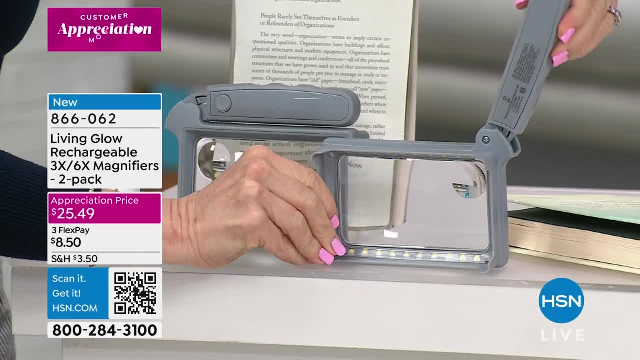 So you can stand it up like this, But this is the one that has a handle, And I'm not even kidding you. If you go to the dermatologist- Yeah, They have something exactly like this, where they look at all your- Oh really. 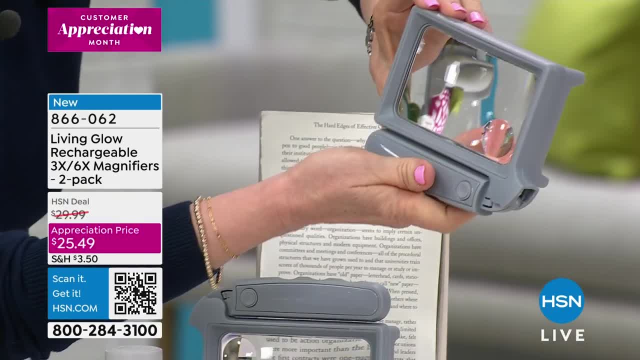 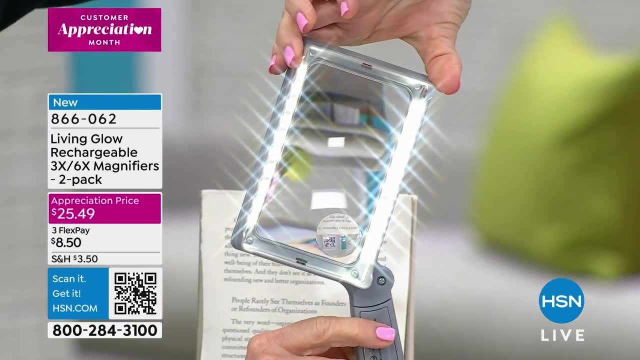 Your spots and your moles. And, yes, they have the exact same thing. So it folds up, Okay, It stands up, folds up, Okay, Okay, Okay, Okay, Okay, Okay, Okay, And you pop it open and there's one button and that turns on those 20 LED lights. 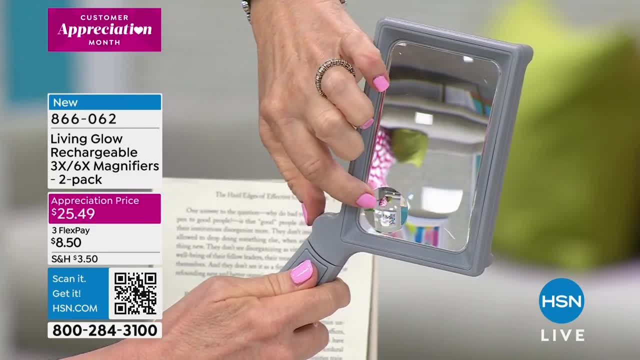 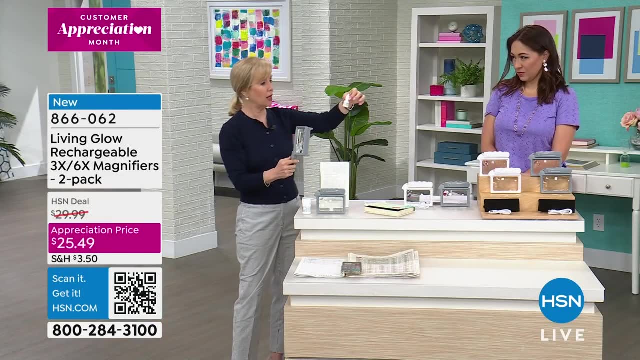 It's a three times magnification And then that little circle. there this is the six times magnification. So I'm going to take the smallest little thing that we have. This was a little eyedropper for my dog And I put it in his eyes the other day. 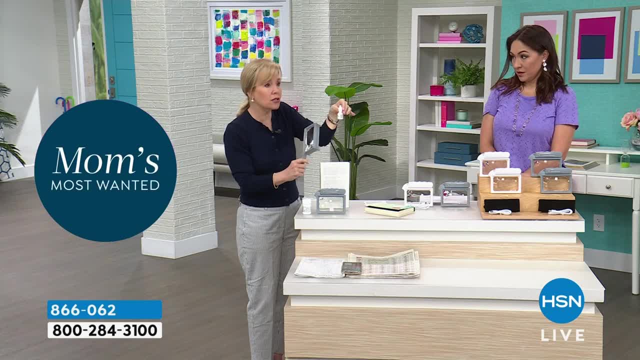 I wasn't sure. I'm like, oh no, Was that the right one? Because look how tiny this little thing is. You can see how itty bitty it is. So now hold on. Let me turn off my lights in here. 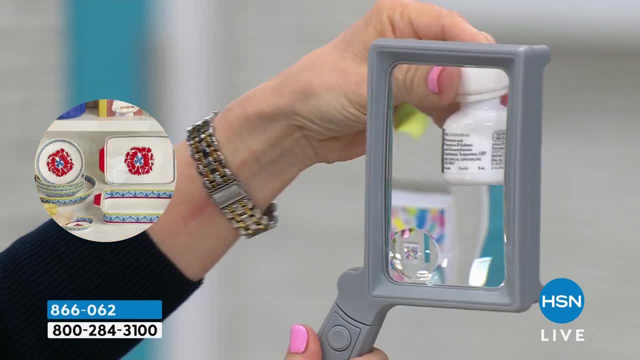 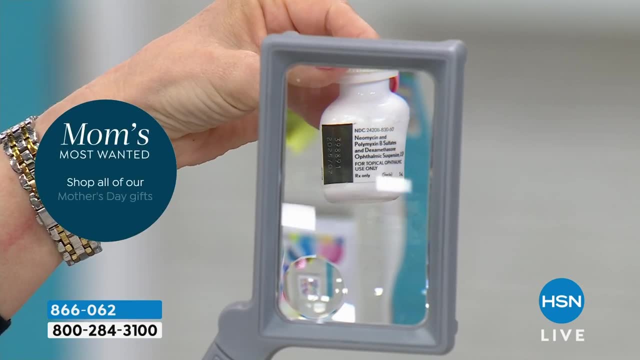 You're going to want to use the lights at home. Look, Hold on, There you go. Let's try and get it. Look how much bigger and better it is. Now I can read what it is that it is for the eyes. 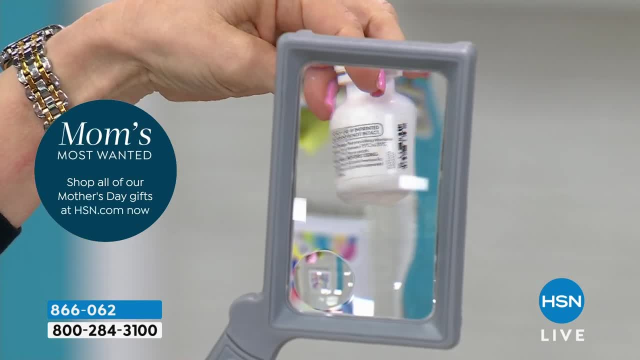 You don't want to put something for the ears? I'm sorry, This was for the ears, But I didn't know what I was putting, Or no, it was for his eyes, But I didn't know what I was putting after I put it in. 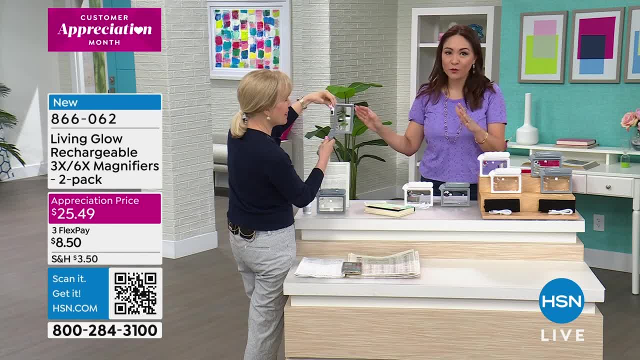 Listen, let me get ahead of everybody. Julie used the magnifier and read this before she put it on her dog. Yes, exactly. But imagine if you did something like that and you're not sure what it is because you can't read what it is. 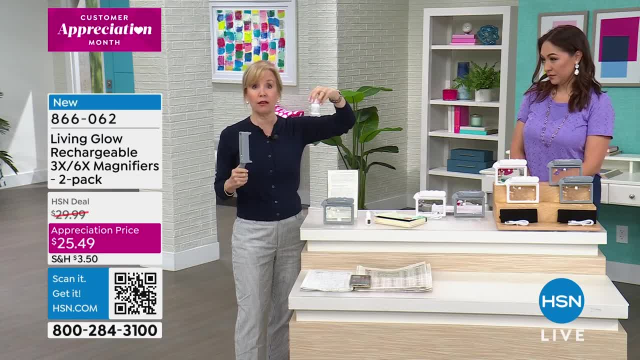 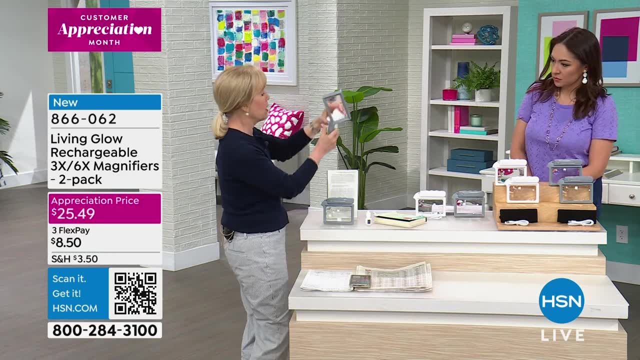 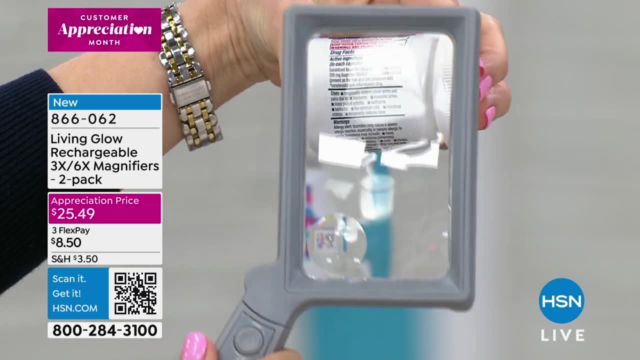 Or maybe it's this which I pulled out of our medicine cabinet and I realized it was expired, because you don't really check those things and you can't see it. So let me show you too, If you just want to read your medicine bottles. and again, just like any magnifier glass, the further that you pull it out, the bigger that it gets. 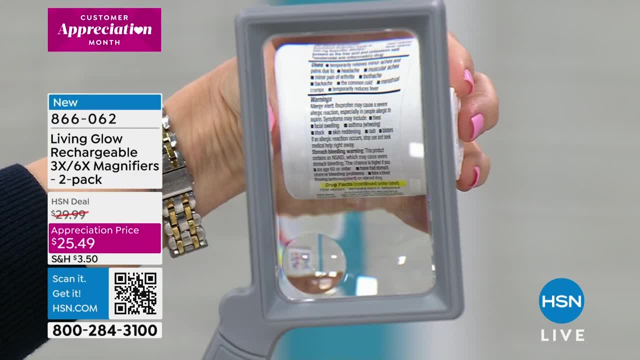 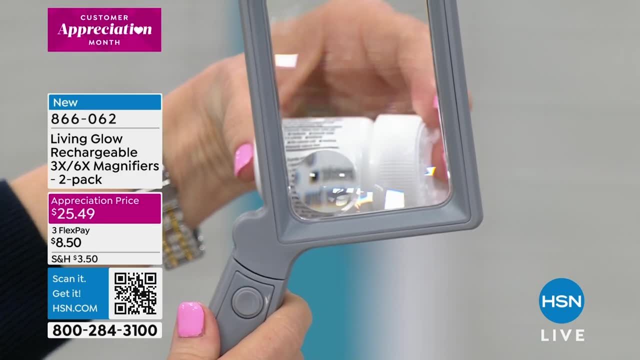 So it's 300% bigger. So the further you pull it out, That's three times the magnification. And then that little right here Is six times. Yeah, that is six times. That might be. I mean, that's way big. 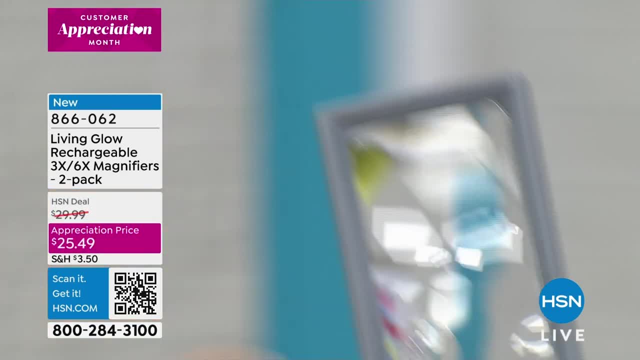 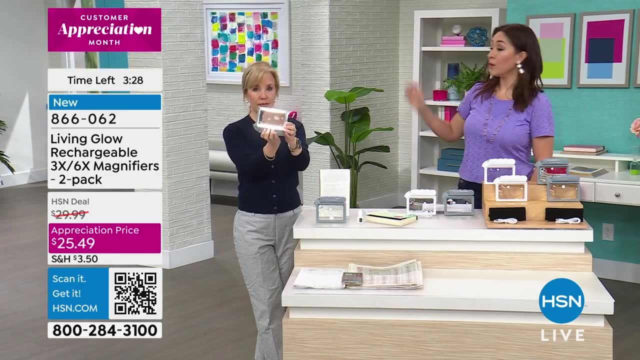 Yeah That you're going to be able to see in there, Yeah, But I mean, I'll tell you and you know, maybe everybody has hit this point in their life where one day- it was probably like a random Wednesday- I was like why are they printing everything so small and everything? 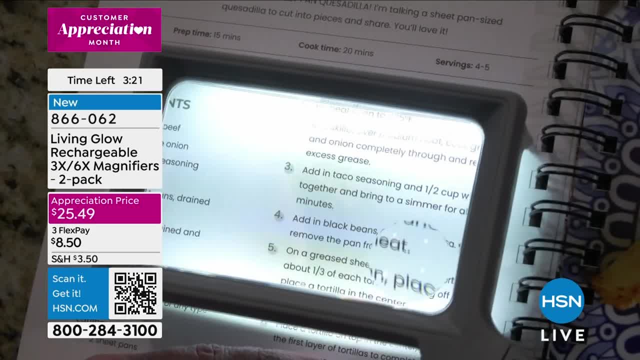 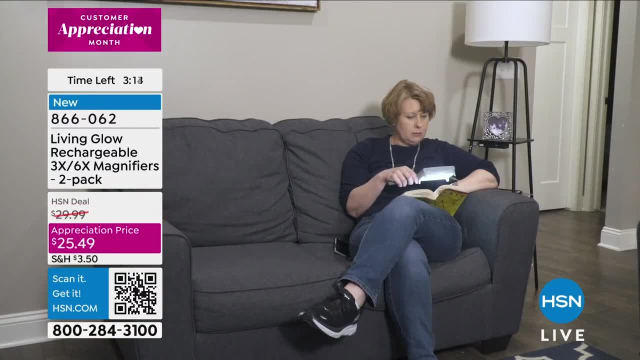 And I was like, oh no, it's not. Things have probably been printed like this my whole life. But now I can't read anything Exactly And I have Riker, my four-year-old, And every medication for somebody at that age is all different. 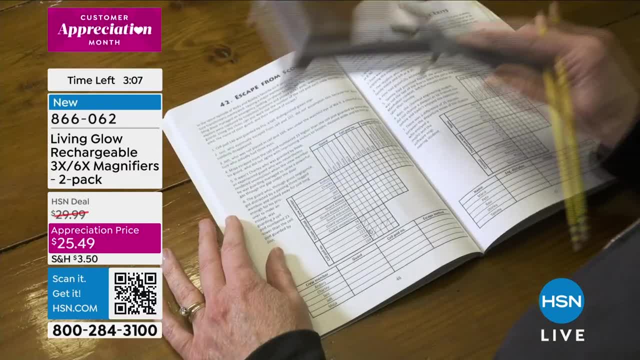 Like his. you know me, I'm like adults. we use the full amount. I have to read every little single thing. I don't want to give my four-year-old too much or too little of anything, Right? So I started being like I need to read everything. 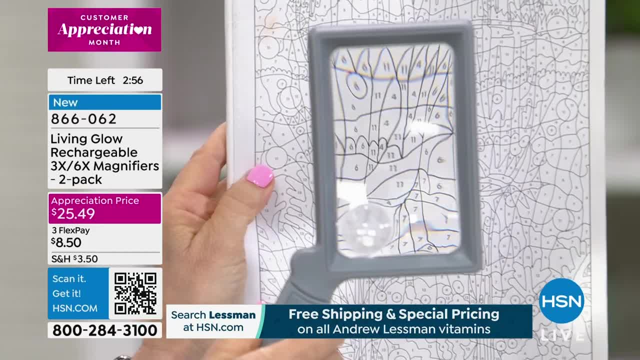 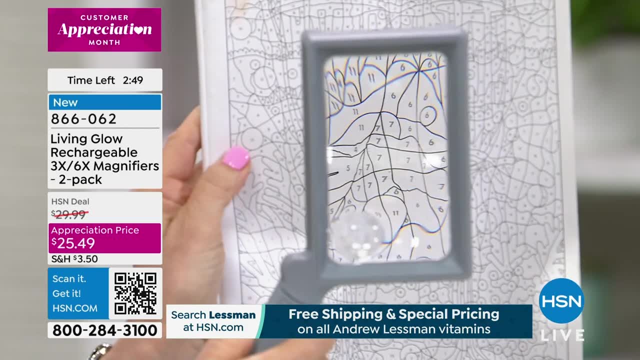 Then it was like menus got smaller, Even like the little menus that you do, you know, at home, when you're going to do takeout or anything. Everything just became smaller and smaller and smaller. Crafters would love this. Crafters would absolutely love this. 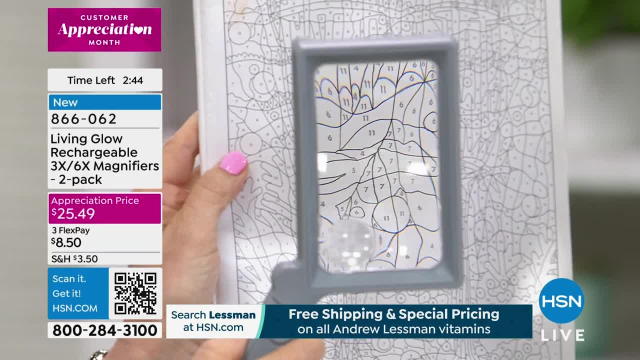 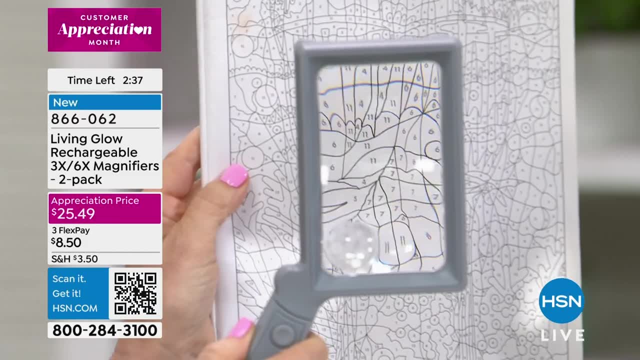 Even if you're trying to thread a needle. Yes, When you get over 40, seriously, the day I hit 40. Maybe that's what it was. Everything, yes, Just everything- would start getting hard to read. This is just so much easier on your eyes. 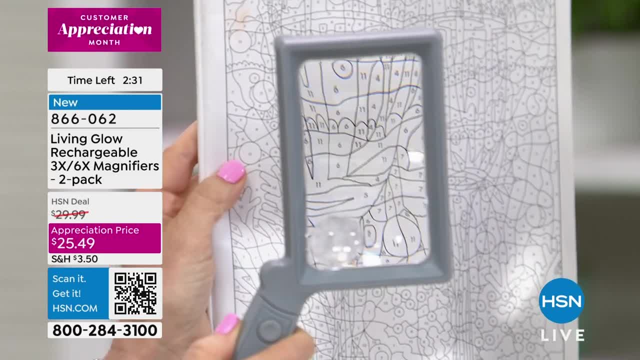 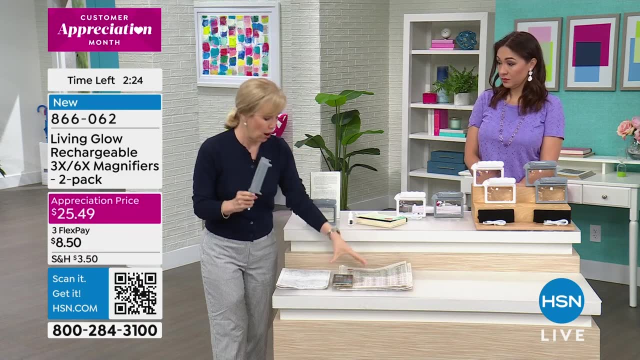 And it's funny, I even have my contacts in And I have one does one thing, The other contact does the other. So nothing is 100%, Nothing is great. So I still need a little bit of help, Even if just let me show you on my phone. 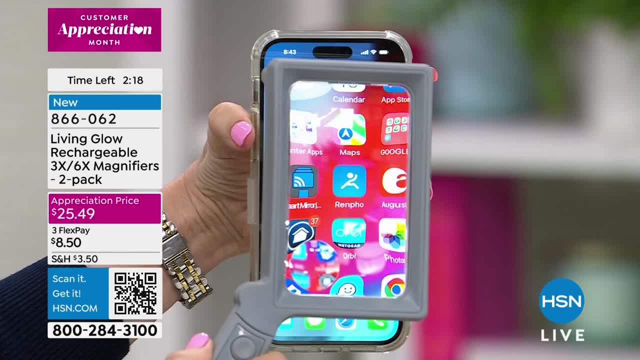 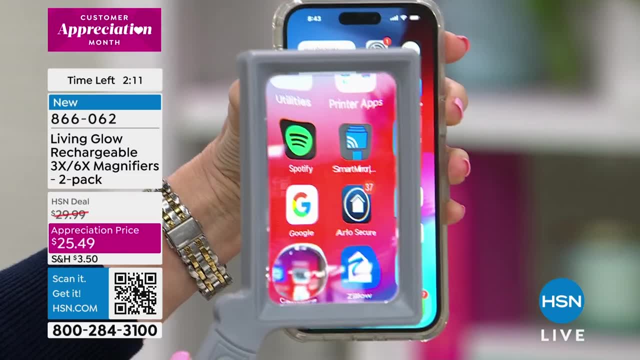 Even if it's just reading your phone, Because not everything. look at the difference Here. it is regular, And then you pull it out You can see how much bigger those are. Look how much clearer. And, by the way, this is glass. 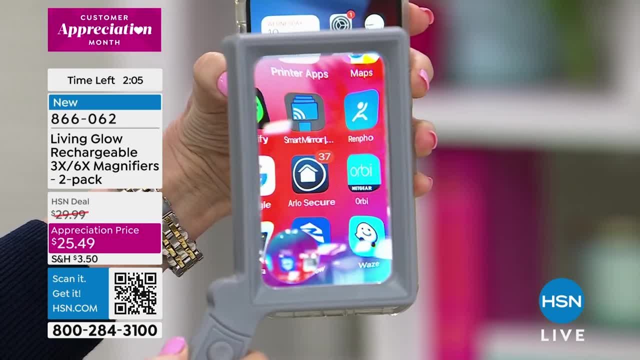 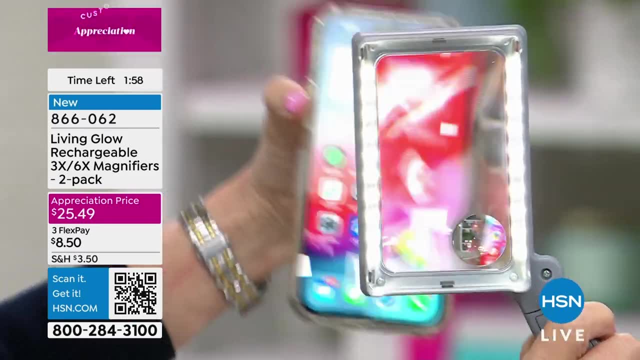 Everything is crystal clear. Three times and six times the magnification On the other side. you just push the button right there And there's the light: 20 lights And the light is daylight. You get 10 hours of using the light on one charge. 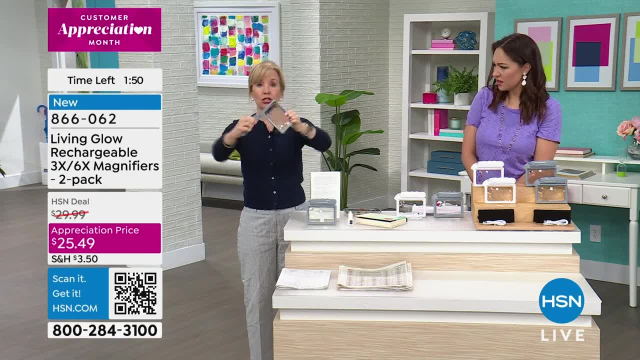 That's a lot. Yes, that is a lot, That is a lot. And then let me show you too the handle. So it folds up like this And you can stand it up, maybe on your little desktop. And then the handle. 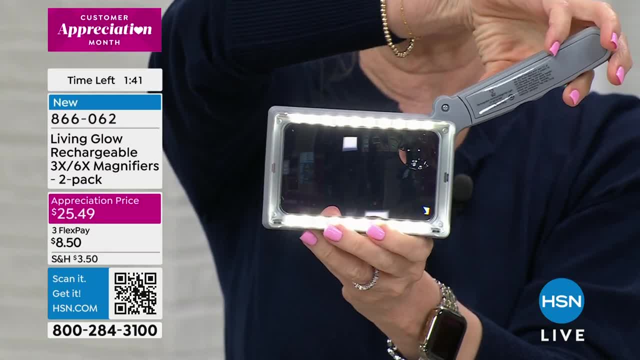 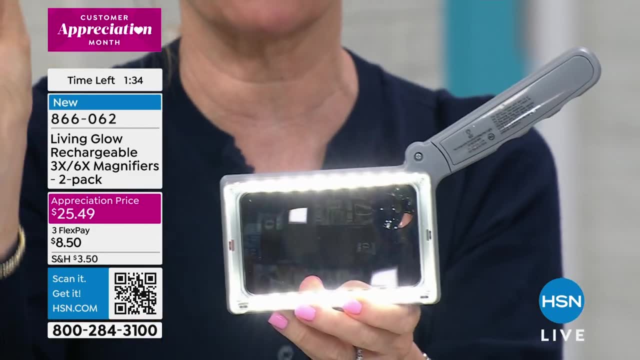 Pops out like this: You push the button, There's those 20 LED lights. I put it on the highest when I'm reading: And this is that daylight. That's the daylight. It's bright white where you can really see. 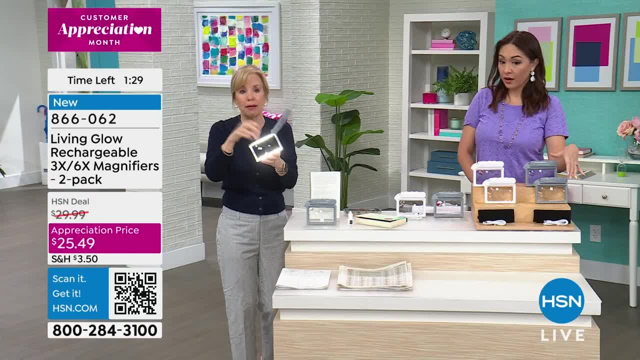 I always use it in the highest And I always have the lights. Just that little bit of light makes such a huge difference. And you're getting two. by the way, I know Julie's showing us the magnification that's on there. 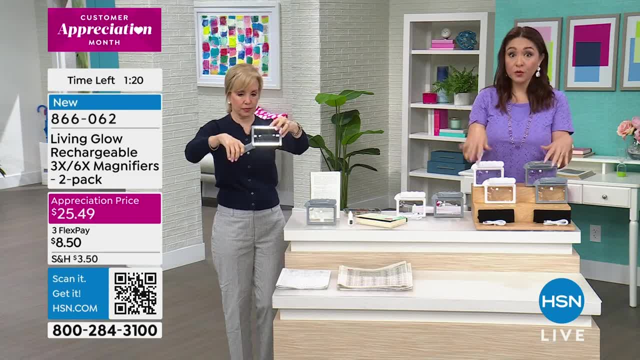 It's two. They both have the light, They're both rechargeable, They both have both three and six times magnification. And if you're like, what does that really mean? It's 300%. Is that bigger or 600% bigger? 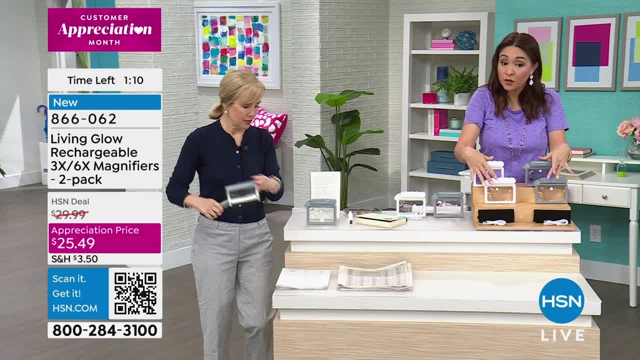 That's what that means: three and six times magnification. And you're getting two of them: two in the white or two in the gray. So whatever color you pick, you're going to get both. You're going to get the little carrying case. 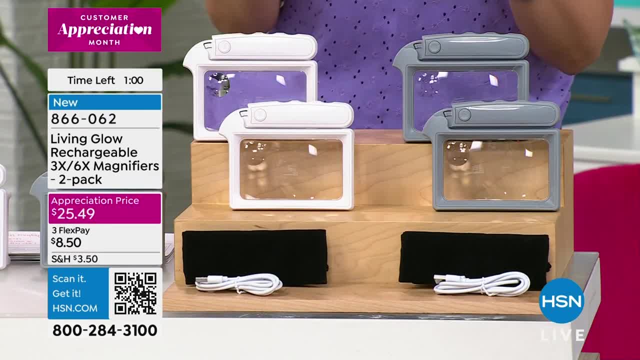 And then you're going to get the cord to charge it up to get that 10 hours of light. It's all white, you know, like daylight light, But you get to pick the brightness levels- three different brightness levels for $25.49.. 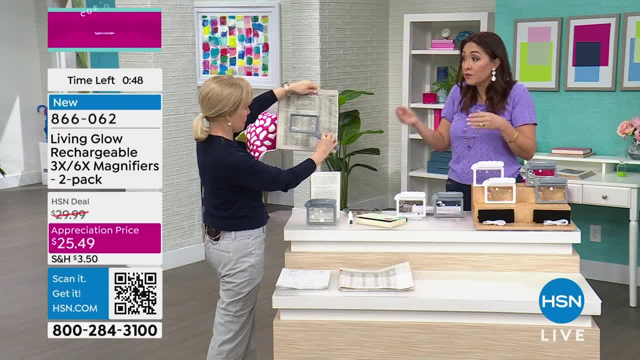 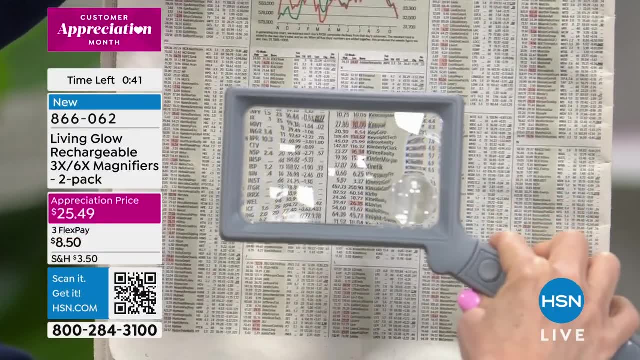 And I use the brightest at home. Keep one gift one. put one in the bedroom, one in the you know kitchen maybe, where you can't see. Keep your medication in, like wherever that happens to be, But I'll tell you on my phone. I use something like this on my phone. 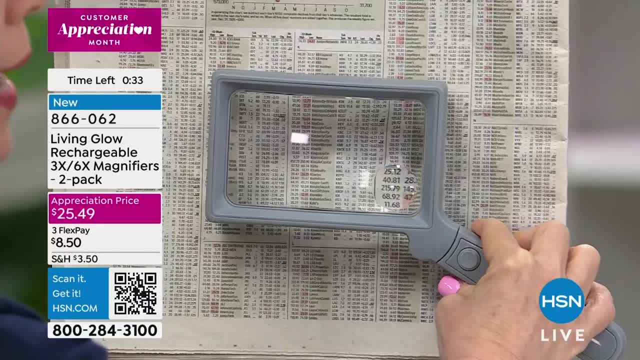 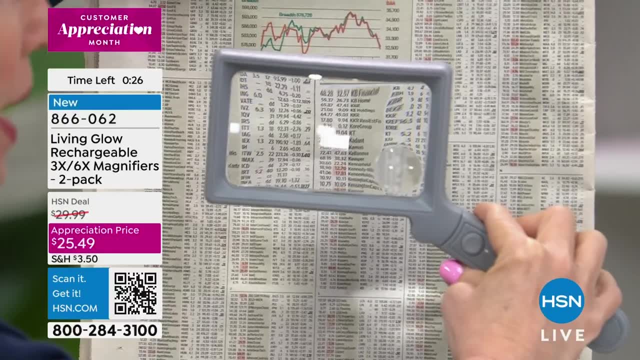 Because if I zoom, then I only get like two words on the screen. I need it to say it's regular size, But I need the words to seem bigger to me. Right, I have my font expanded too, But you can only go so much. 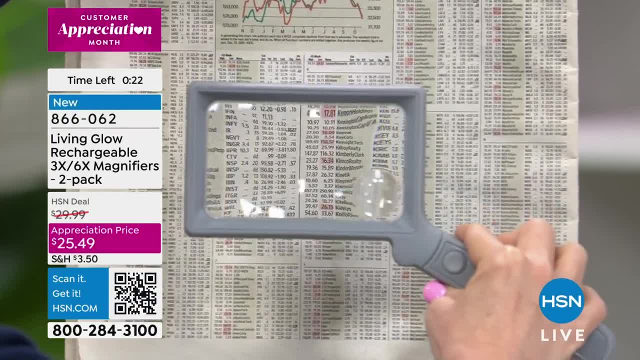 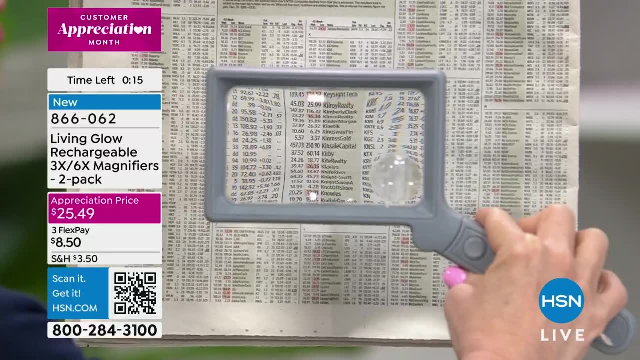 Otherwise it's hard to read. So you can see this. This is probably the smallest print in the newspaper is the stock page, But you can see when you pull it out it gets bigger, obviously, And then I love the handle. 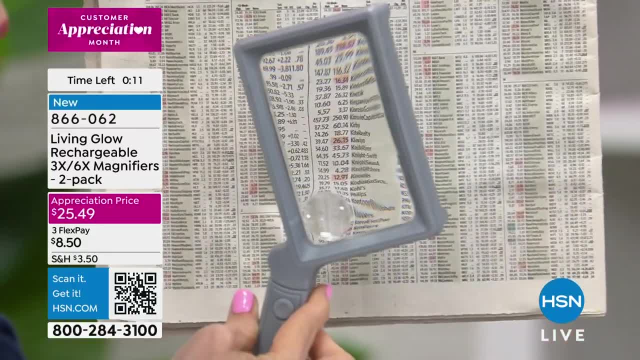 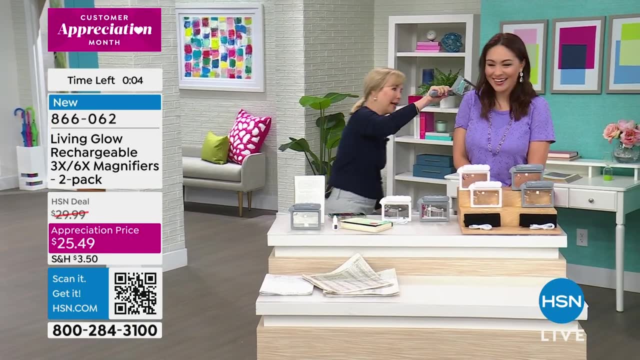 And you can do it this way or this way, depending on what you're reading. This is the exact same thing of what my dermatologists use, And they do this. They go over your whole body. They look for all those moles. 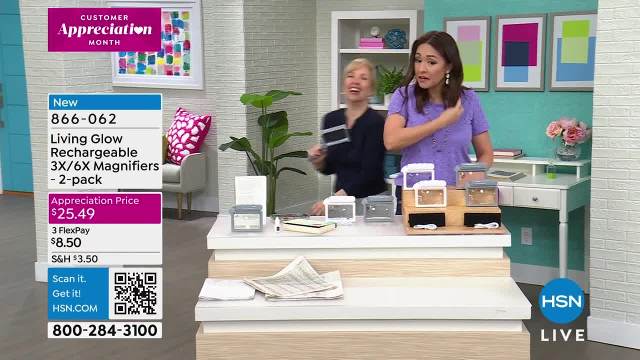 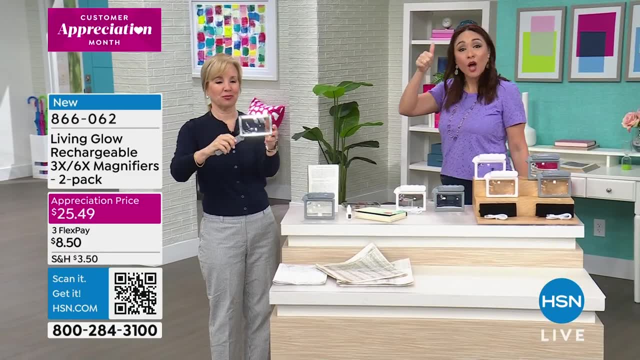 Do you know what you would find? right now, Julie, I have whipped cream somewhere in my hair and on my shirt. That's where your magnifier would go. There. it is Whipped cream. It's because of the game 2-2-2,. launch Living Glow. 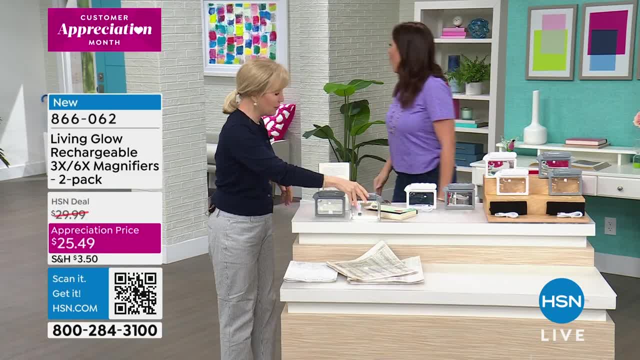 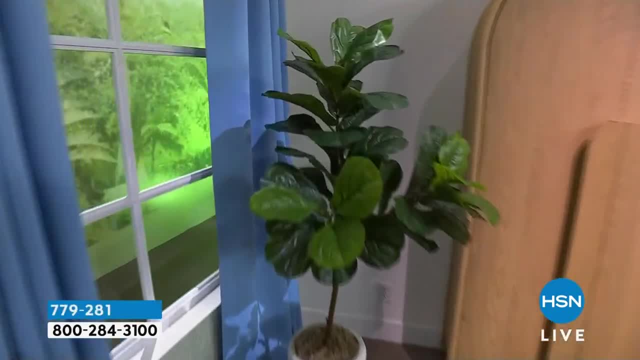 Grab them while we still have them. Yes, Thank you so much. You're very welcome. While I'm walking by, can I tell you, On the set you'll see these beautiful plants And you're like, oh, they must have a professional plant person. 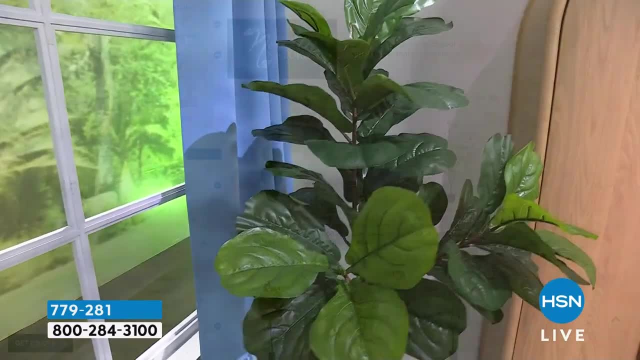 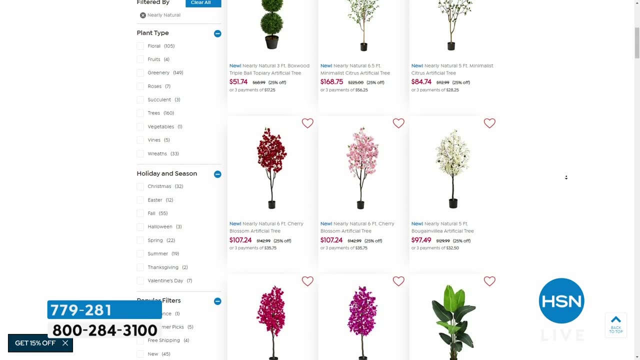 Those are faux, But they really look like natural beautiful plants. It's actually from a brand called Nearly Natural. They are here at HSN. You could also own yours, And they're up to 25% off right now. So if you put in Nearly Natural, look at the full collection. 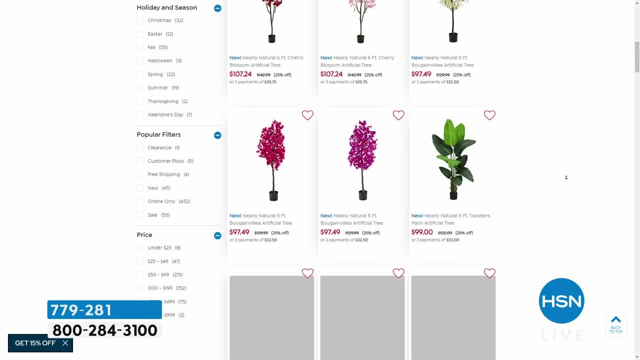 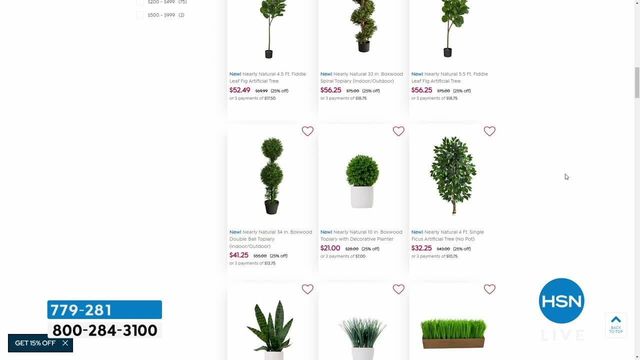 Some that have color, Some that have big leaves, small leaves, Pots, no pots, They're all in there. Okay, I'm not even sure If Carrie Mileto knows this. Did you know they loaded more. Now I get to say we only have one state that's missing. 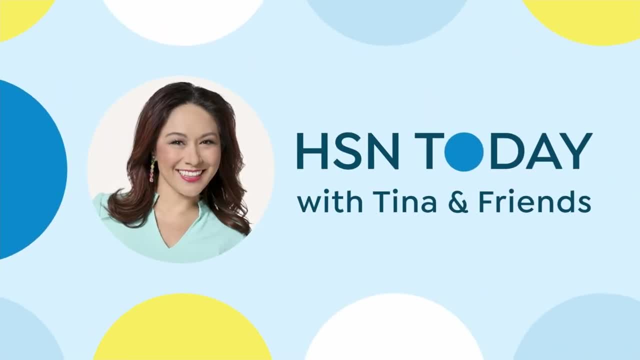 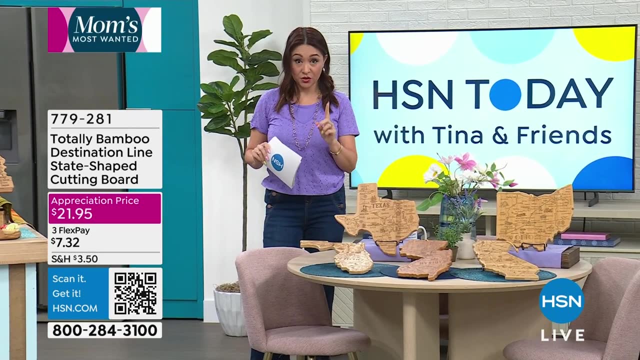 Oh, wow, Okay, Carrie and I talked about this on Sunday morning And I was like saying so many states had sold out. I get to say that I think all my states, except for New Mexico, is sold out. Mother's Day is coming up. 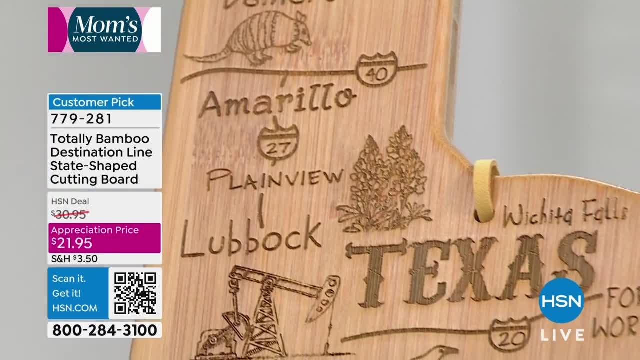 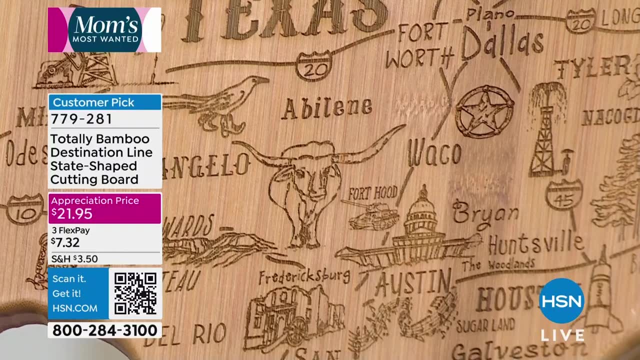 If you're like I have no idea what to get her, She has everything. I love her. She doesn't have this, And it is something that is so useful, functional, It is personal. It's going to bring back memories. 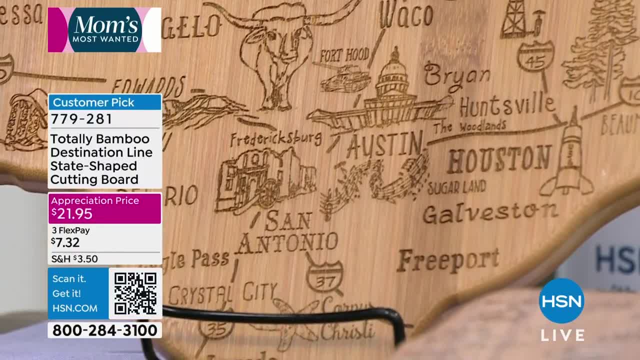 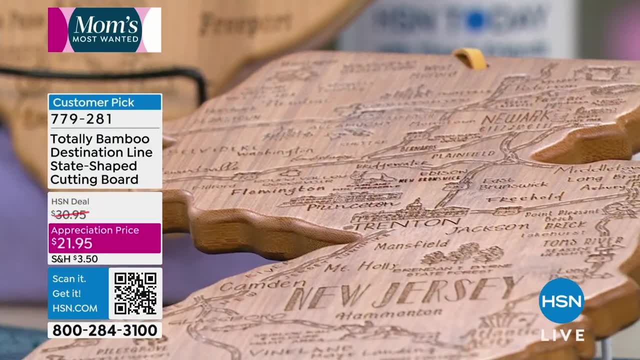 It's going to be clean, It's going to be close to her heart. The customer pick of this is people telling us it's a customer pick because of how other people felt. Isn't that crazy? It is from Totally Bamboo. These are going to be in the shape of the state that you choose. 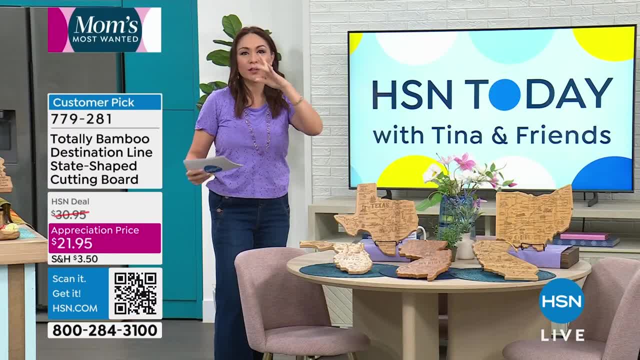 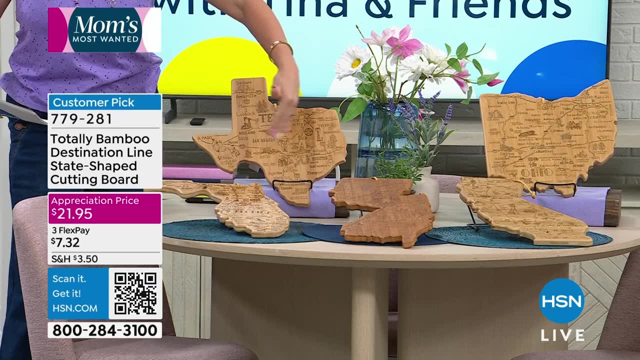 And it's also going to have like cities and little landmarks and fun little things about every single state. Now the front looks like this And you can use this as kind of like a charcuterie board and put all of the different like nuts and cheeses and meats. 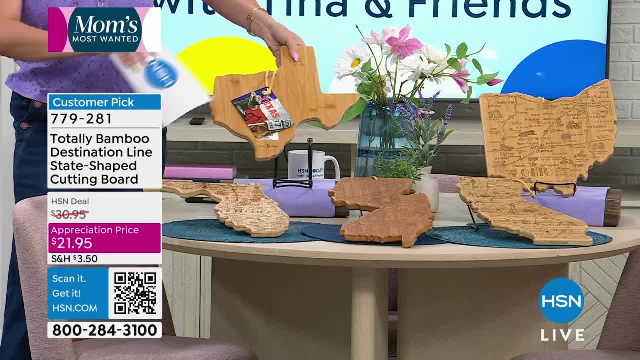 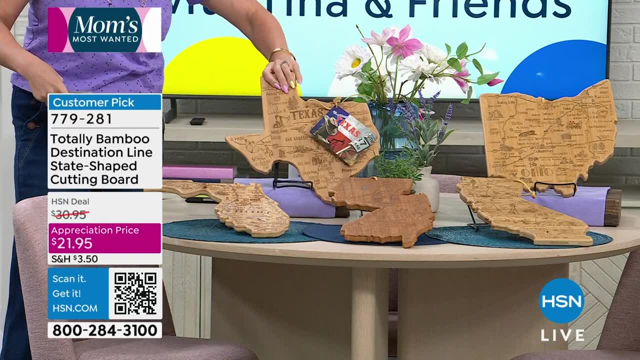 On the back. it's actually nice, Nice and flat. So this is a functional cutting board: $21.95.. All states except for New Mexico. Oh, they put this up here Now I'm not going to know how to get it back up there. 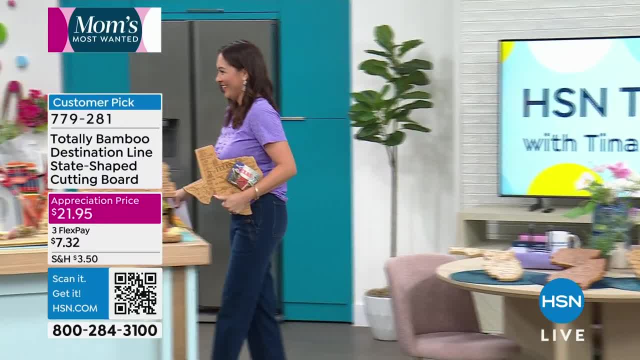 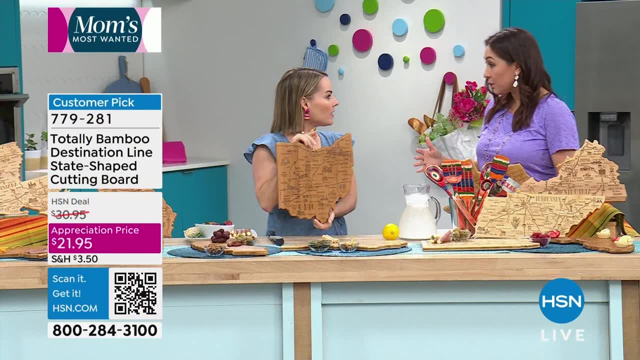 I'm just going to carry Texas with me. Just keep Texas with you, Keep Texas in your heart. I knew I shouldn't have picked it up. I knew it. That's awesome. This is always a big hit. People buy multiples. 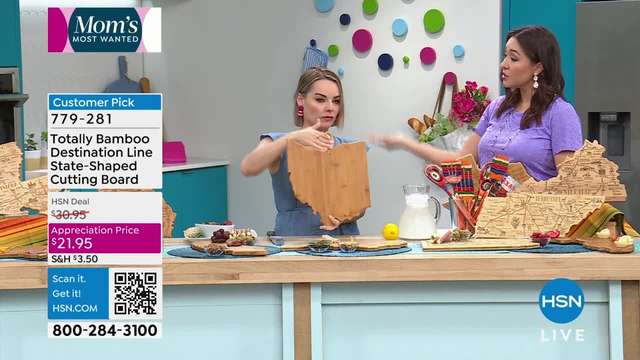 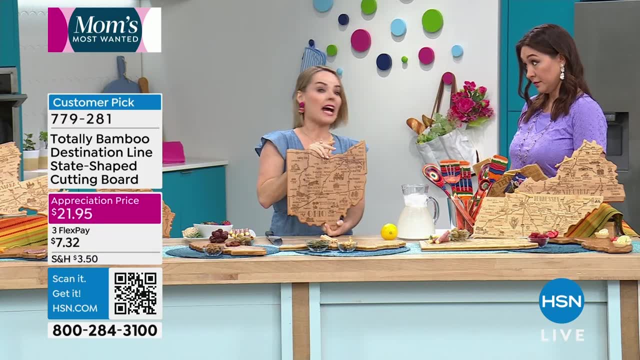 The only negative that I saw in any of the reviews. they said I bought multiples, gifted them all out, came back to buy one for myself. That's what happens, And my state was sold out. Multiple reviewers said that. Yes, it happens every single time. 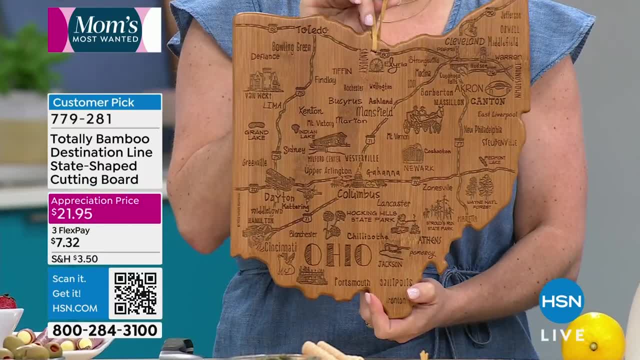 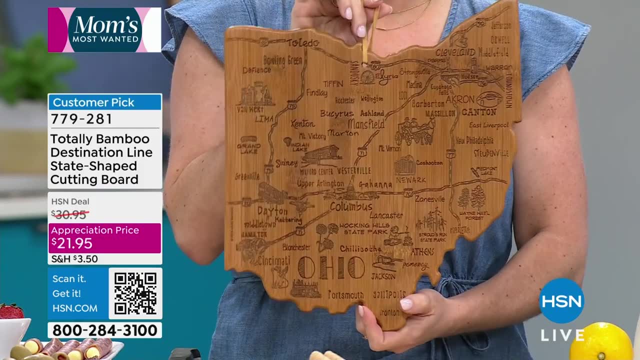 Every single time We were able to scurry up a few more, so we wanted to make sure you had a chance this morning. I don't have any scheduled feedback, so this is it. This is it. So here's the deal. 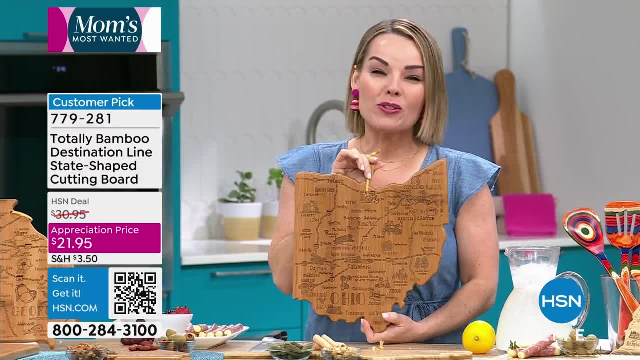 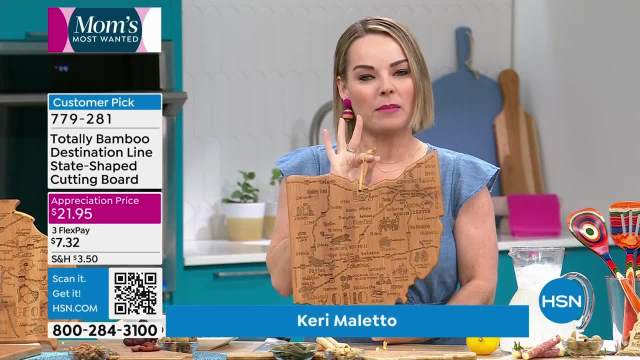 This is totally bamboo. This is a board that's going to give you so much versatility and so much use And, as Tina was just saying, make sure you get one for yourself. First and foremost, get your own state, Get one that means you know something to you. 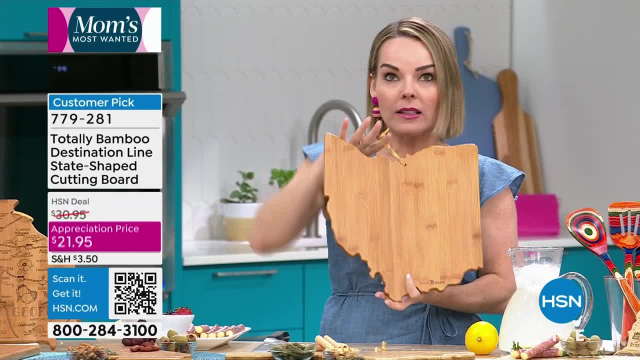 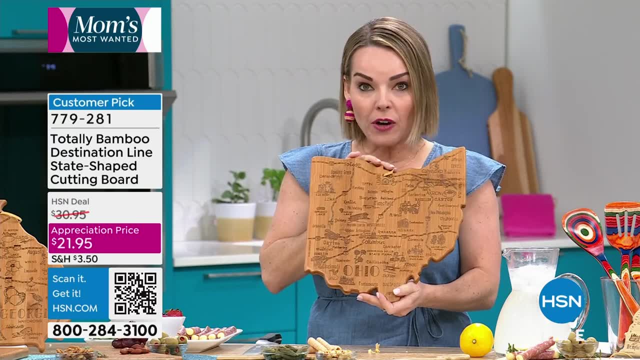 But start thinking about all the different gifting. you know holidays that are coming up And you know this is the time of year where there's weddings, there's people moving around, there's lots of things happening. So on the front, as Tina was saying, this is your like kind of pretty, pretty charcuterie board idea. 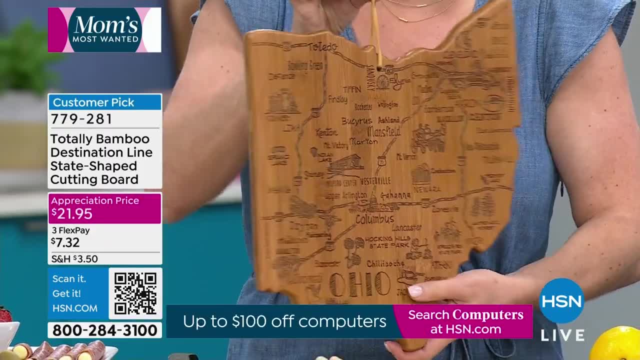 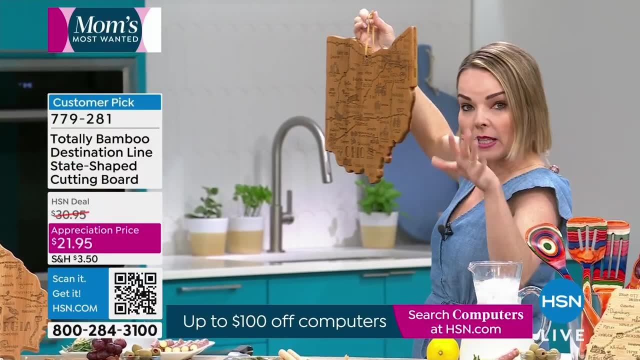 But notice that there is this leather hanging tab here and I can actually hang this on the wall. So when you came into my house, if I pop it back like this, it's hanging back on my kitchen wall until I'm ready to use it. 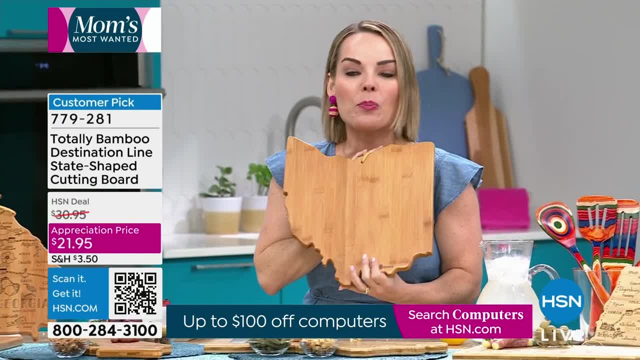 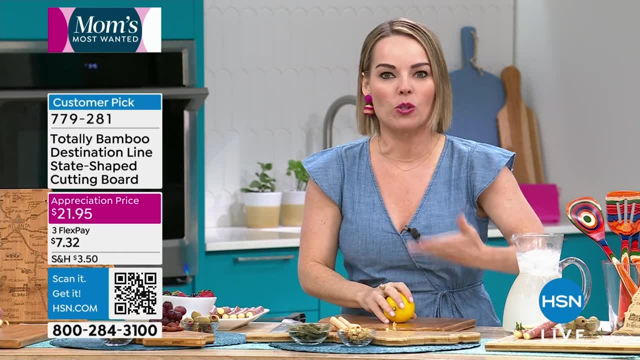 Then, when you take it down and you come to this side, it's a beautiful. It's a beautiful, durable bamboo cutting board. So I'm even going to start there and just start cutting. But what I love is that I love items that give you multiple purposes and multiple use. 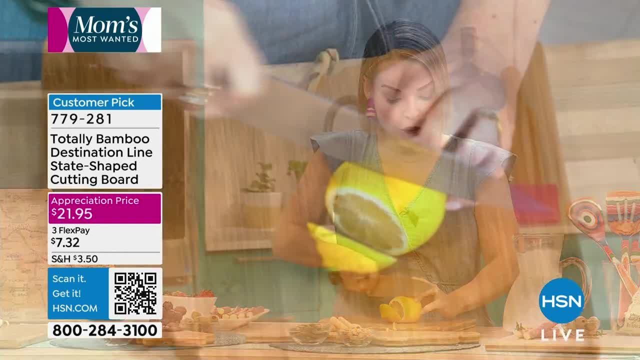 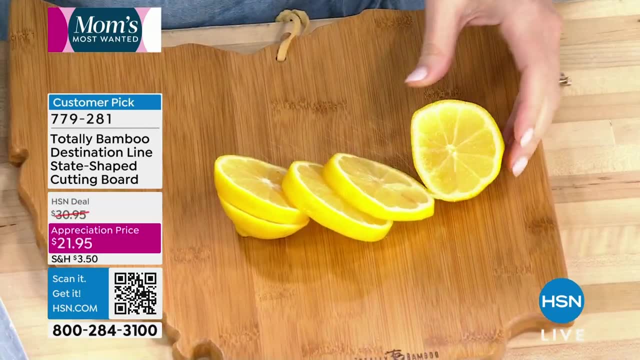 Because then it looks beautiful in your kitchen. but when it's time to get busy and do the workhorse items, this is less prone to marring. Bamboo is a really, really cool Wow. this lemon doesn't want to cut. It's a really durable substance. 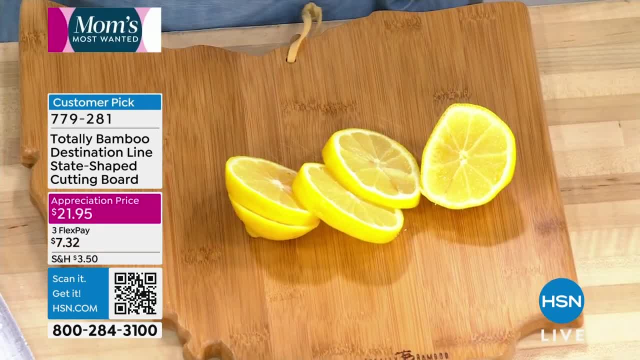 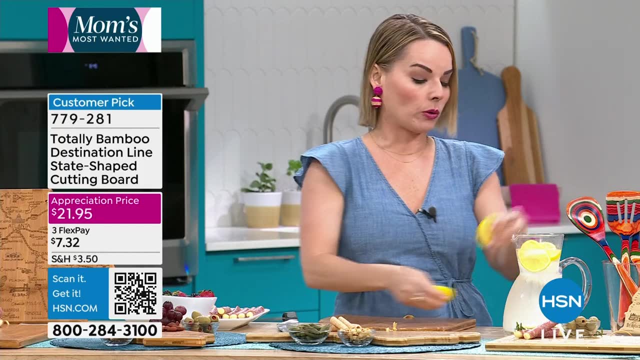 So that is, A lot of people think it's wood, but it's actually made from grass, Yeah, And so it's a really sustainable thing, which I really love. But also, I had bamboo. I had bamboo in my kitchen before I ever worked with Totally Bamboo. 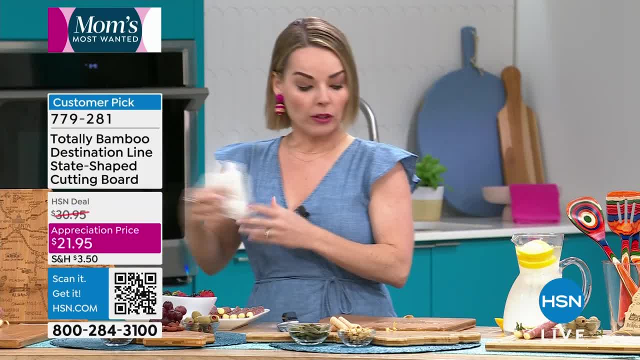 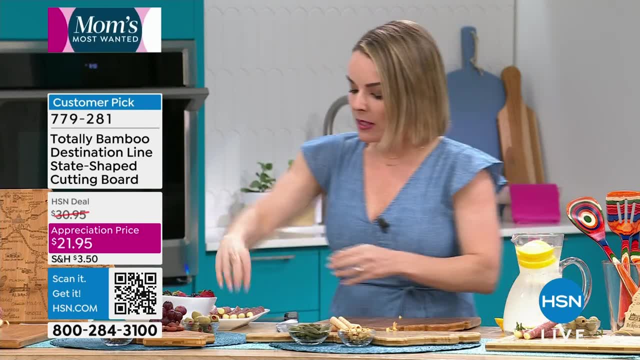 So I really love this for the fact that again, you're going to have this in your kitchen for a very long time. Now I'm done cutting, So say I was cutting all my items ahead of time. Now I can flip the board and now I can start making it beautiful, because maybe my girlfriends are coming over. 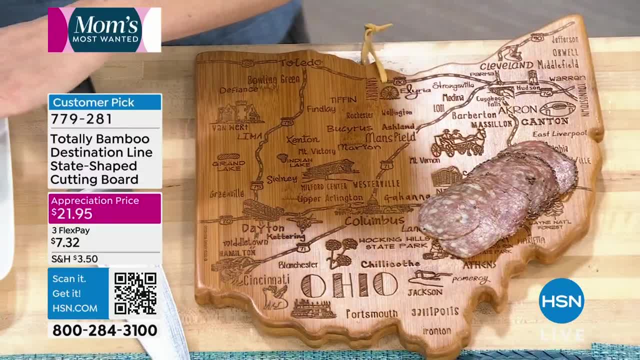 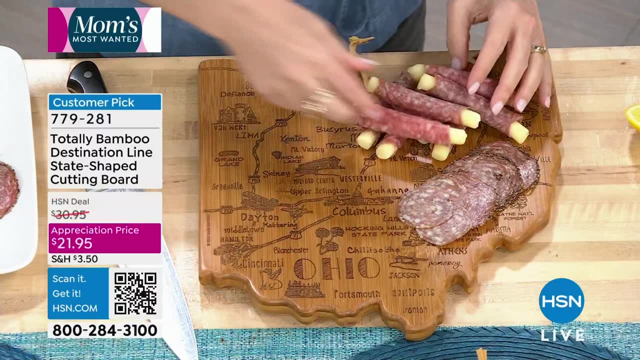 Maybe I have some family coming over later and I want to make a really beautiful charcuterie board In a matter of seconds of just placing food on here. it looks gorgeous because the board does the job for you, So you don't have to know how to be a charcuterie master. 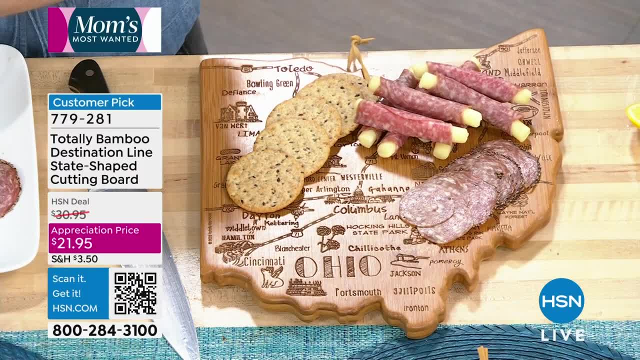 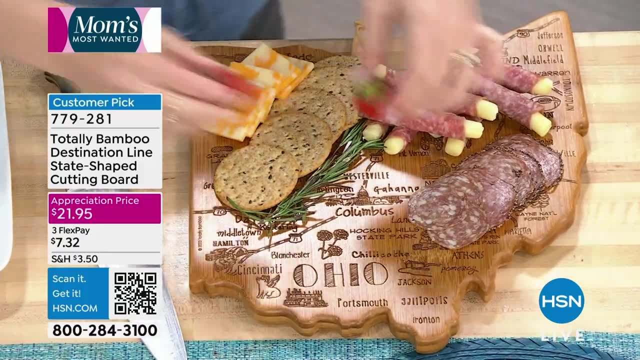 I've seen books on how to do charcuterie, you know, because it sometimes feels a little overwhelming. So here, look at this. It just made it look like I went to some really expensive place and got this really beautiful board. 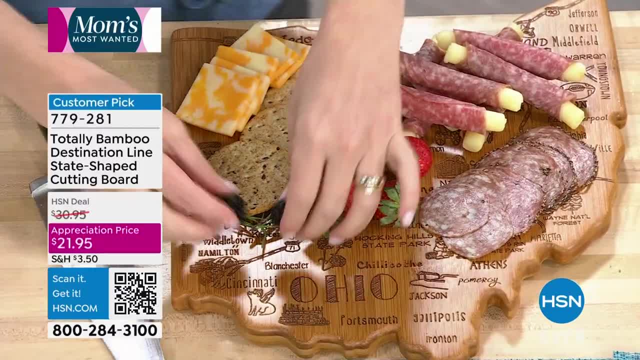 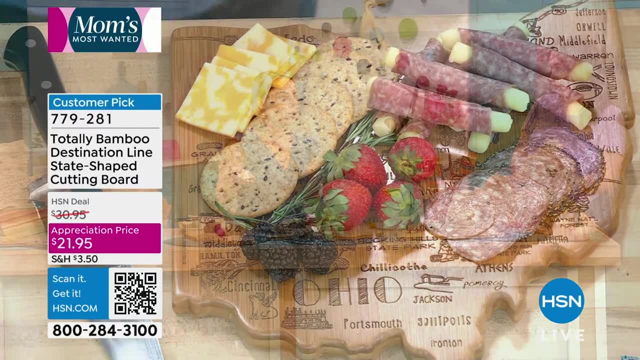 And I'm just talking and placing things. So this will up your quality level of how your boards look And, as Tina was saying, this makes such a beautiful gift, So, like when you give it to people, they're going to use it. 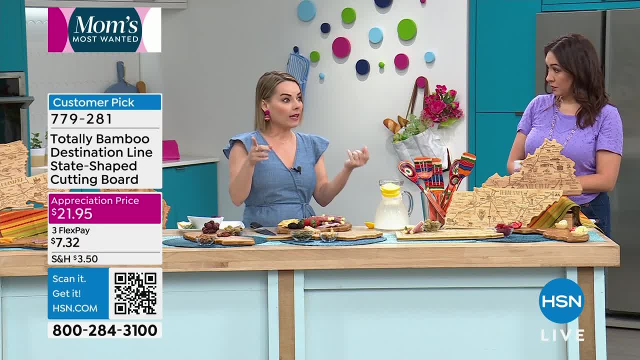 And I think it's like you know, sometimes we give gifts And I'm telling you, lately I've been pricing out, Like if someone's birthday comes up and I don't want to get something chintzy, But like it adds up fast. 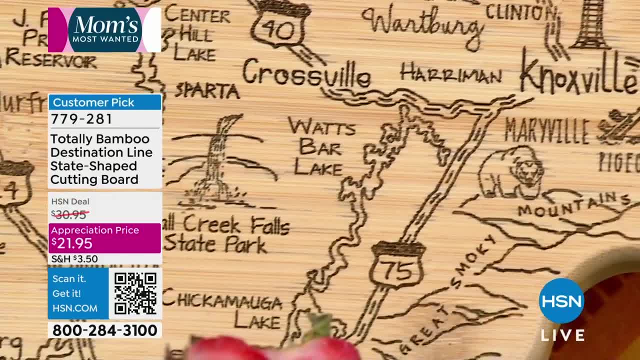 Like. if you're trying to like, I want it to feel like it's a good, you know right, I don't want it to feel chintzy For $20-something. Are you kidding People? think you spend $40, $50.. 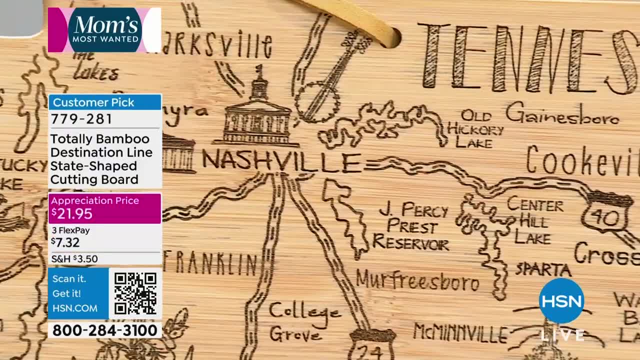 I read the reviews. You know how much I love reading reviews. Do you know what? one reviewer said? What? They bought this for an 8-year-old. And it said: I bought this. I think it was a nephew, an 8-year-old nephew. 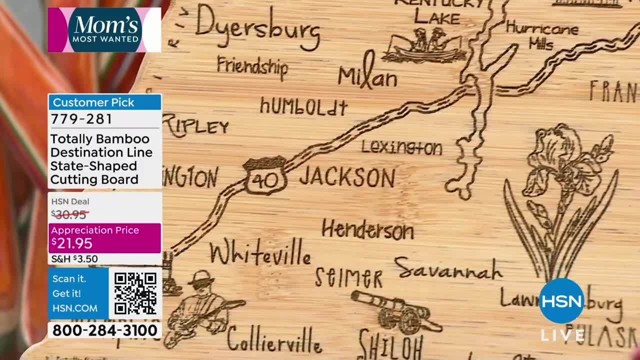 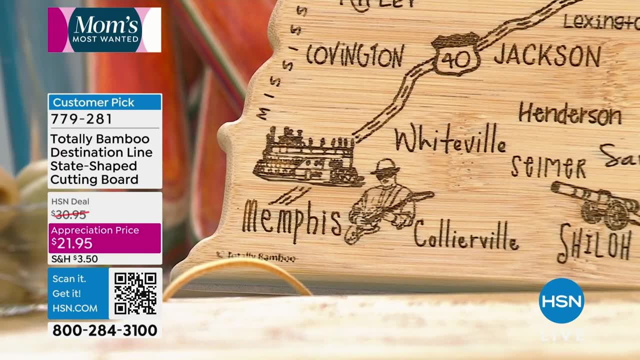 And they said that he loves like states, Like he's really into that. I love that 8-year-old loved this as a gift. Like how crazy is that Somebody was saying they bought several of these and then handed them out to family members. 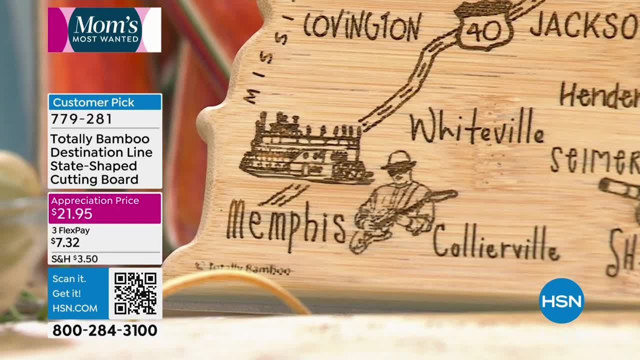 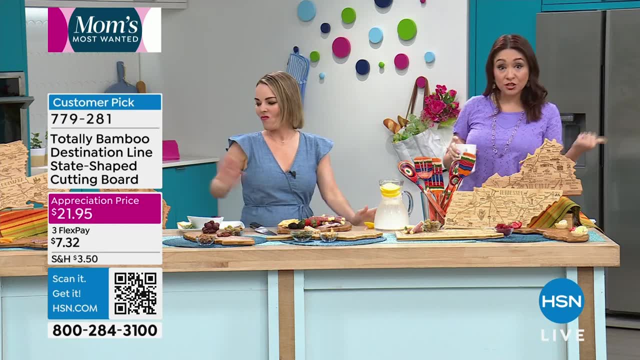 And then, when they were opening them in front of them, they opened it and started sharing memories about the different cities And where they you know, the memories of this town and that town. It is a conversation starter. That's another reviewer said. 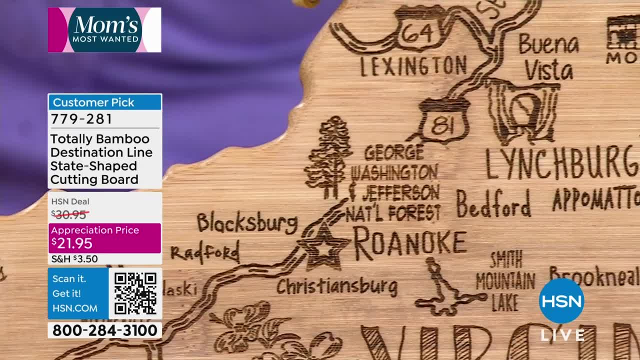 It's a great conversation starter, Especially if it's in like a charcuterie and you start eating away. You start eating away. I remember being there. What is this? Yeah, exactly. And if you're thinking about Mother's Day, 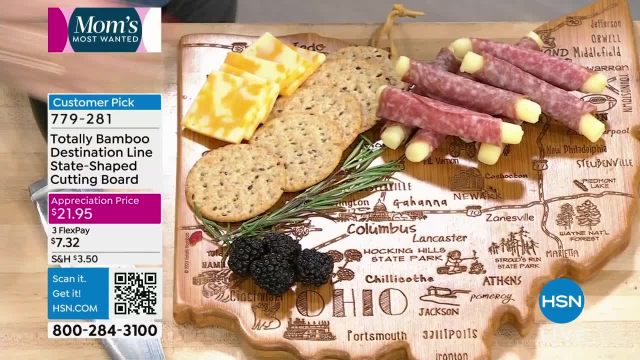 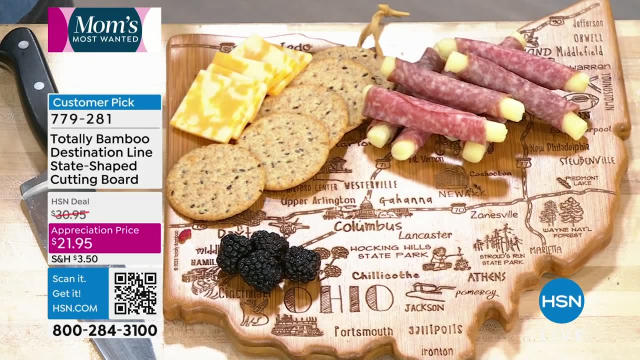 And I started that way Because I know that's the next holiday up Is think about this. Maybe she lives in Oklahoma, But she grew up in New York, right, And she's always like talking about New York And she's always like the memories. 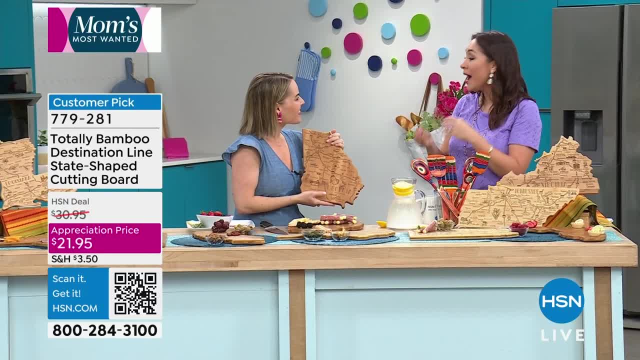 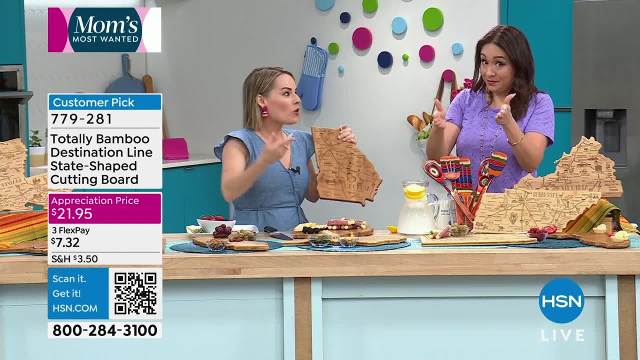 And I remember doing this back there And you're like Mom, but you live in Oklahoma. I can't buy New York stuff in Oklahoma, 100% Right. Yes, You can only buy that state you're in, Right Right. 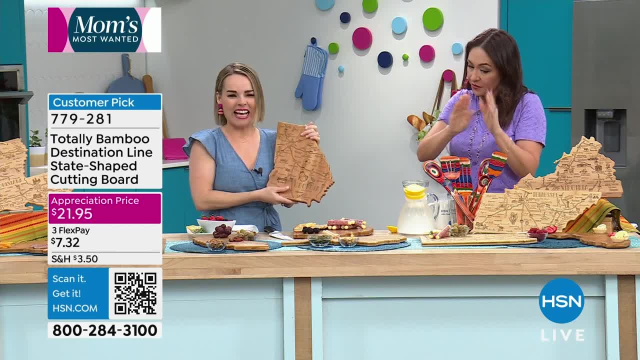 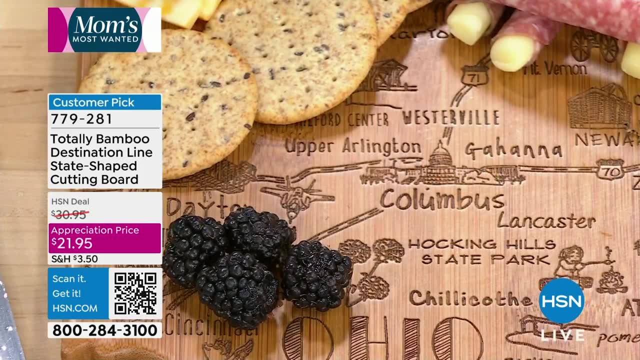 We have all, except for New Mexico. My New Mexico people shopped fast and got the last of those, But we have able to get at least A little bit in every state available. So if you need multiple, now is the time to buy it. 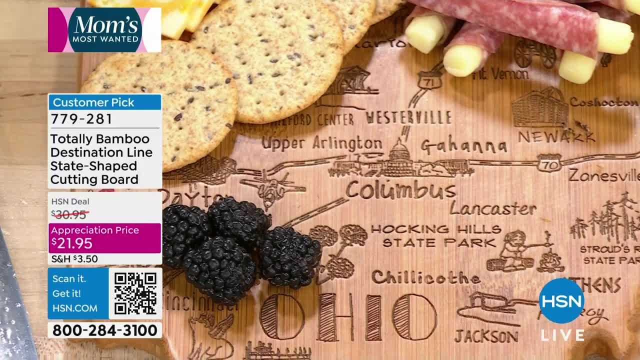 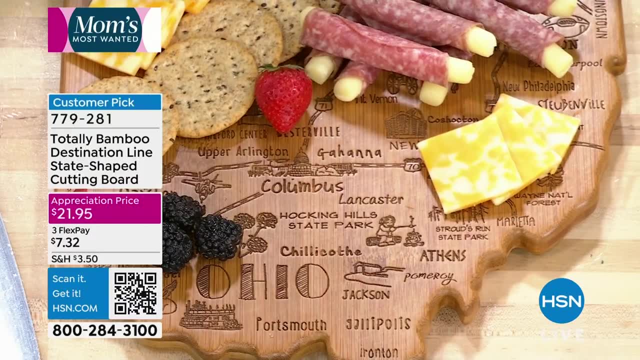 If you are thinking about anybody And if you're even on the fence about maybe you also need it. Get it now. Get it now on a sale price. Grab it while we still have it. And these are all laser like engraved in here. 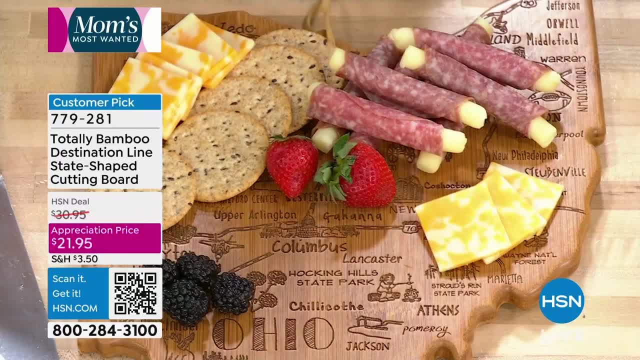 So it's not like something like on top of it, That's correct. That will like peel away or anything like that. It's not going to peel away, It's not going to fade away. The laser etching that happens when it goes on here is forever. 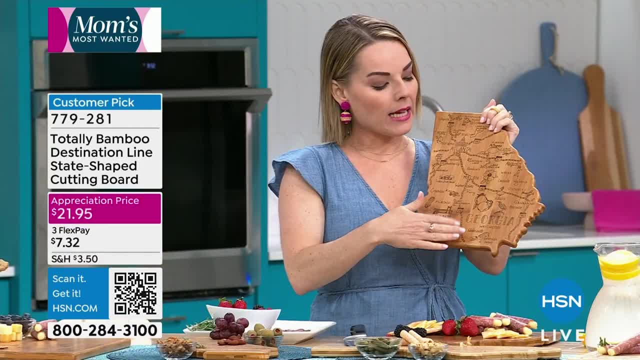 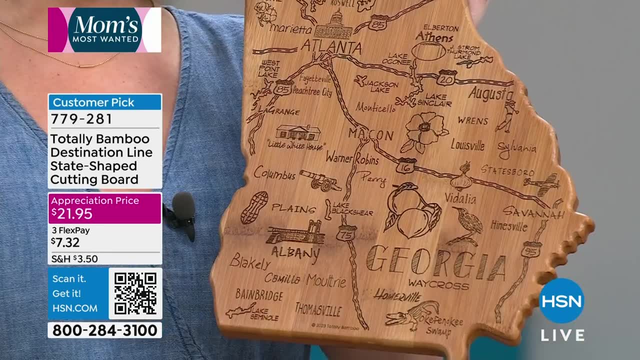 I mean. so it is laser etched into the bamboo And All the different locations, All different spots. Let me tell you a little bit about Totally Bamboo. When we first started here in 2022, we were a company of 25 people. 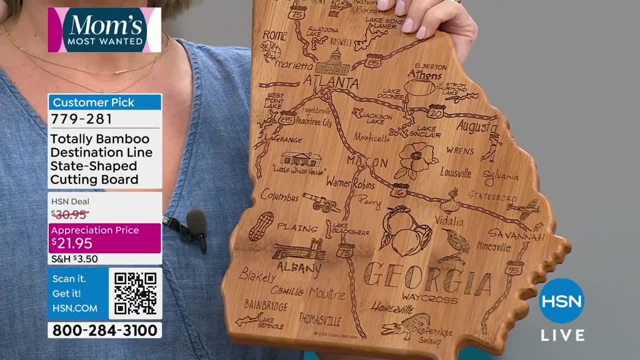 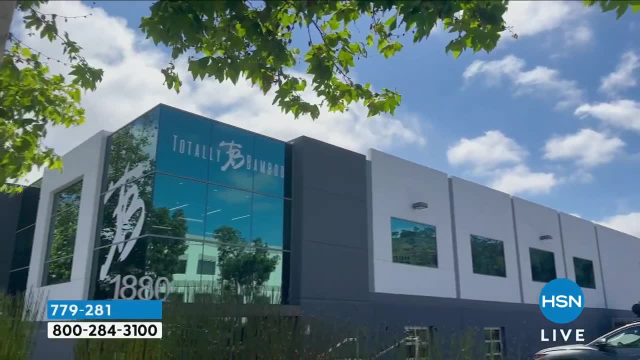 And we are now a company of 45 people And that has everything to do with you. here at HSN. We want to thank you so much. It's so appropriate that we're here for Customer Appreciation Month, Because we appreciate you so much. 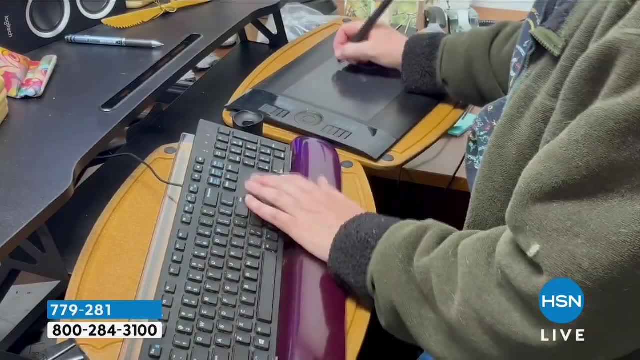 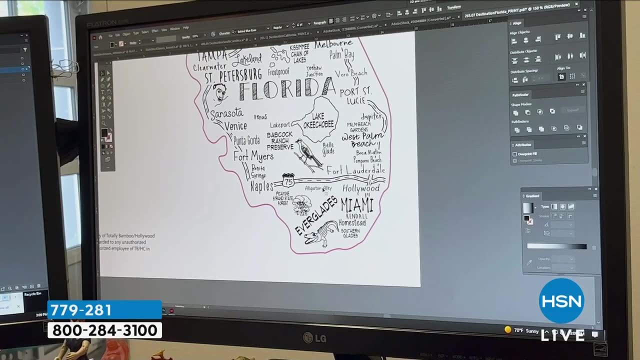 This is our facility in San Diego, California. This is Joelle. So each employee- There was about five, six employees that each got like five or six states And they had to then go And find out everything about those states. 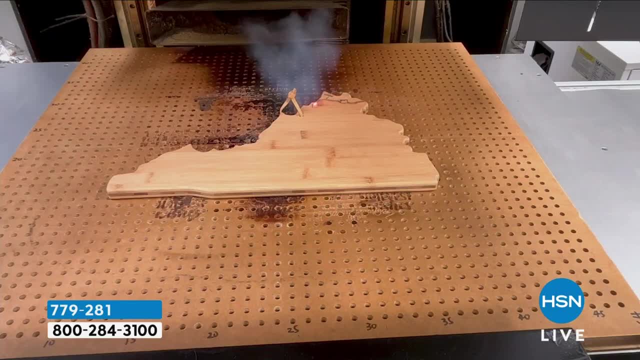 What were the good landmarks? What were the state parks? What were the really fun things about that state? And then Joelle was tasked with making it look cute. So when you look at how cute this is And how it has all the little highways- 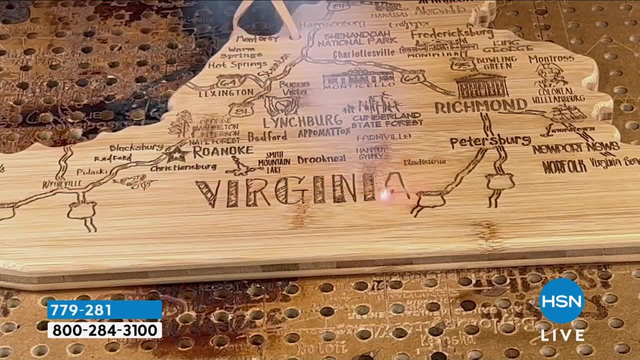 And, like you know, in Florida there's a little alligator And a little boar And all this like really cute stuff. She's the one who did that, And then that's the laser etching process that you just saw happening. 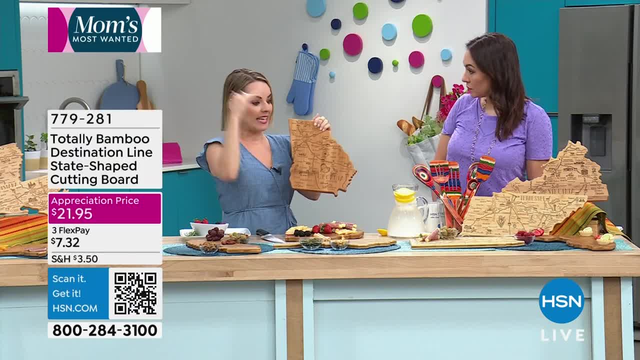 Which I thought was the coolest thing, Because it like jumps around And it's in the bamboo. So even when you feel it, you feel that it's not at the top Right, It comes down, It sets underneath. 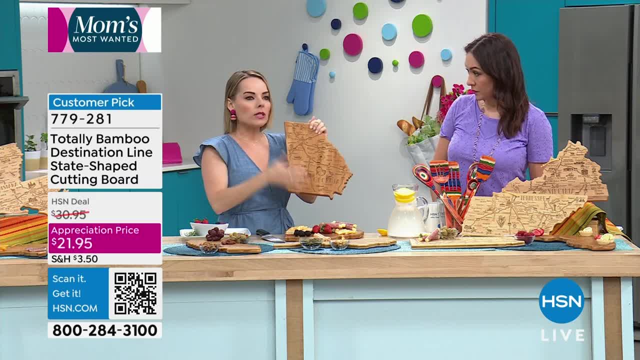 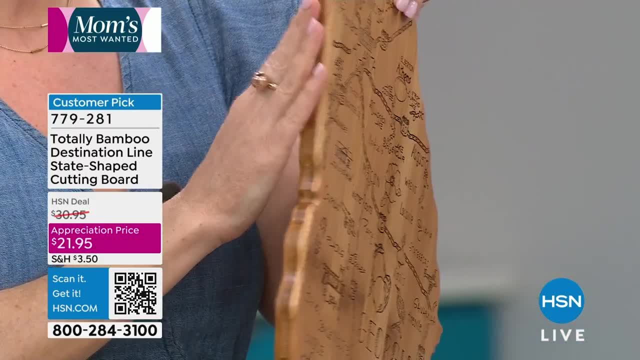 It's like flush- Yeah, High quality. When you touch this, When you feel this- Even the side of it It's thick, It's really strong- You know that this is something you're going to have for a really long time. 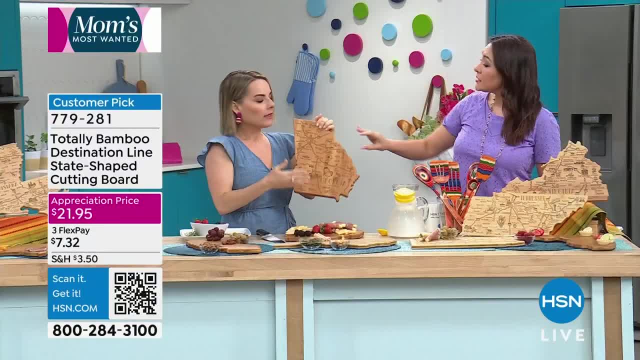 So, whether it's decor, Whether it's charcuterie, That's what I was going to say. Some people take their cutting boards and they put it inside a drawer Right, And they only bring it out when they're cutting it. 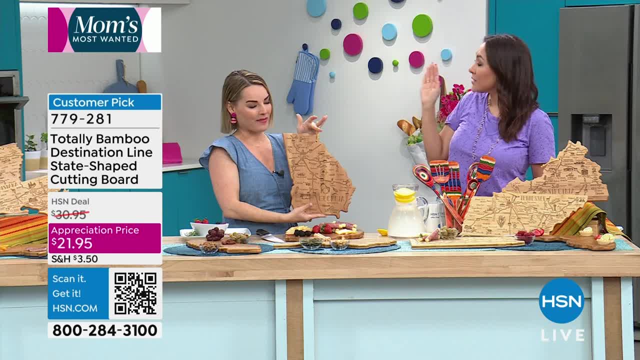 Your gift will be displayed all the time. That's right, Because I would say 99% of the people that get this, Yeah, Or buy it for themselves, Or buy it for themselves. Hang it Absolutely, Because it's pretty and it's decoration. 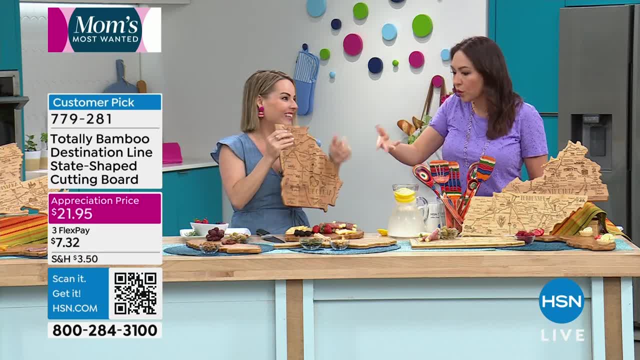 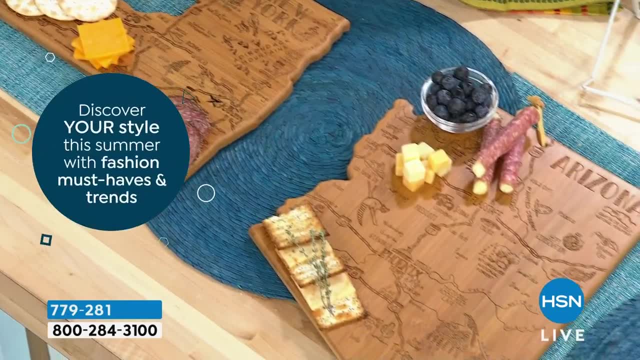 Absolutely. So you're not buying a cutting board that goes into a drawer or into a cabinet. It stays out, It gets hung. I will show you what I do in my house Really quick. Kentucky, Kansas and Vermont: I've got last call on all three of those states. 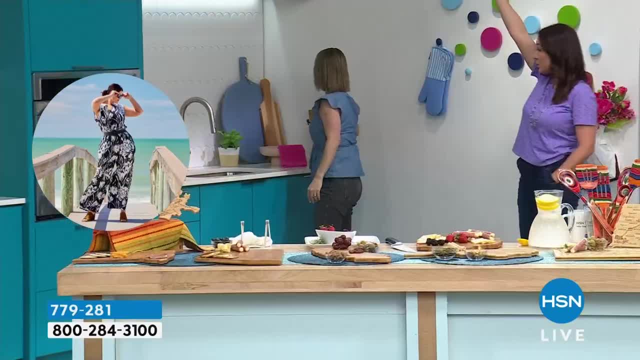 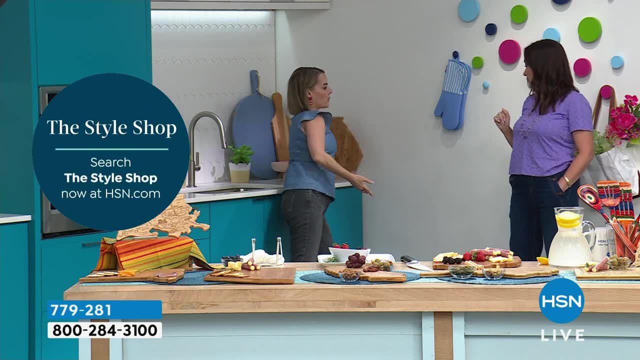 So I want to make sure that if you do want one of those three states- Kentucky, Those are my people- I want to make sure that you get the one that you want. But look, Just propped up, If you come to my house. mine was like that: 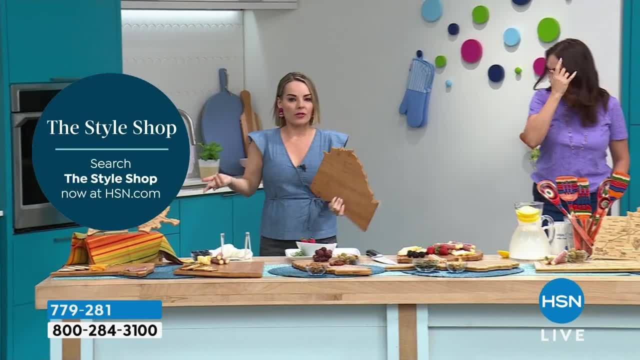 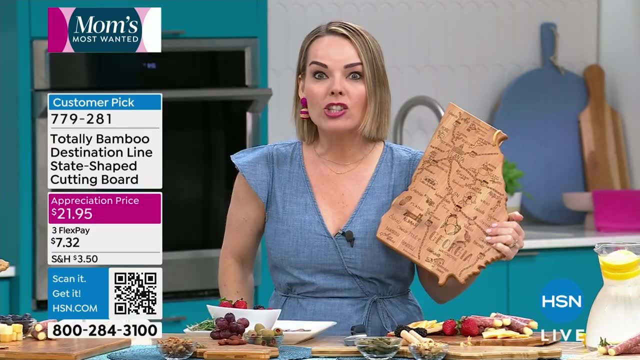 And now I just hung it. So I changed mine, But I reserve the right to change my mind. I move things around in my kitchen all the time, But it always stays out, And when people come over they go: oh my gosh, that's so cute. 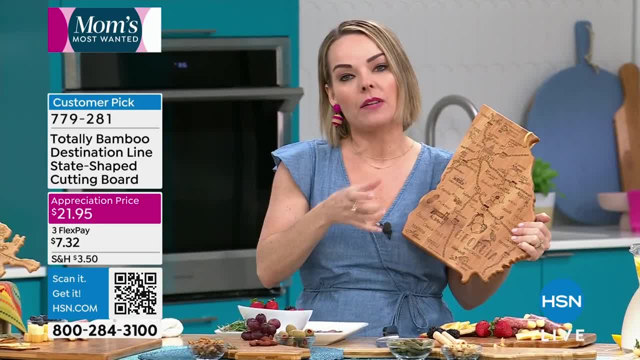 And then we start talking about it And so it creates talking points. Everyone loves their state. So if you have a state that you were maybe born in but you don't live there anymore, But you know, I was born in Florida. 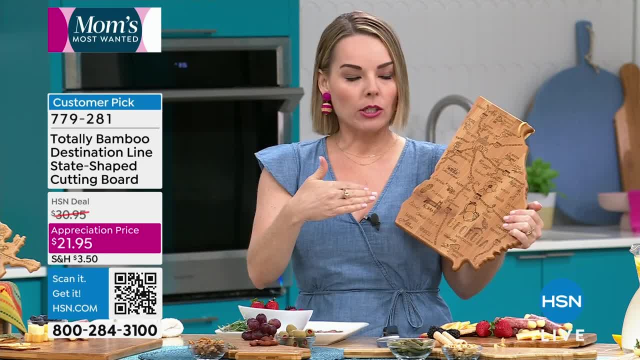 I live in Atlanta, Georgia now. My husband was born in Pennsylvania, But again we're in Atlanta Georgia, So we have Pennsylvania, We have Florida And we have Georgia, And so when family comes over from different places, 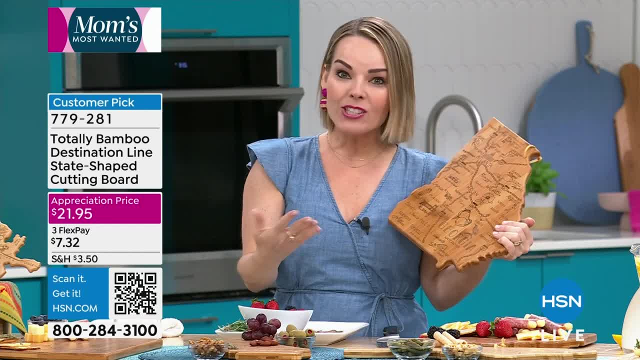 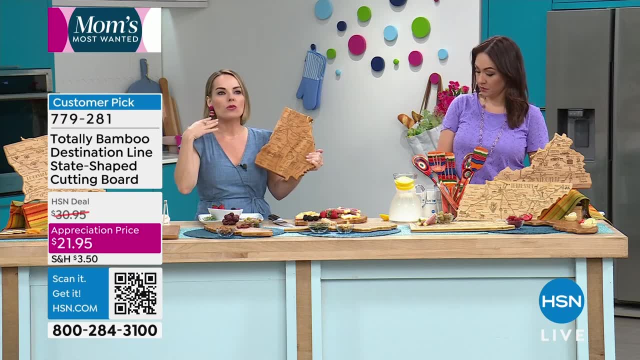 we'll put those boards out And then it creates talking points. Oh my gosh, look at this board. Oh, do you remember when we lived here? And then you remember we took that trip and we went over, you know. So that's exactly why these are so nostalgic feeling. I think you know. 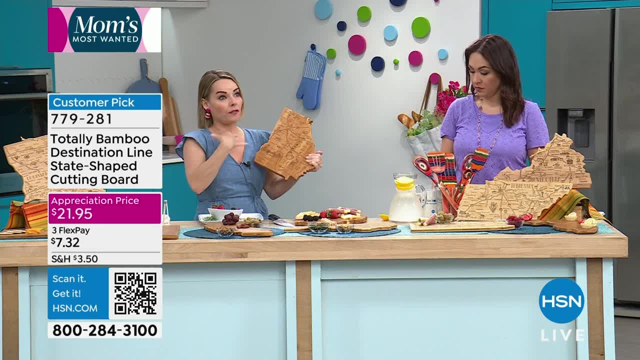 And people like to. as you said, if I'm in Florida and I have a family member, Look, I have a lot of family members in New York and New Jersey. I can't find anything that's New York or New Jersey in Florida. 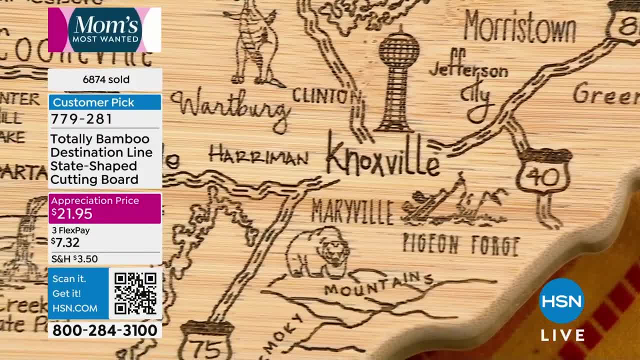 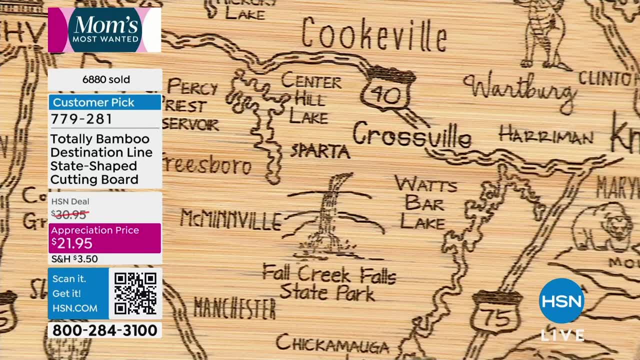 So being able to click and know that you can send this to a friend, a family member, Direct ship to them. yes, Exactly, That's what makes this so fantastic. And if you're just like you know, get in the gift closet full, get as many as you need. 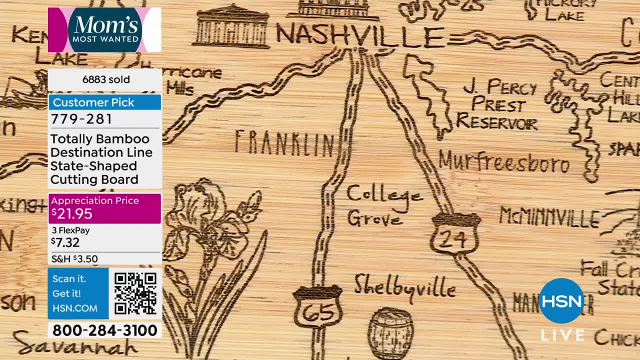 If you're in real estate- mortgage brokers, real estate people- these are great for closings. Like to give to the people. you know what I'm saying. So a friend of mine in Georgia bought a whole bunch of these for her mortgage closings. 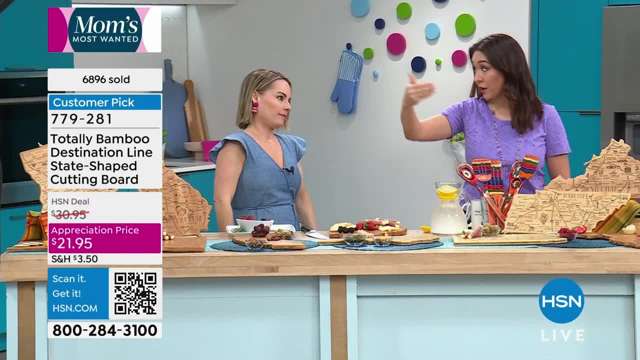 You can't go wrong. Graduations around the corner. I think a lot of people will be going to out-of-state colleges- Their new college- And going different places. Kind of give them either the board where they're going or a board where they're leaving. 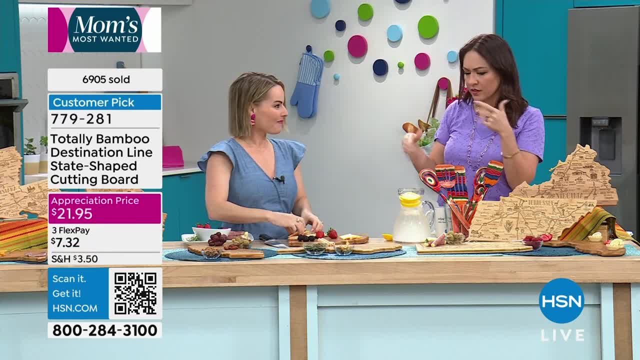 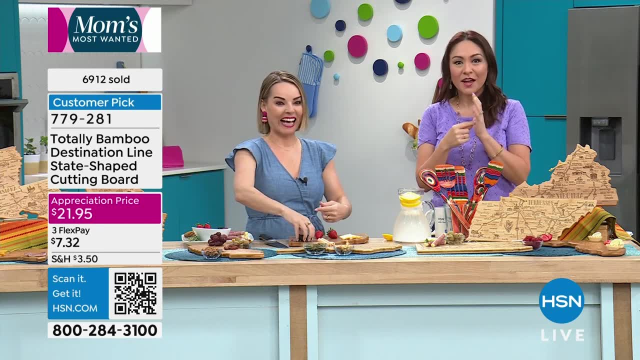 It's like even when I say conversation starters. So Carrie and I have done these boards several times, But last presentation on Sunday, I took Arizona, which is my home state, Right, And I was like, look, it says nothing on here. 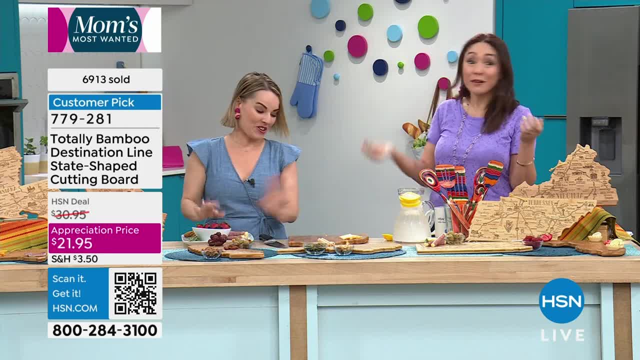 And she was like: why would they put nothing? I was like, because there's a city called Nothing Arizona. I did not know that And I've driven through it a million times. Why they would put nothing on there is because now we've had a whole conversation about Nothing Arizona. 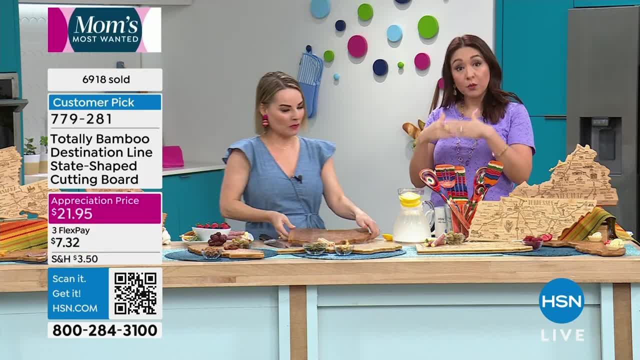 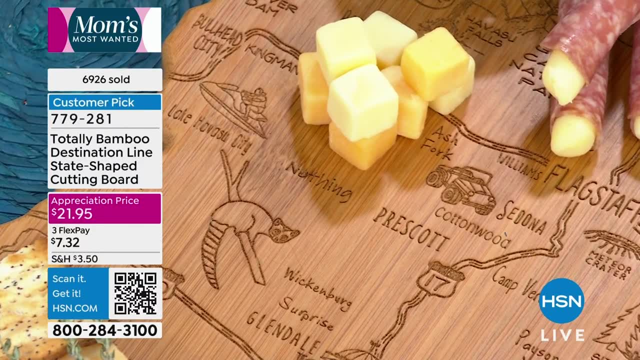 And now I know, But look, Arizona's home for me. I currently live in Florida, where my son was born, And my husband is from Kentucky. Right, Oh, are you guys zooming in on nothing? Oh, look, there's nothing. 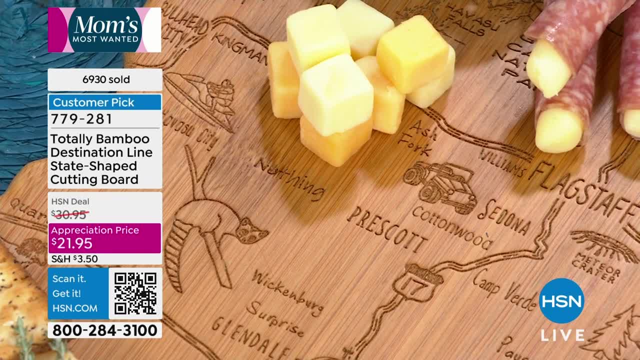 There's nothing Right below the cheese And I'm telling you it's a tiny little thing, It's a tiny little place in Arizona. So the fact that they put that on there is meant to be a little like trivia, a little fun fact about Arizona. 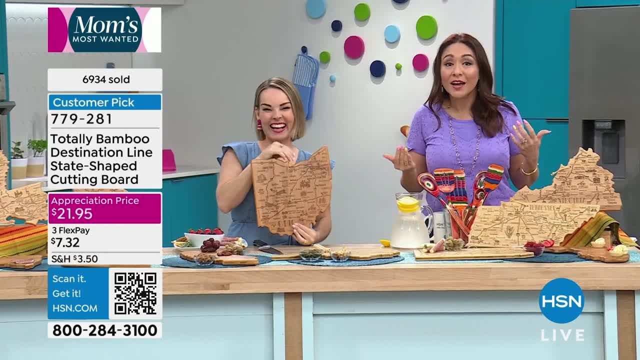 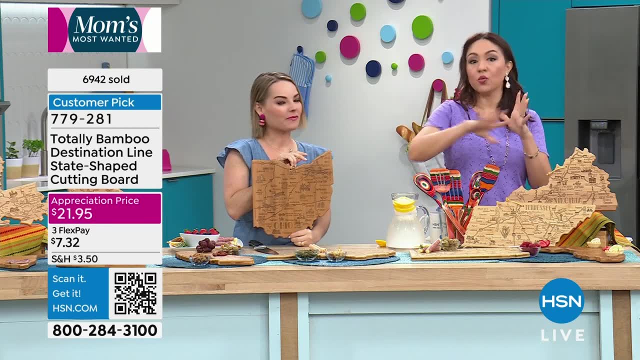 And people from Arizona would be like, yes, And I would tell you about Nothing. Arizona, These are so different And I'll tell you if you want to kind of do what I would do, or what Carrie does, is do all the places that are special to you. 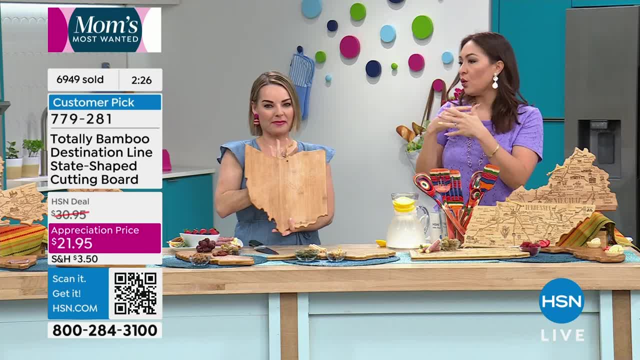 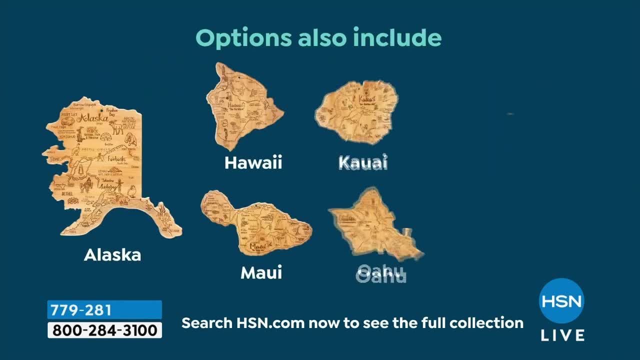 Maybe the place you honeymooned. If your grandmother, you know, speaks about a place or you know and is very heartfelt about it, this will give her like a shared memory. Yep, She'll think about it, She'll look at it. 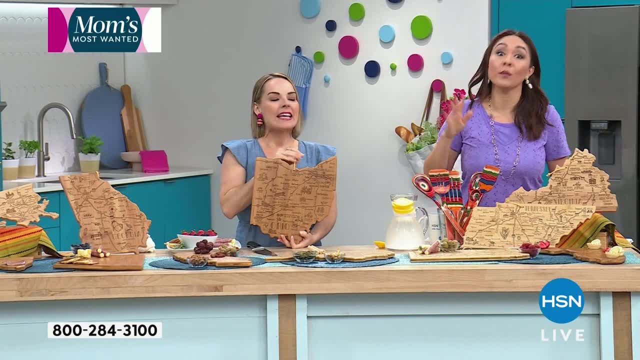 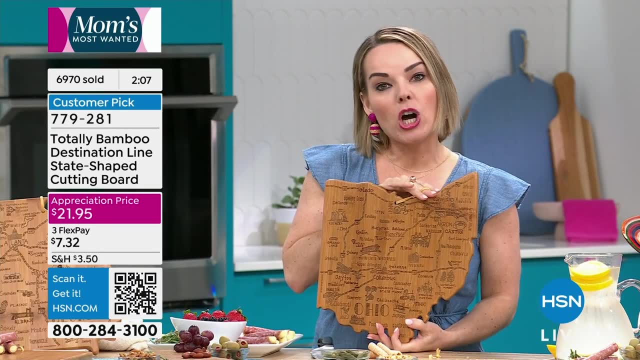 It's not just a cutting board. No, It's so much more, So much more. That's why it's gone crazy. That's why every time we have it, people just are buying it up. It's unique. If you were walking through like a craft show or something like that, and you saw all the states like up you, I was instantly drawn to these when they first came. 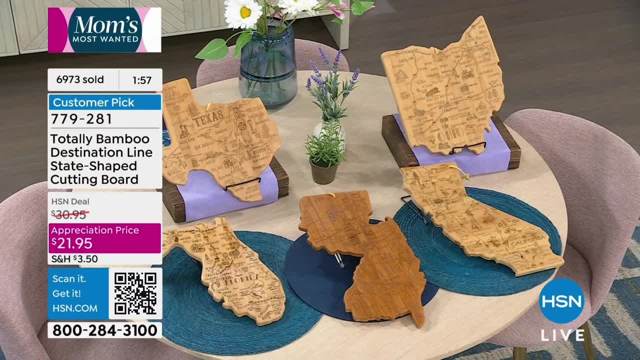 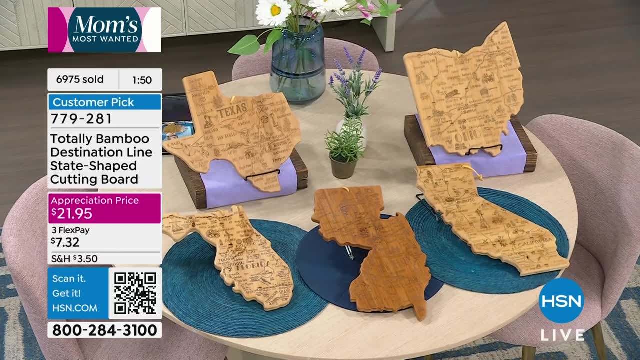 And I just went: oh, what is this? That's what happens when it's in your house. That's what happens when it's gifted to someone. They'll go. whoa, Because again, nothing like it. Super special. 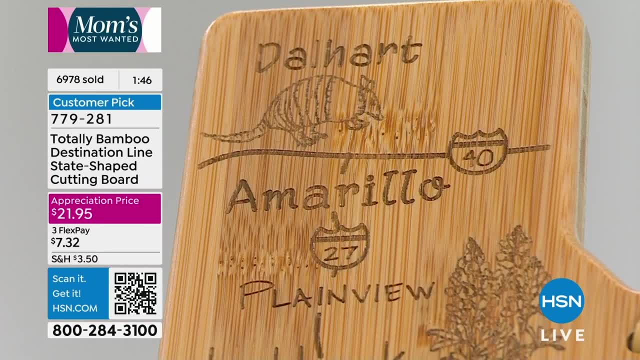 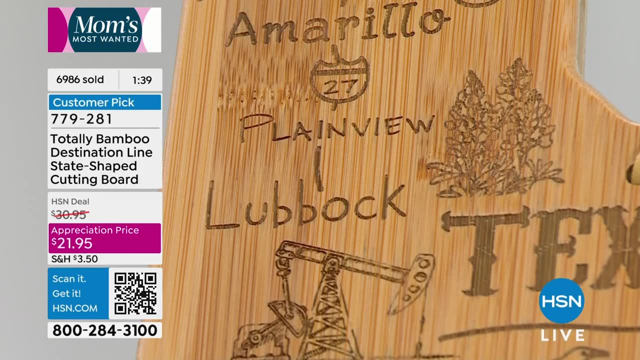 And that means you're going to be the ultimate gift giver, Because I love to always be the person that they're like. oh my gosh, I just love what you get me, And so I challenge myself all the time to find something really unique and really special and really different. 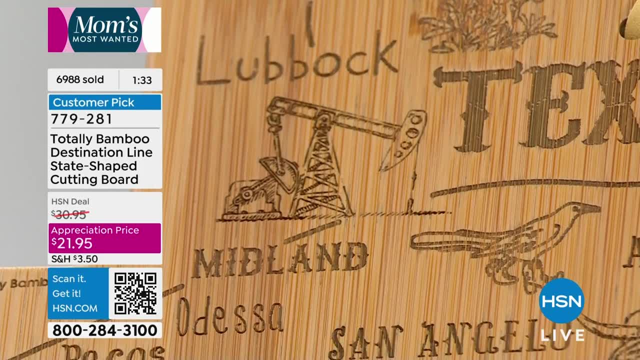 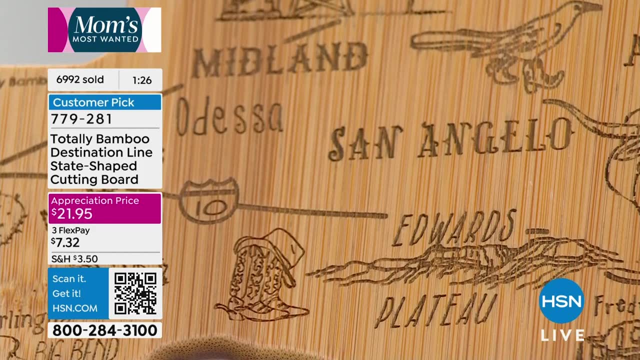 Listen, everyone loves their state, Everyone loves where they were born, usually or like where they called home. And so I think you were saying you had to like secretly ask your: was it a friend or family member that you were like? so what state do you call your home? 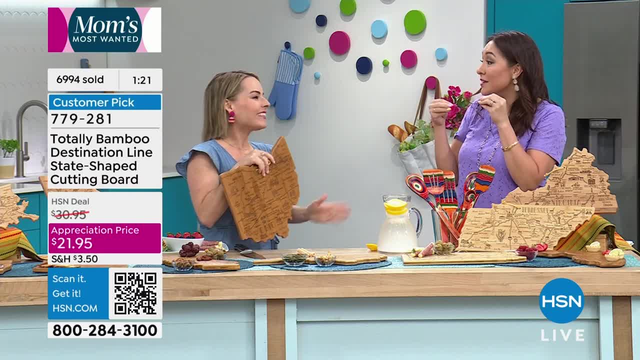 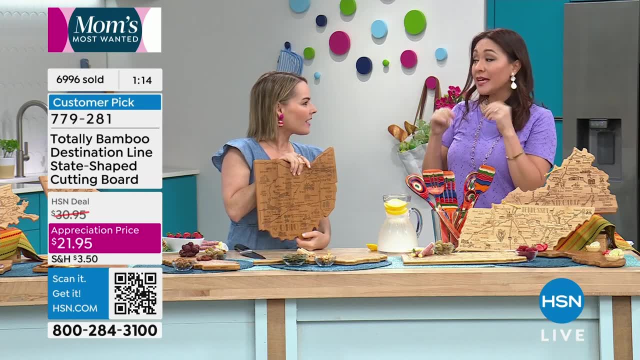 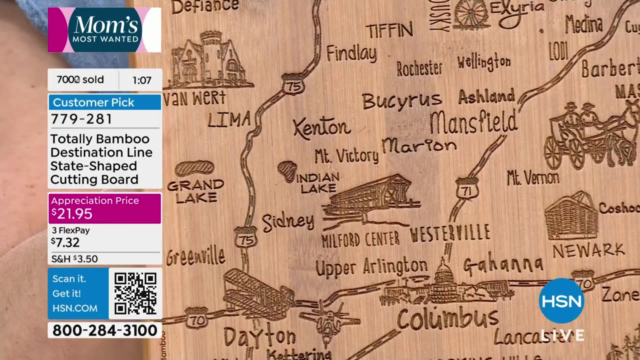 Yeah, yeah, yeah, Right, That's the only work you've got to do. And look, I feel like when you were saying like craft, Yeah, I think airport, You know, when you're in an airport and you go, where they have all the state things that you can kind of purchase right before you fly away. 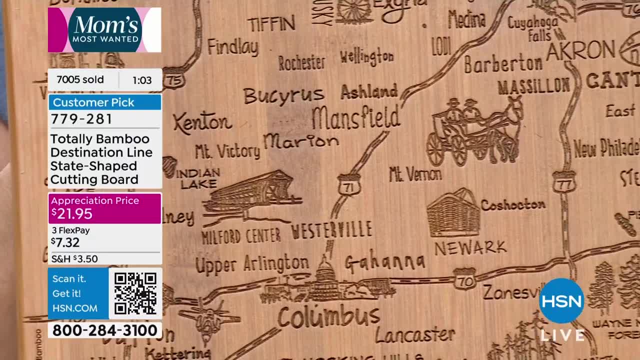 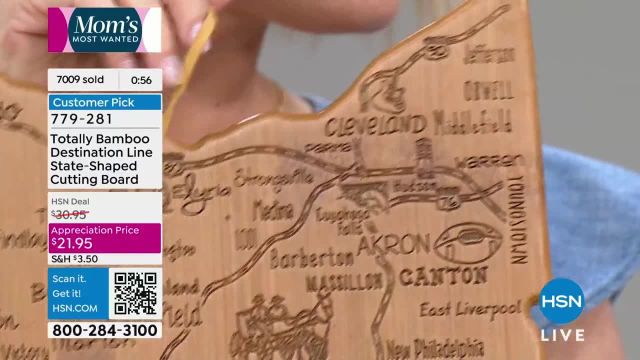 If I saw this board in the state that I'm leaving now, I want a memento from that state where I have had this great vacation or I've honeymooned or you know something. the airport would gouge me. This would be quadruple the price because they were now, it's state, identified. 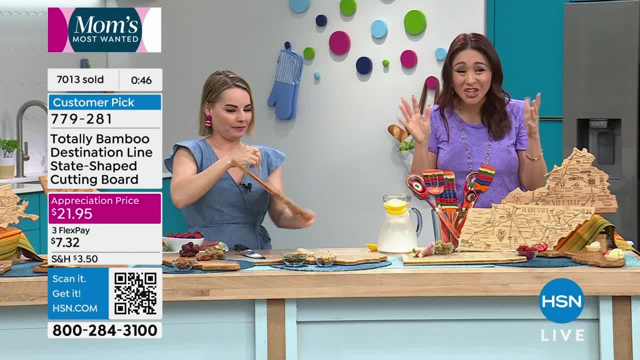 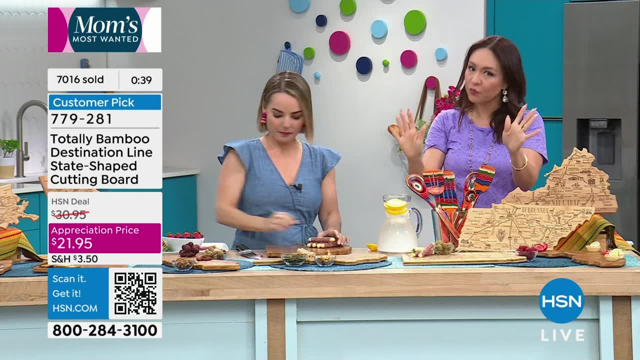 You know you want something as a memento- for $20, $21.95 to get this And it comes with a little leatherette. So if you want to hang it, which is what a lot of people do, is they display this? 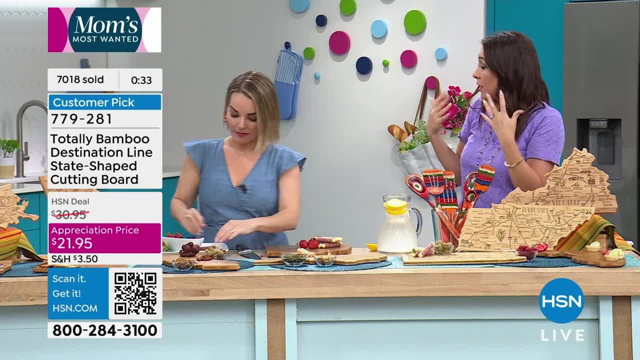 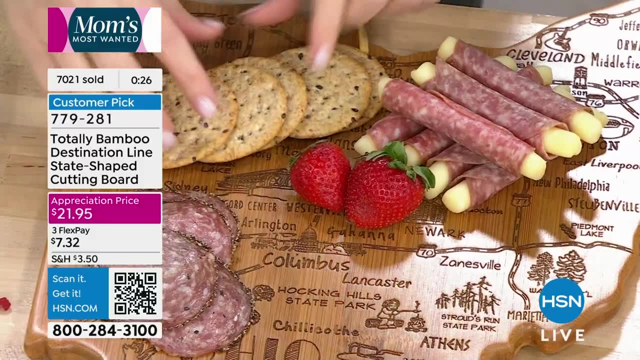 Some people may never even use it as a charcuterie or as a cutting board. They are just like I love it for decoration. $21 still worth every penny of it. But it comes in the state shape And it's not just your regular the capital. 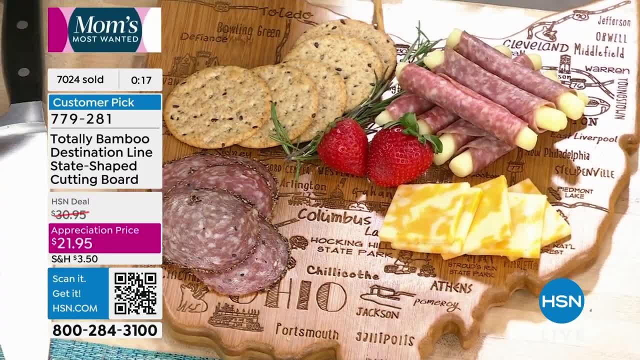 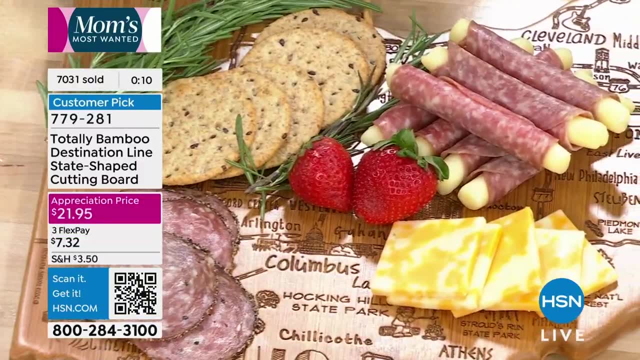 The other big city, Like they really made thoughtful pieces on every single one. They really did an exceptional job And that's why you guys are loving it. But if this is your first time seeing it, understand that Get one for yourself. 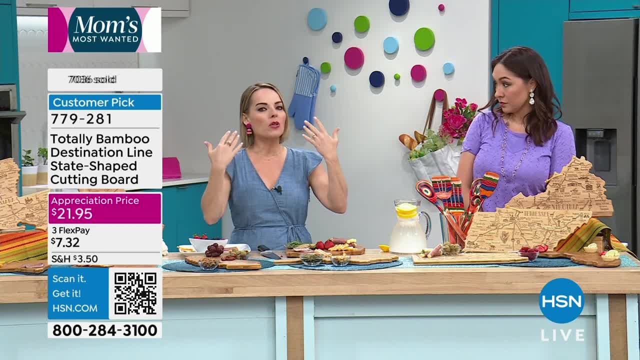 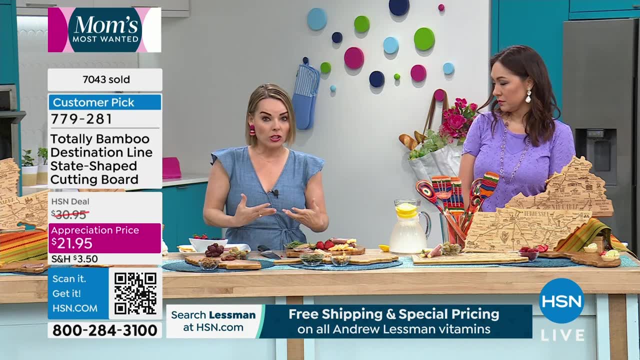 Get one for the state that means something to you. Then start thinking about all the you know events and activities and holidays and all that that are coming up. Get some of these in your gift closet. Be ready to use them for your gifts. 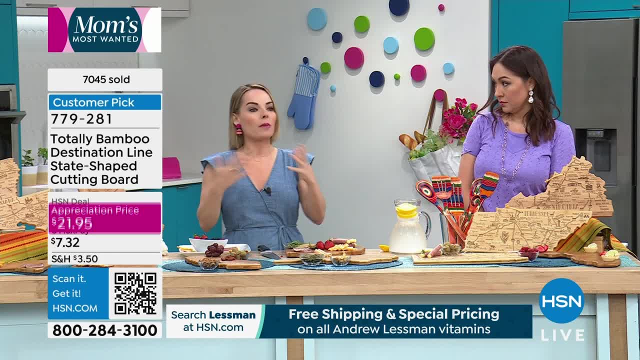 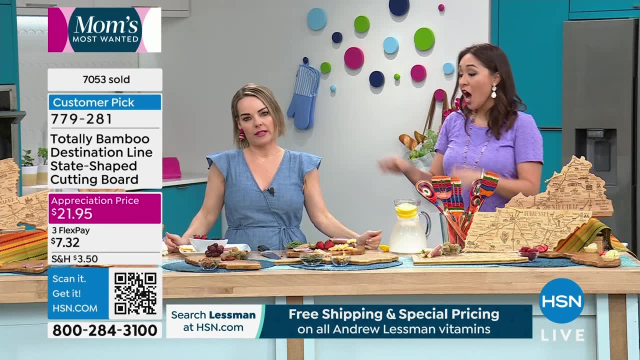 Again. perfect gift for someone going to college, Perfect gift for Mother's Day. Perfect gift for Father's Day: House warming, House warmings, Everything, All of it, All of it. Grab these. I will be back tomorrow at 7 am for another HSN Today.